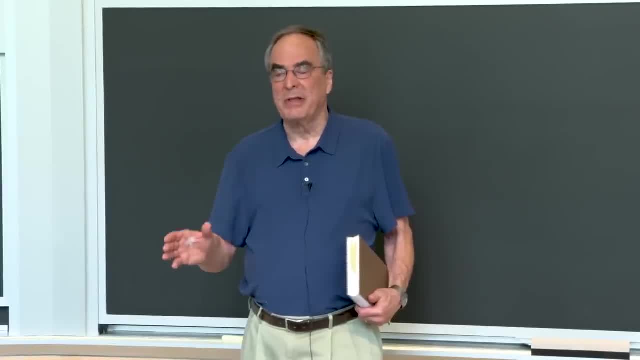 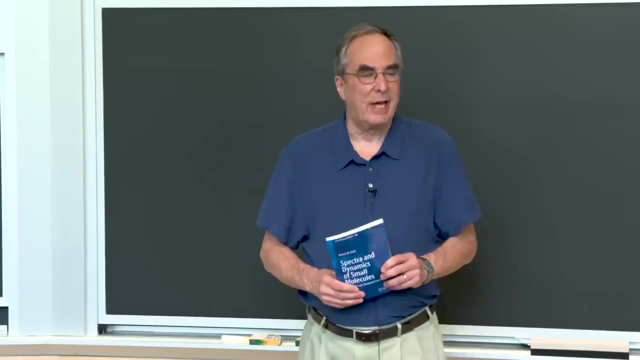 You're responsible for that. If I don't finish all the material in the notes, you're responsible for the material I didn't finish. You can ask me questions about it. You can ask your TAs questions about it, But there is a supplementary text, which is a book, that I 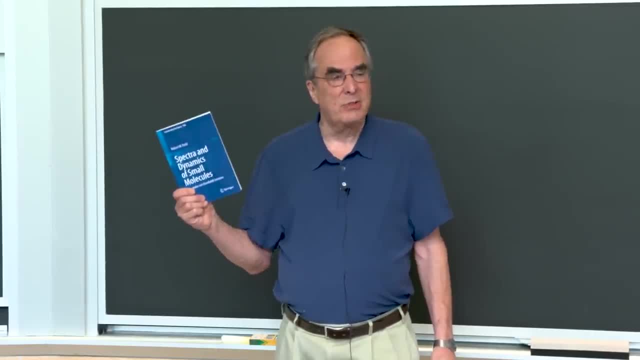 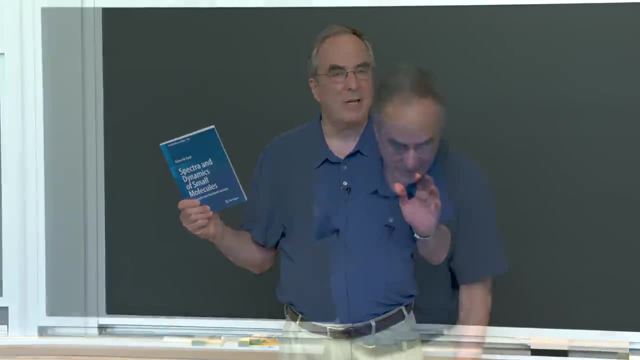 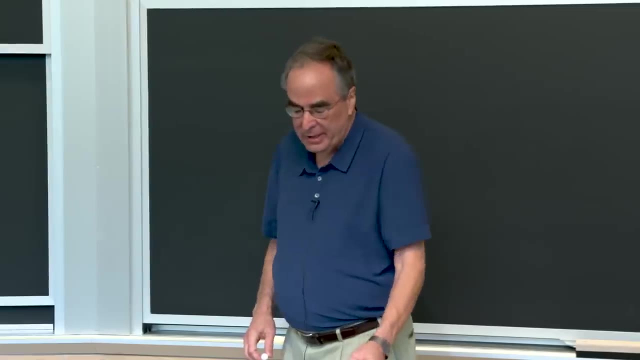 wrote And it is intended to take undergraduates like you to the frontier of research in spectroscopy. This is the book that I used to use to teach graduate quantum mechanics, So I've written a lot of stuff which is already available on the web. 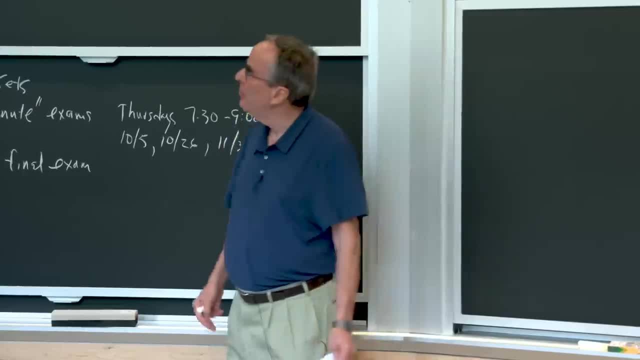 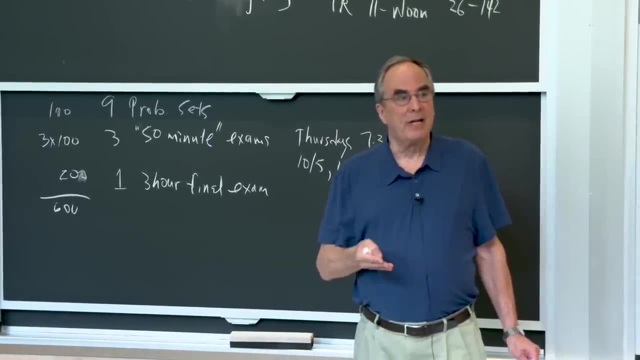 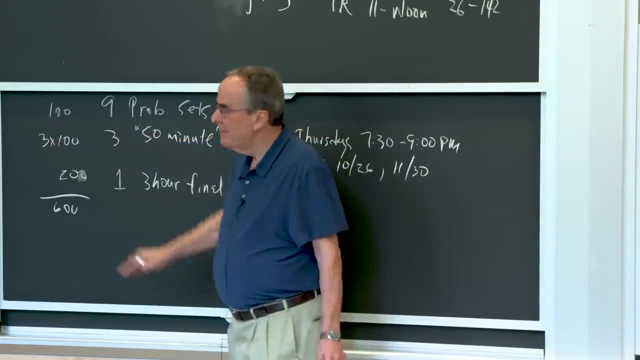 But I just want to make sure that you know the structure of the course. There are going to be nine problem sets, always in weeks. there is not an exam when there is not an exam And the problem sets are worth 100 points. 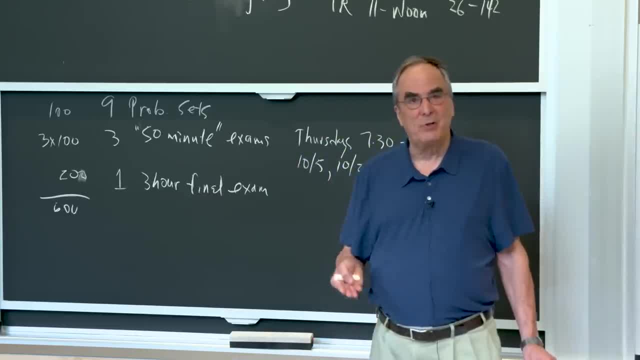 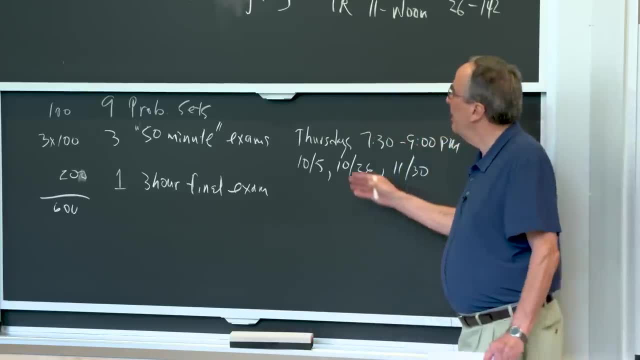 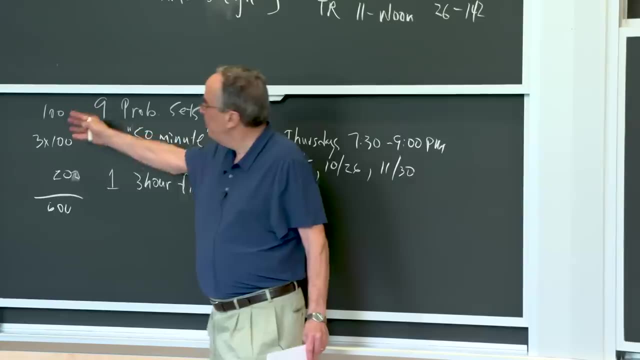 There will be three 50-minute exams, to which you will be allotted 90 minutes, And there'll be evening exams and on Thursday nights- OK- there will be a final during final exam period, And so the points for the course add up to 600. 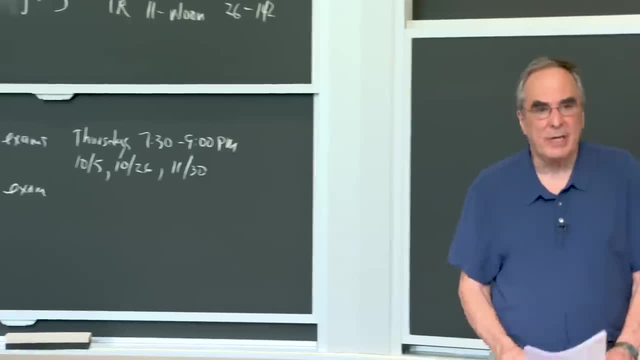 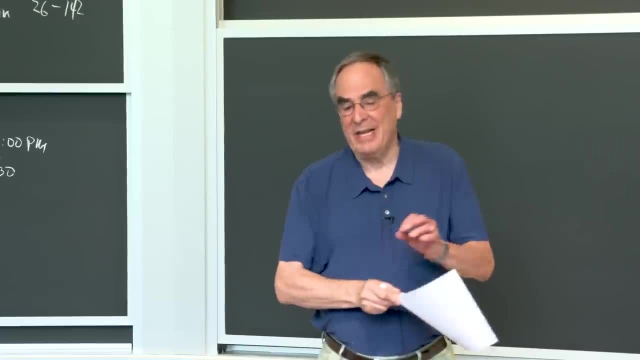 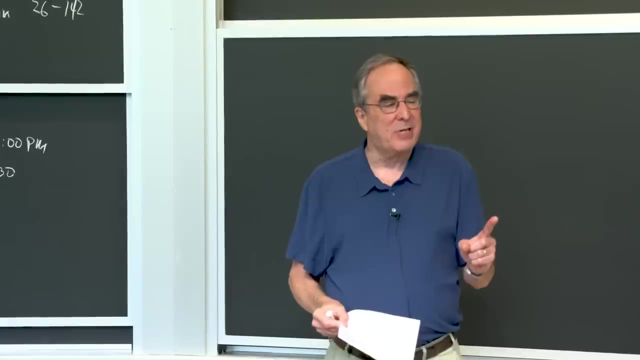 For each exam you will be entitled to bring one 8 and 1 half by 11 page that you prepared with as dense or as course writing, as you want. a different one page, only one page for each exam and for the final. 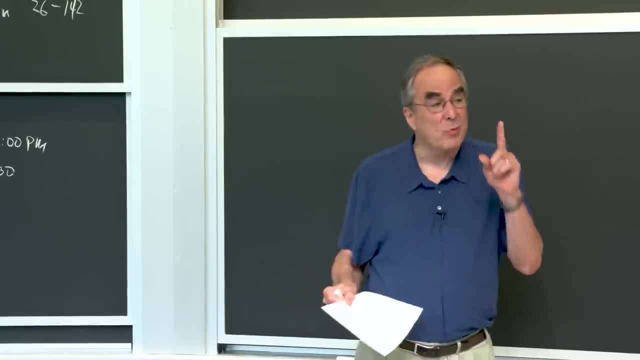 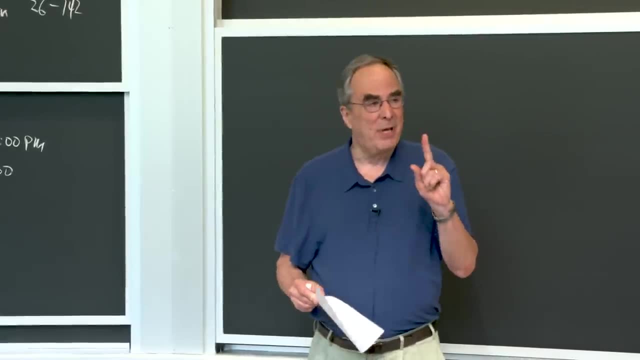 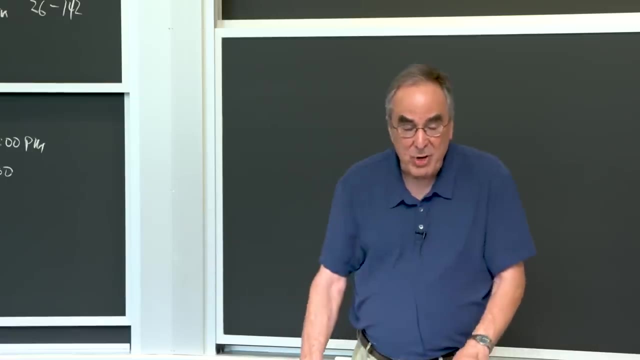 One page for the exam. one page for the exam, one page for the final, Not four pages for the final, not two pages for the second exam, et cetera. One page. I believe that writing these pages of notes or pages of things you should remember, 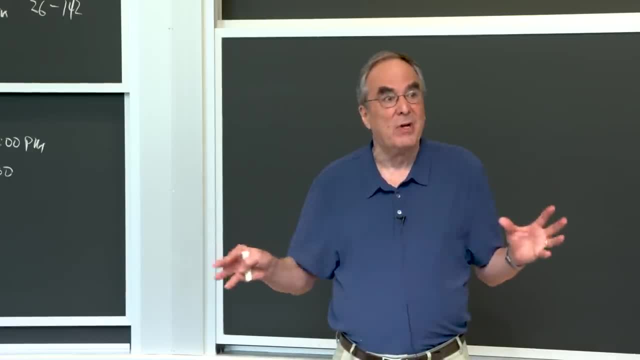 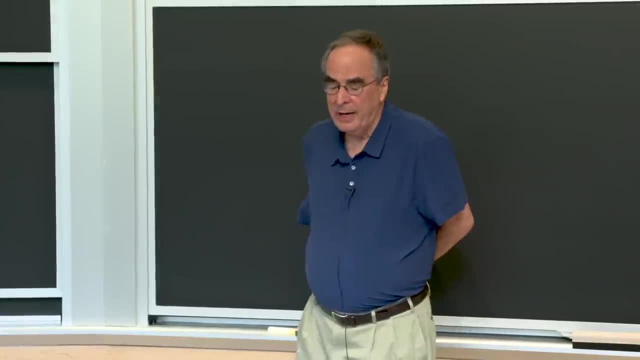 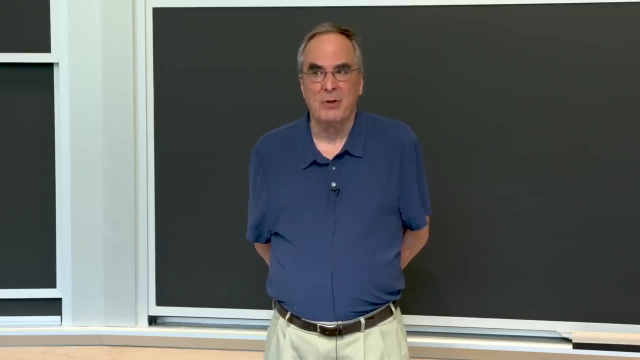 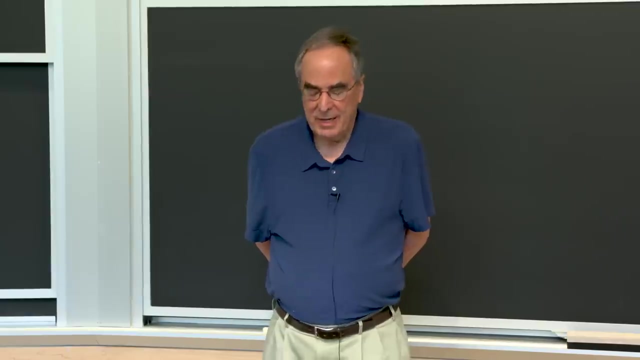 provide structure that you actually learn by preparing this, And so I stick to this. My job here is to force you to suspend what you expect about the way matter and light behave. You expect things based on your experience with macroscopic objects, And you're very smart. 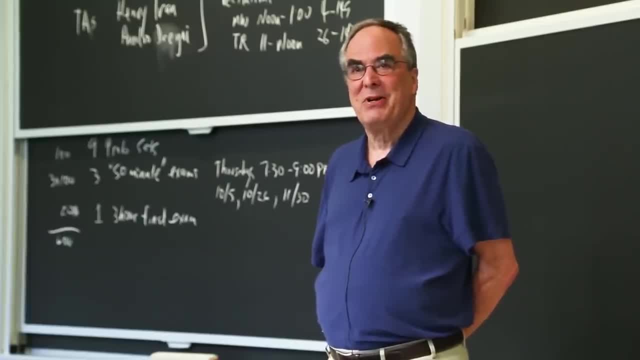 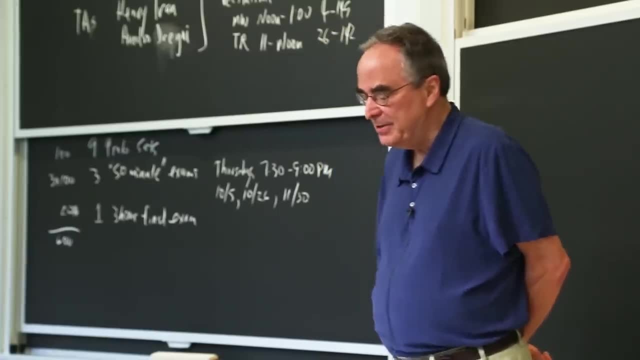 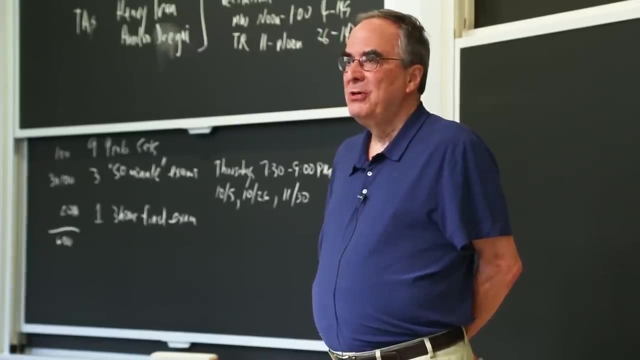 You're here at MIT because you are able to integrate that material, those expectations, and to express them in mathematical analysis of your observations. So you're pretty good at that. But quantum mechanics forces you. It forces you to step away from what you think you understand. 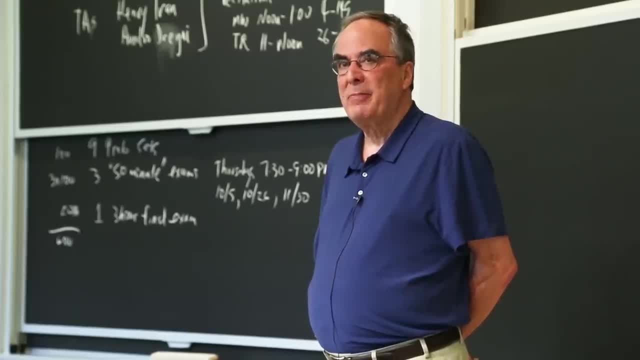 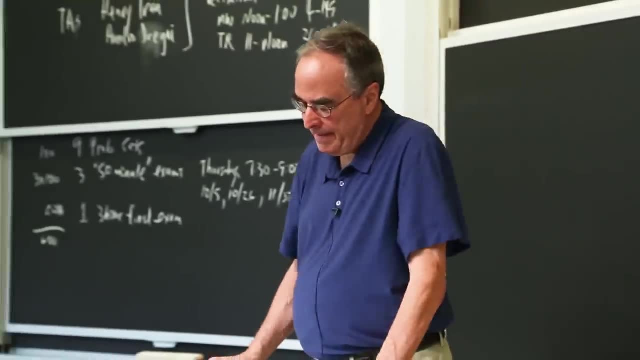 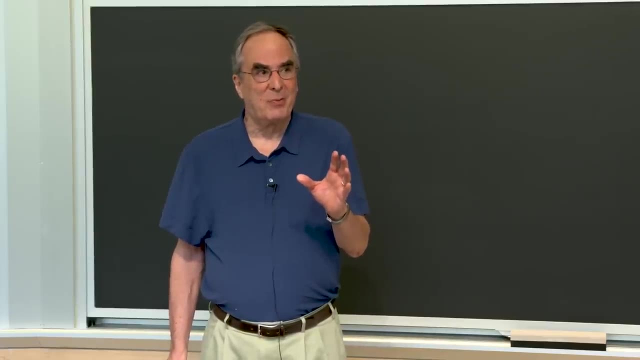 perfectly, because it doesn't apply to microscopic systems, And so I'm going to destroy your expectations about how things work at the beginning, And by the end, I will give them back to you in the form of- well, I don't know. 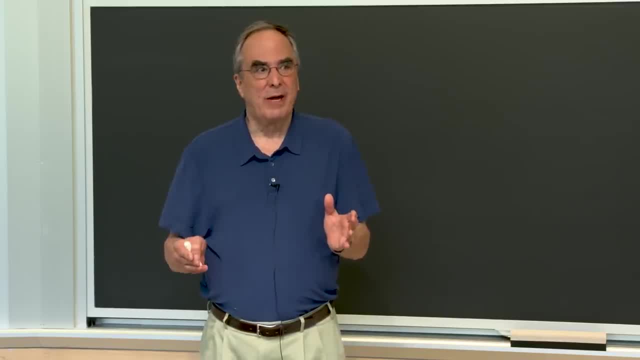 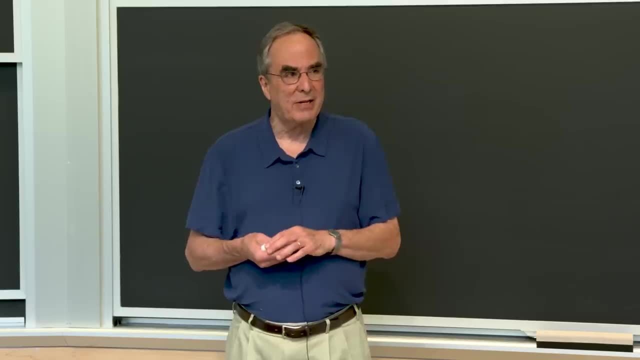 I don't know. I don't know what's going on. I don't know what's going on, And so I want to show you that it's a form of things called wave packets. Wave packets are quantum mechanical particle-like objects. They obey the rules. 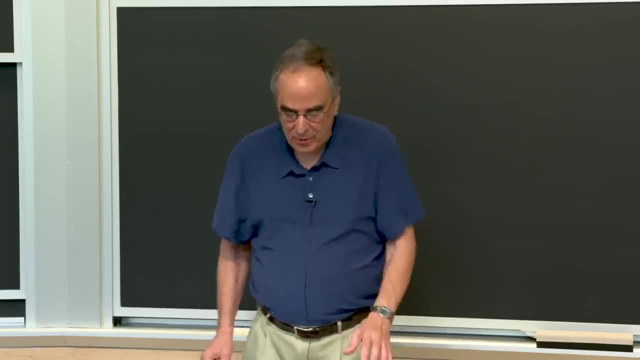 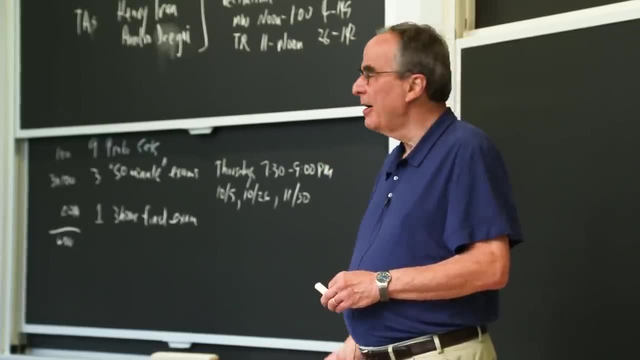 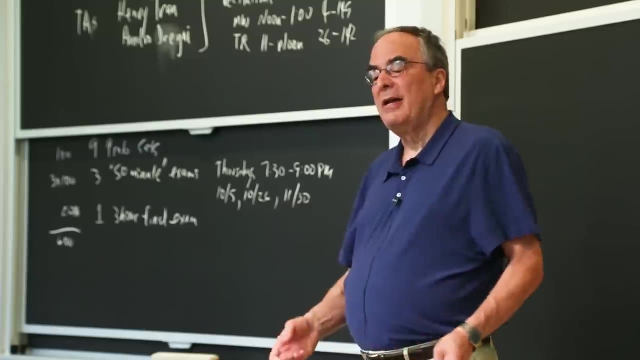 And they do a lot of the things you expect. But initially you have to suspend that belief in particles. OK, So I'm going to start by throwing a piece of chalk. I have to show it, And the chalk followed a trajectory. 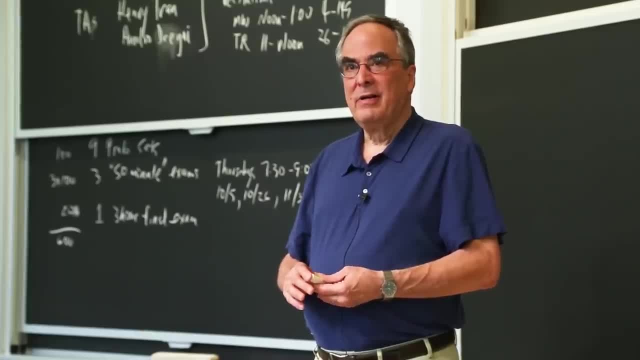 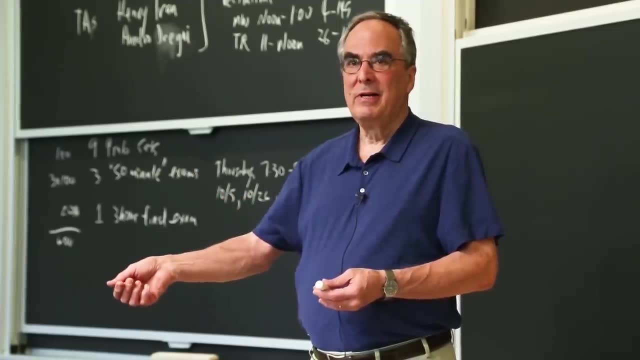 If you're a major league outfielder, you look at the initial part of a trajectory and you can pretty much figure out where you have to go. This sort of thing would be the subject of 801.. But the outfielders don't know physics. 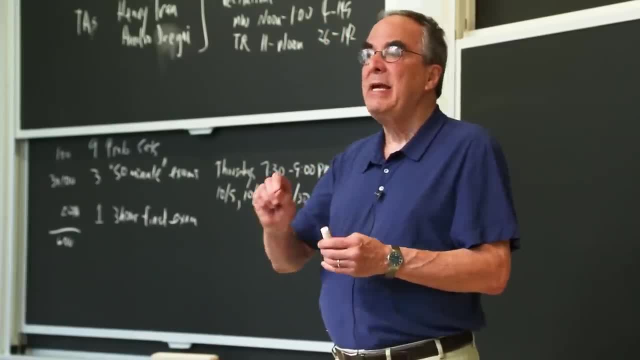 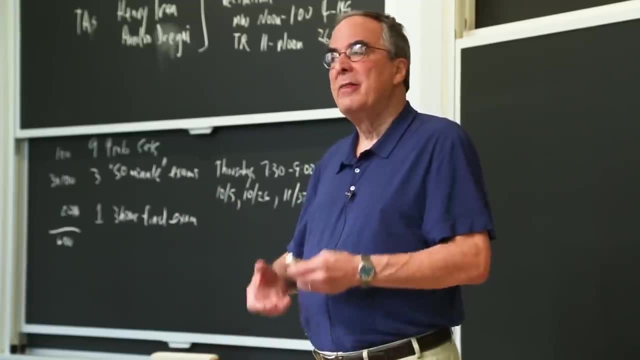 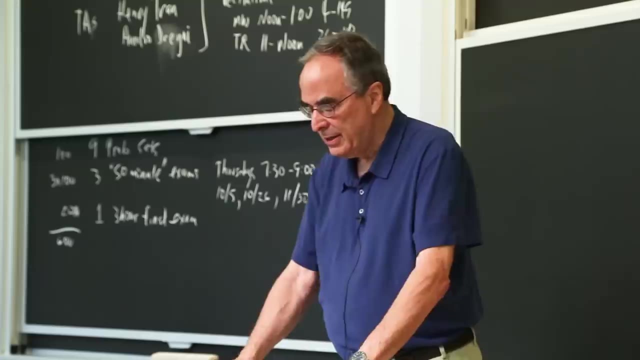 They just have instincts And they know that if they look at the beginning of a trajectory, they can predict where it will end and when it will end. And this is really important. That's the macroscopic view. We talk about trajectories. In quantum mechanics, there are no trajectories. 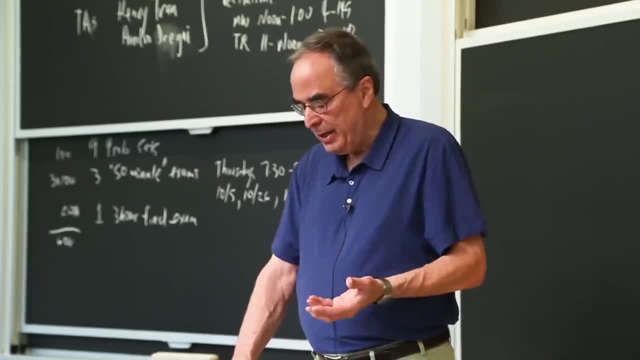 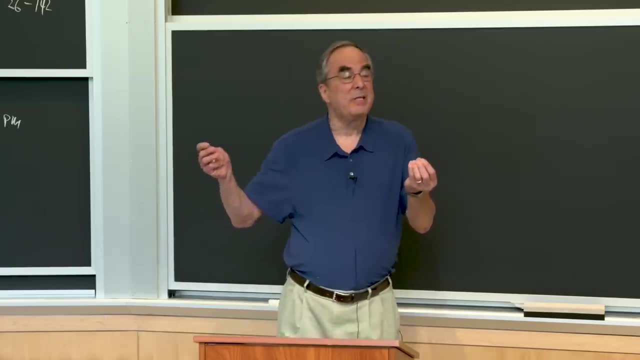 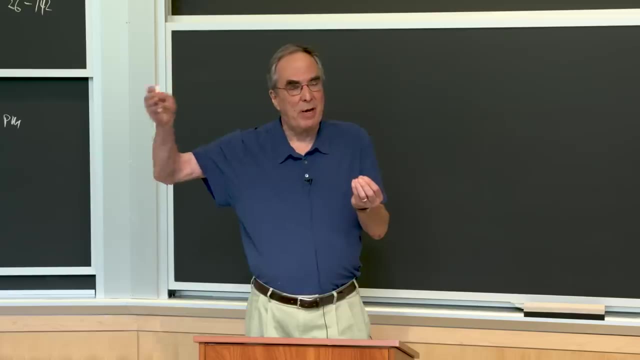 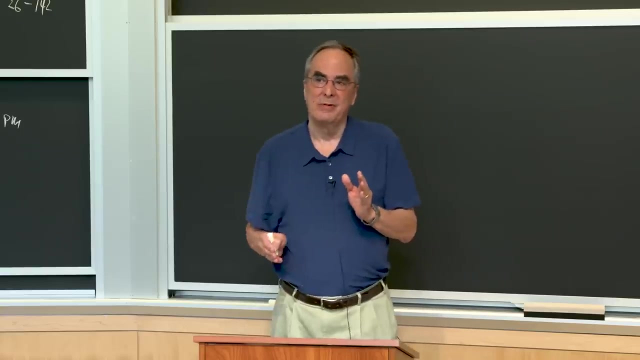 We have possibly an observation of what was the initial condition and what was the detection event, But we can't describe what's going on by observing. We can't describe what's happening point by point, the position and momentum. We're only allowed to do what we call click-click experiments. 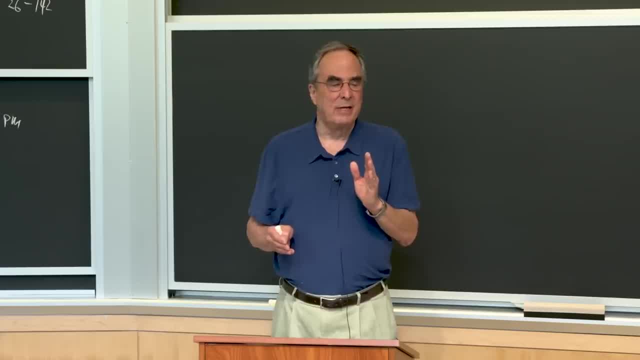 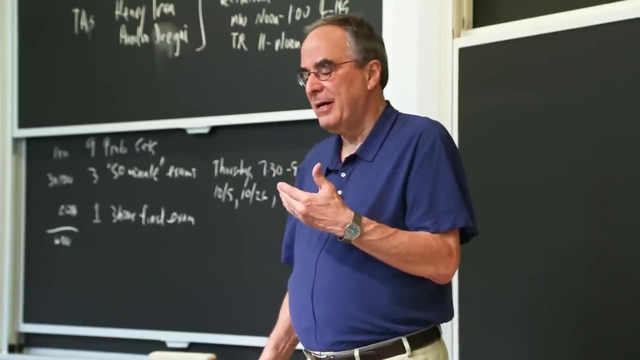 We start something in some kind of a well-prepared state And then we detect what has happened at the end. We might do something to the system in between, but we cannot observe everything as the system evolves, And here I will attempt to a little bit. 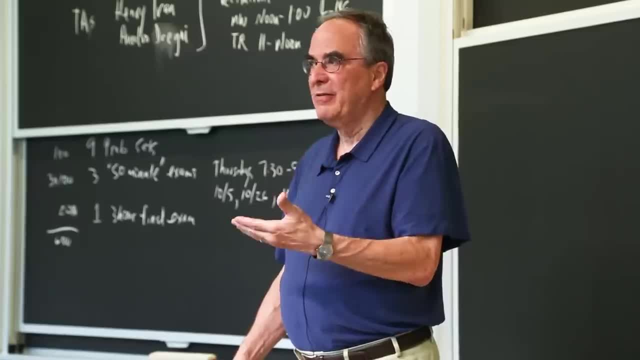 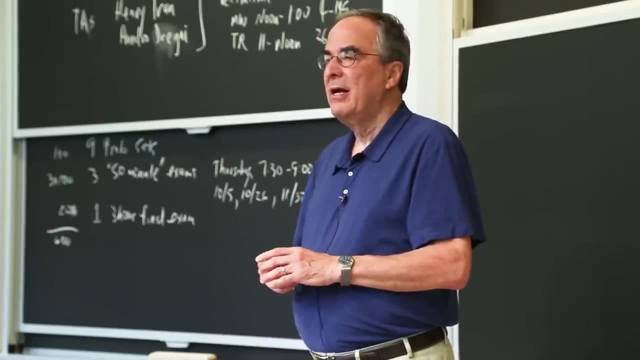 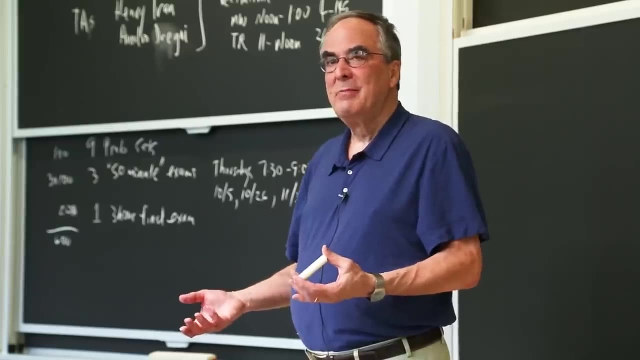 justify that you need to suspend what you believe. I threw a piece of chalk. It could have been a baseball. And suppose now I said let's decrease the mass of the thrower, the catcher and the object by 100.. You pretty much know exactly what will happen. 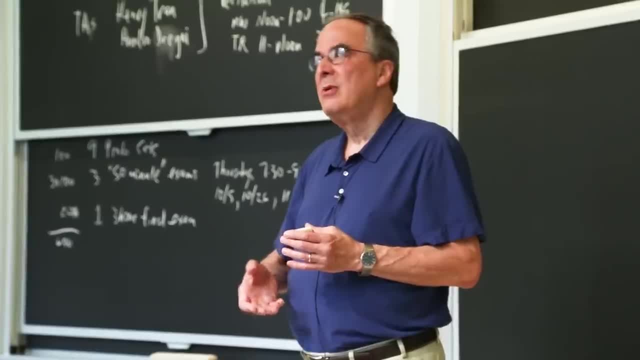 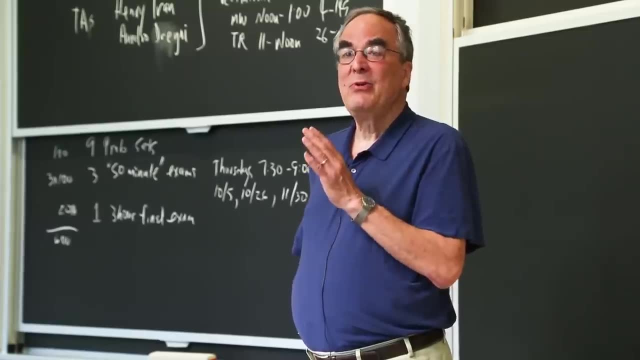 Now let's decrease the mass, Decrease it by a factor of 10 to the 20, which is like going from a baseball to an electron. You think you might know, but I guarantee you don't know And you're going to be surprised. 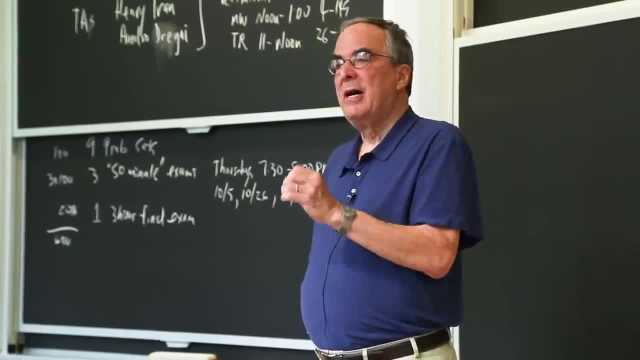 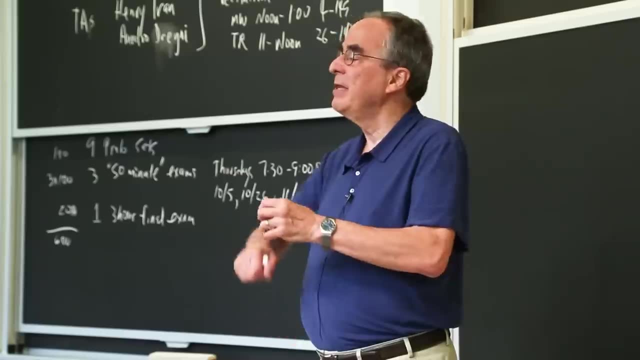 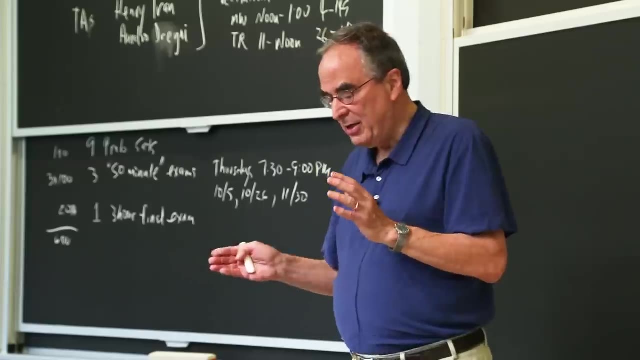 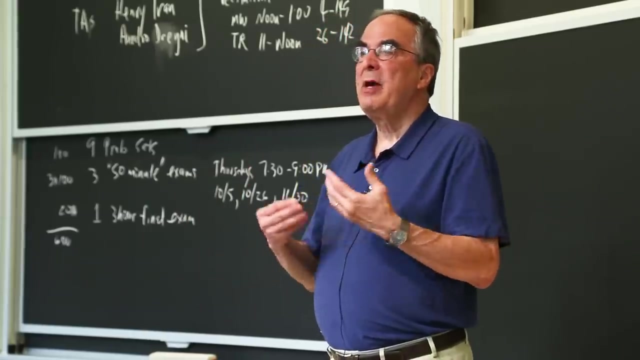 And it's because, in the microscopic world, observation modifies the state of the system, And any sort of interaction of the evolving system is going to affect what you observe, And so we have to create a formal structure which is a kind of measurement theory. 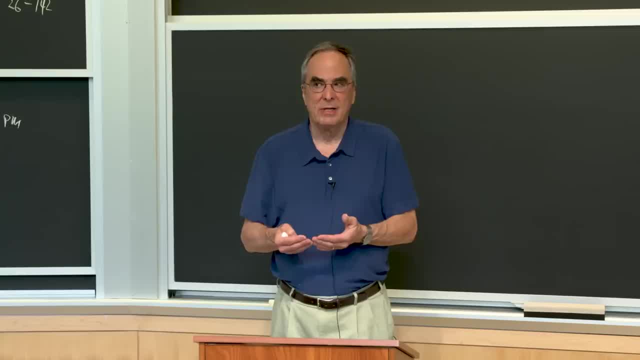 What measurements are we allowed to make and what do they tell us? Because you cannot observe the time dependence. You can calculate what the time dependence is if you know enough, but you cannot observe the thing evolving except by destroying it. OK, 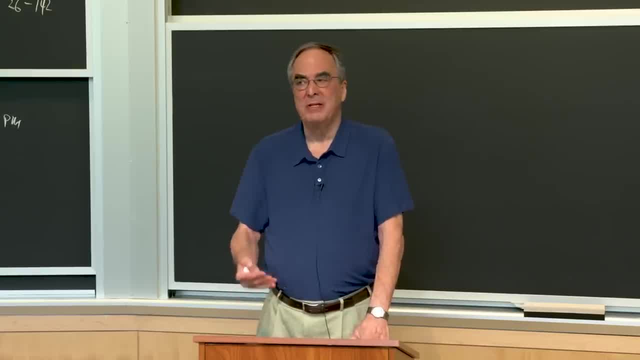 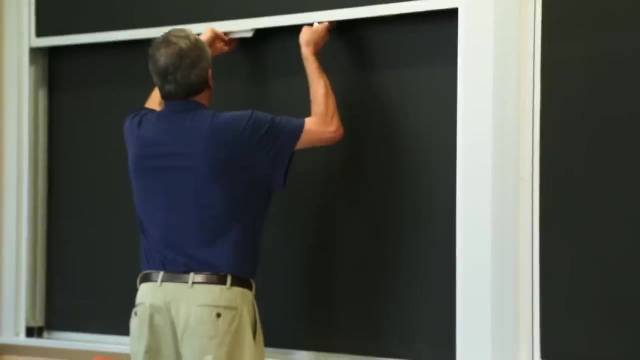 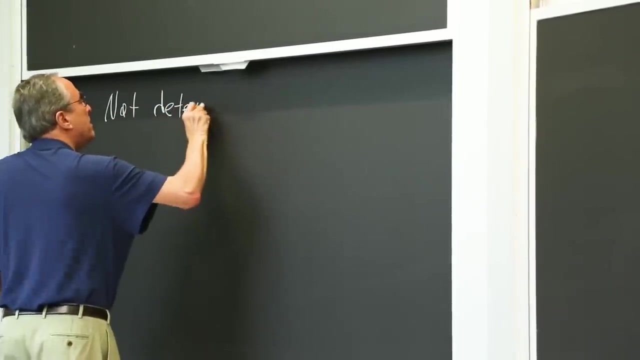 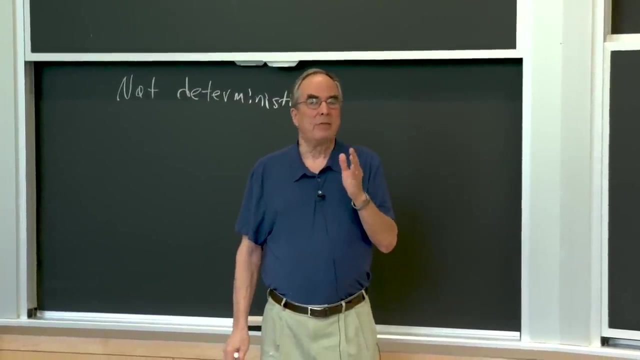 So quantum mechanics is beautiful because it describes the microscopic world And it doesn't tell you you're wrong about the macroscopic world. It matches everything the macroscopic world does- OK, Some of the key ideas of quantum mechanics. So you do a series of identical experiments. 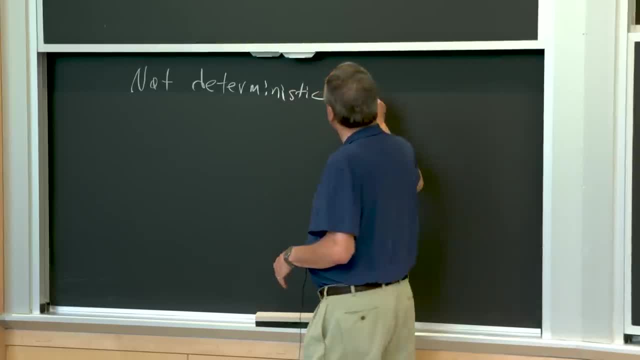 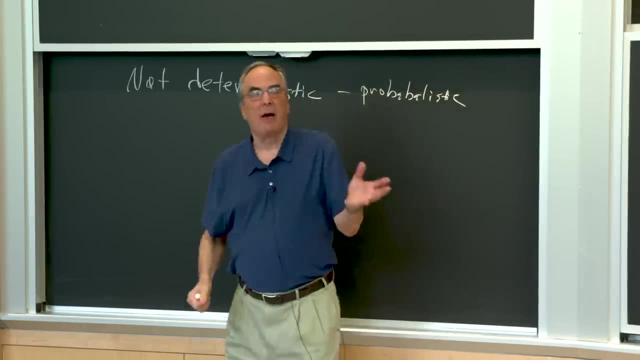 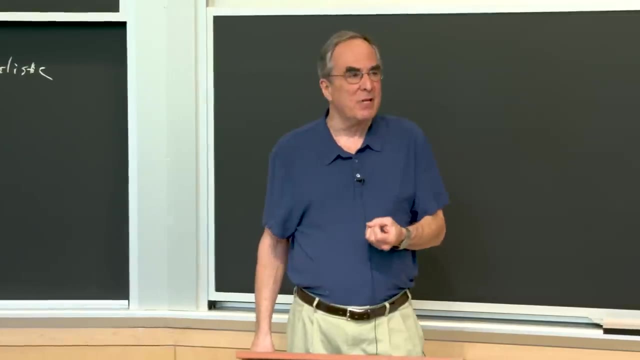 You don't get the same result. It's probabilistic And that should bother you, Because if you do an experiment carefully, you're trained to think that you do it carefully you'll get the same result. But quantum mechanics says tough luck. 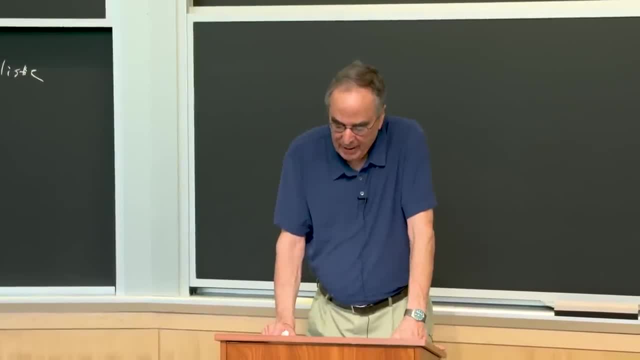 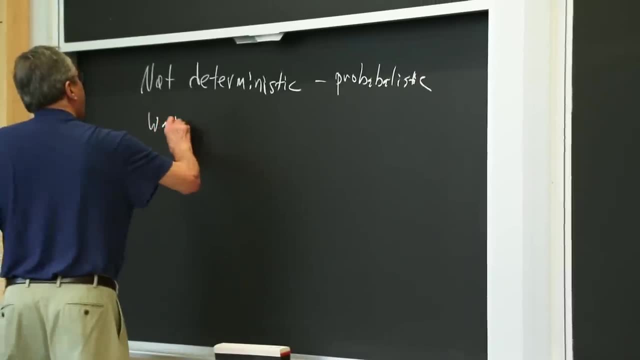 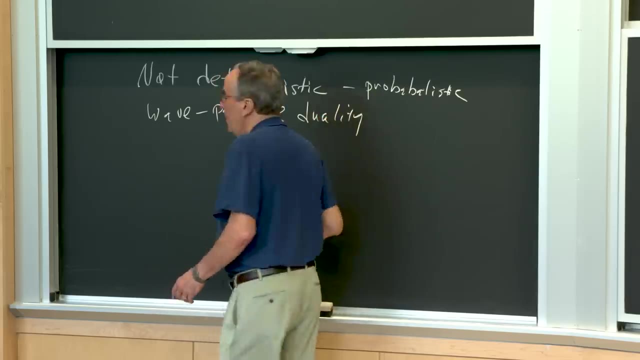 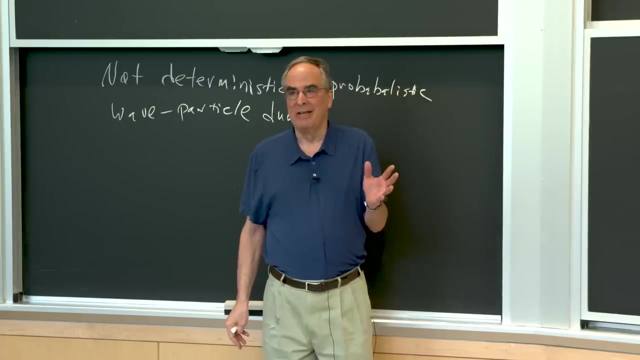 You can't do an experiment that carefully. There is also this wave-particle duality. You know what particles are and what the properties of particles are. You learned that in 8.01.. You know what waves are and you probably also. 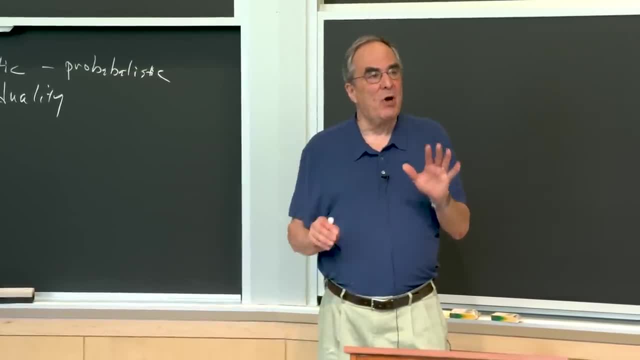 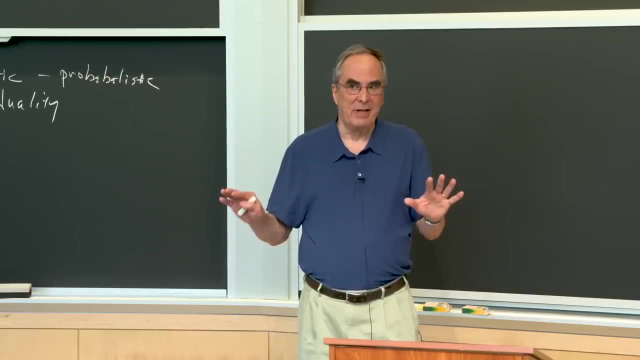 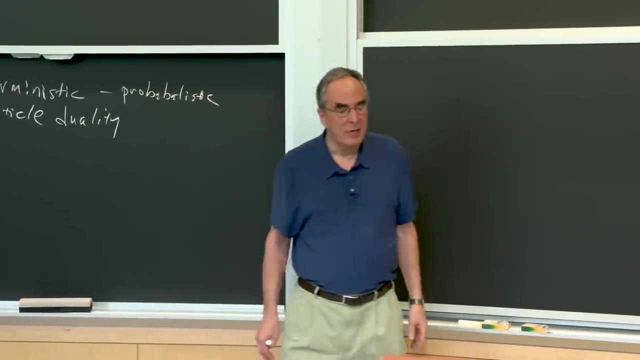 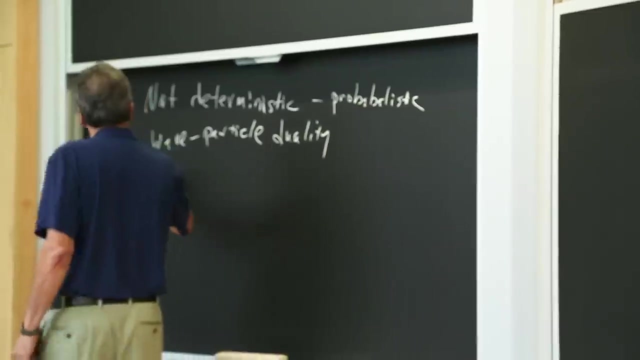 learned that in 8.01 or 8.02.. But you know instinctively that particles and waves behave differently. But in quantum mechanics everything is both particle-like and wave-like, And this is also something that should bother you. And the third thing is energy quantization. 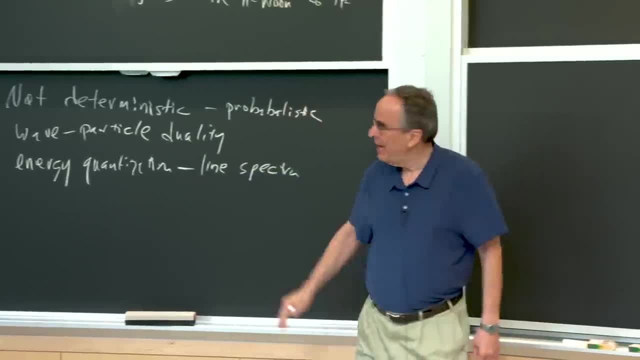 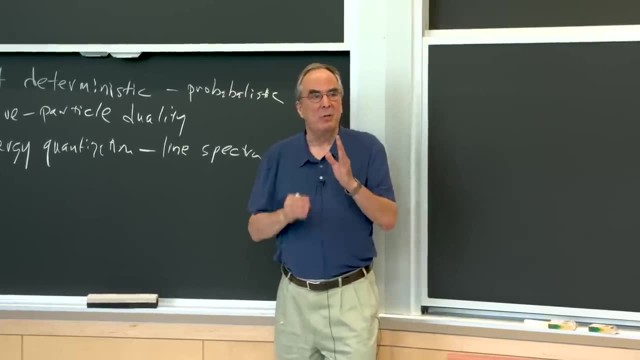 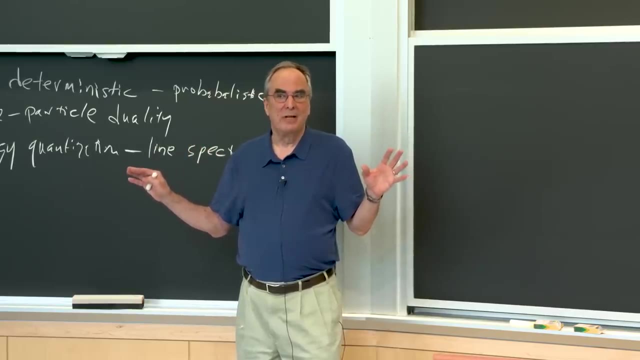 I said, I'm a spectroscopist, So I live and die by these spectra, which consists of transitions between energy levels. And these transitions, These transitions between energy levels, encode everything we want to know about the mechanics of an object, its structure. 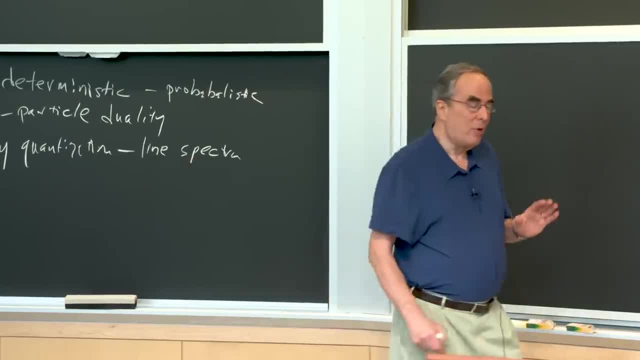 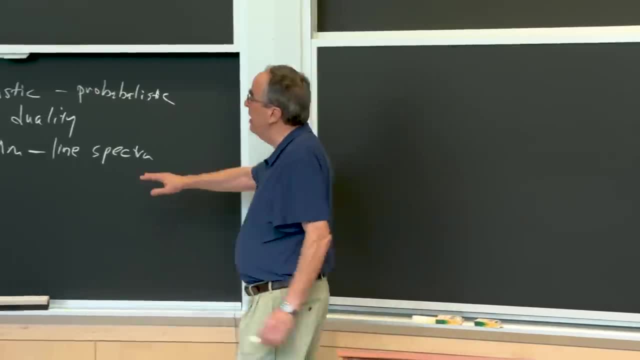 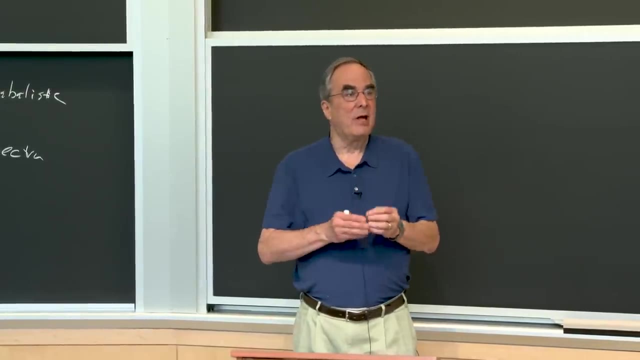 what it does, And so quantum mechanics is an elaborate encoder of information, And it's usually encoded in the form of these quantized energy levels, And so you're going to want to be able to calculate how the energy levels or the spectrum that you would observe. 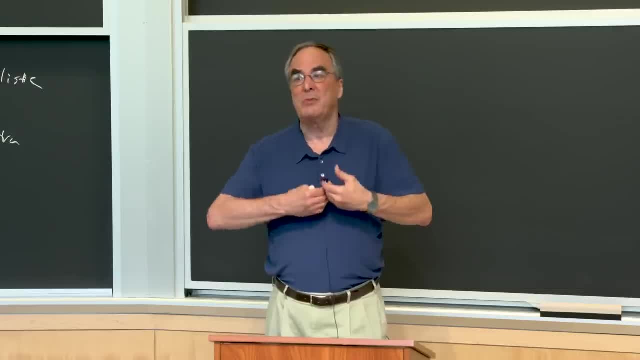 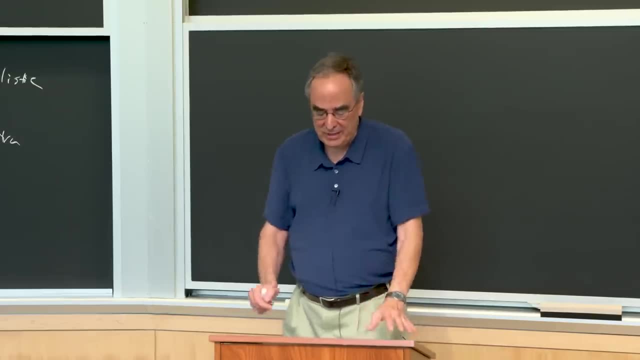 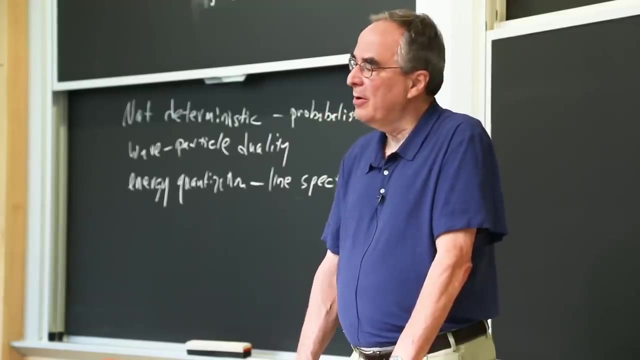 for an object is related to the thing that describes what it can do, And that's the Hamiltonian, And the Hamiltonian will look at in many useful ways. Now I just want to warn you that there are two ways of presenting quantum mechanics. 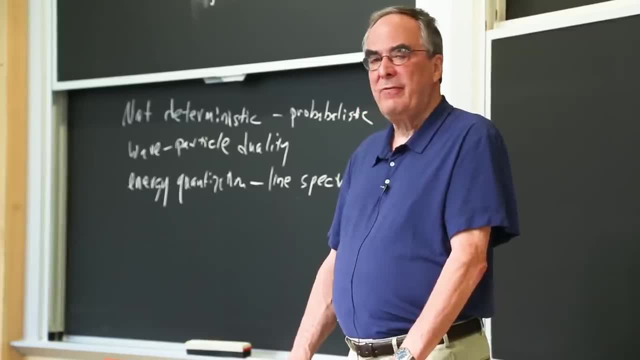 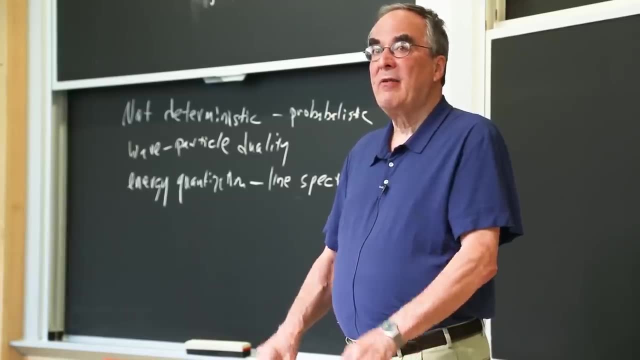 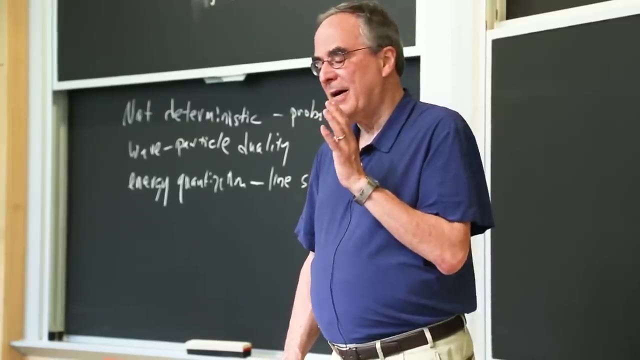 the Schrodinger picture, which is differential equations in wave functions, and the Heisenberg picture, which is matrix mechanics, Which is where we have matrices and we have eigenvectors, And I am an advocate. I'm passionate about the matrix picture. 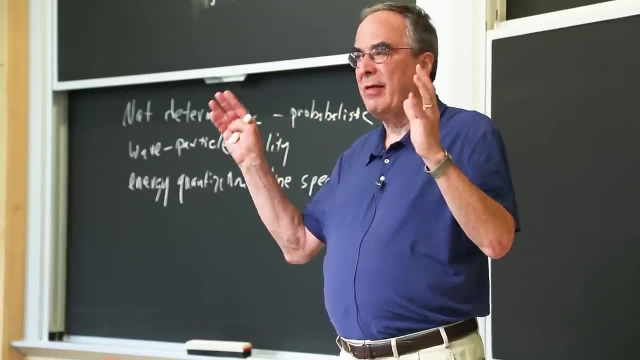 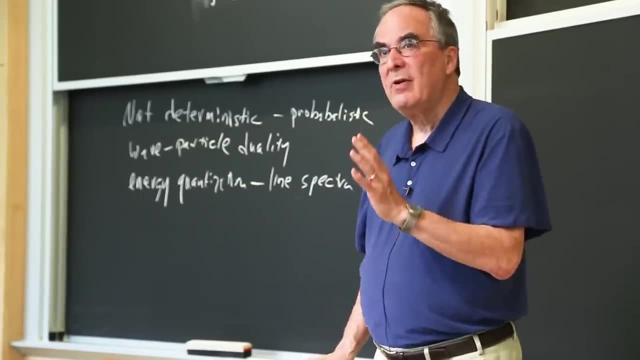 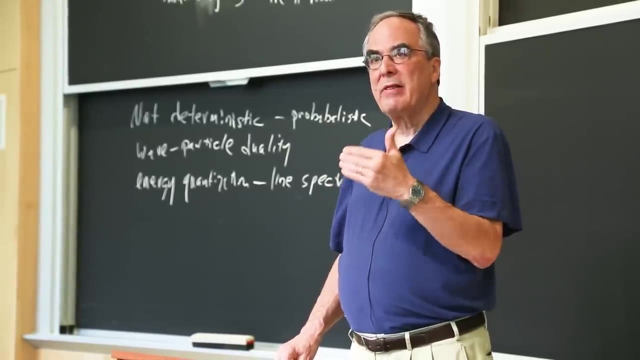 because what it does is presents everything in a way that you can then organize your insights, whereas the Schrodinger picture mostly involves solving one complicated differential equation after another, and the focus is on the mathematics and it's much harder to see the big picture. 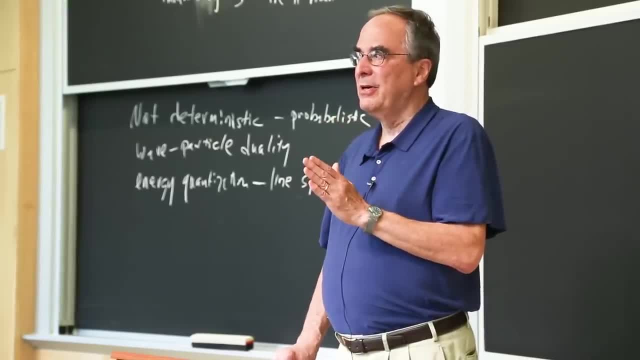 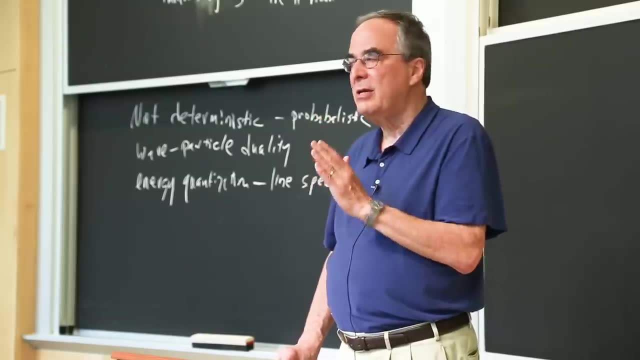 Now that means you need to know a little bit of linear algebra. Now, most of you haven't taken a course in linear algebra, but that doesn't matter, because the amount of linear algebra you need to know for quantum mechanics is extremely small. 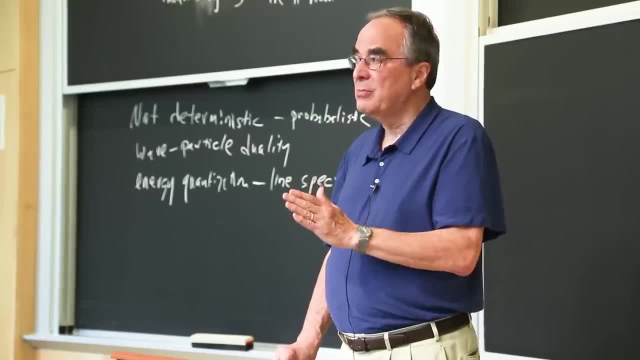 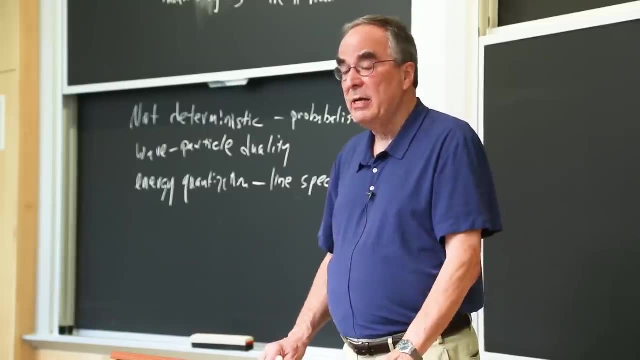 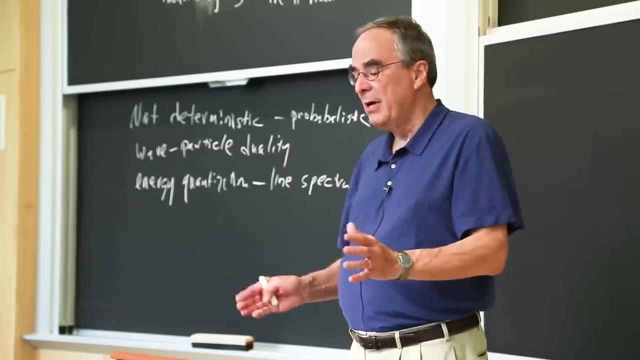 and I will probably present all of it in lectures. but you will definitely have the TAs as a a resource and it's possible that they will give some formal lectures on linear algebra or some handouts. but it's not complicated, It's beautiful. 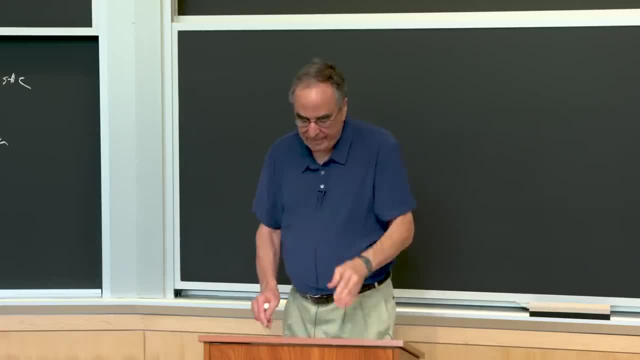 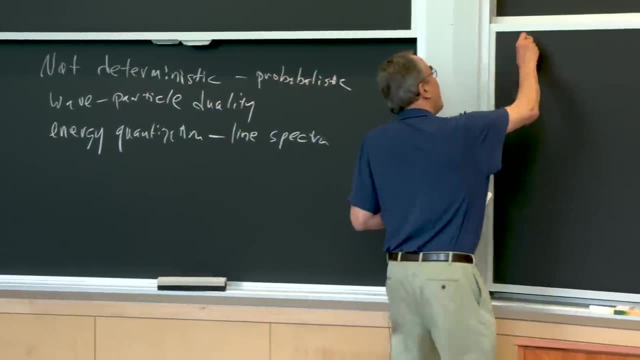 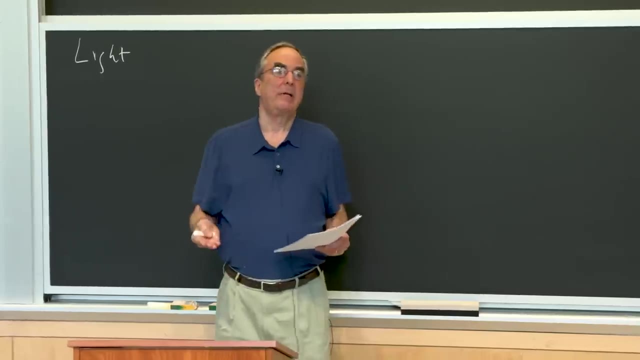 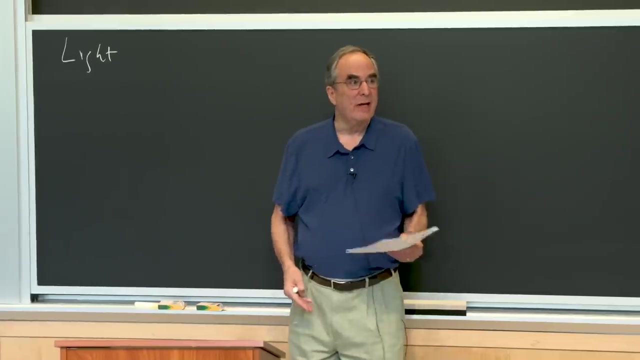 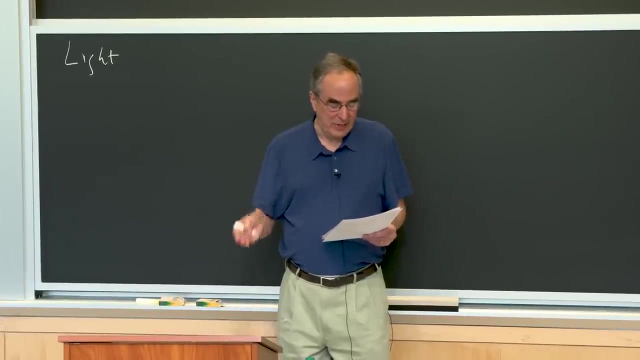 Okay, So Right over here Right Right Light is electromagnetic radiation. You've heard that- And it is both wave-like and particle-like. Now the particle-like aspect of light is going to bother you, but it's very easy to show that it's necessary. 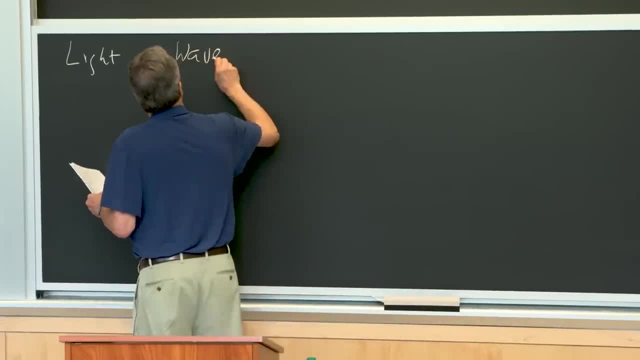 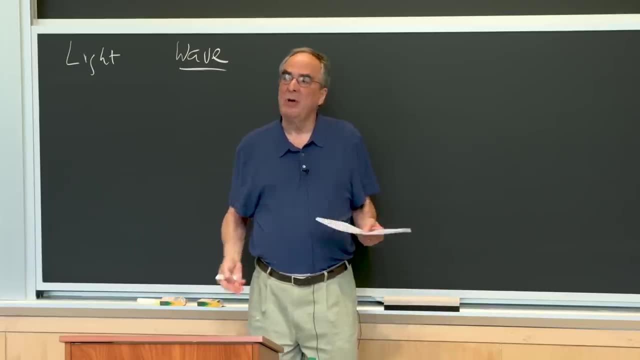 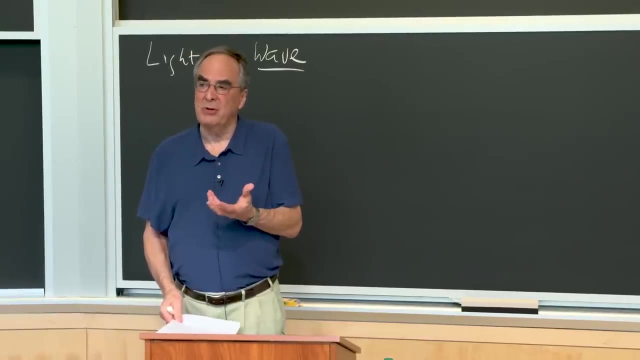 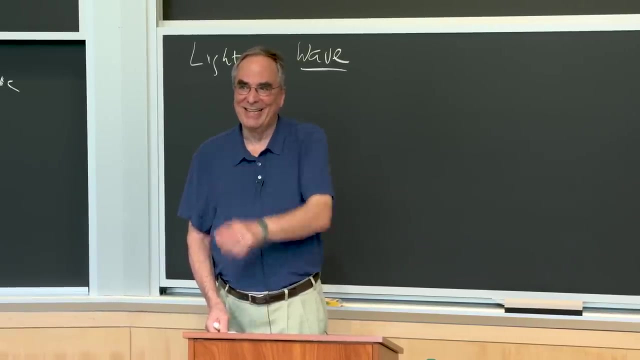 But okay. so first of all, what are some wave characteristics? What, If you have a wave? what do you? What kind of measurements are you going to make on it? Okay, Sasha, Intensity at a point in space. 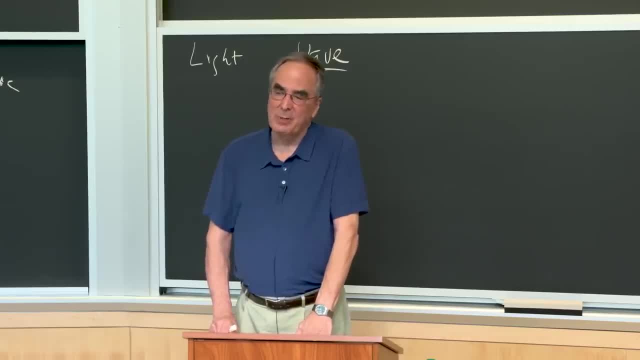 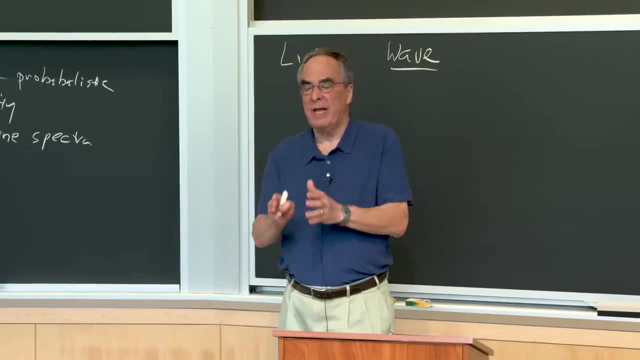 You can. There can be an intensity at a point in space, but there could also be particles that are impinging on that point, So you need something a little bit more that is definitely wave-like, And you have. Yes, It has a frequency and a rate. 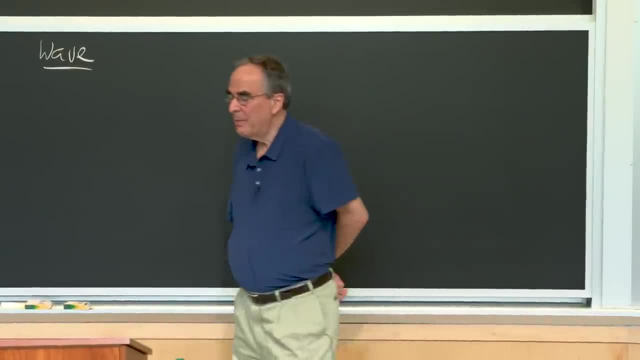 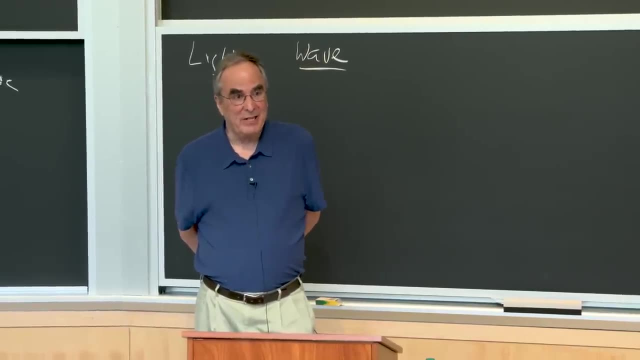 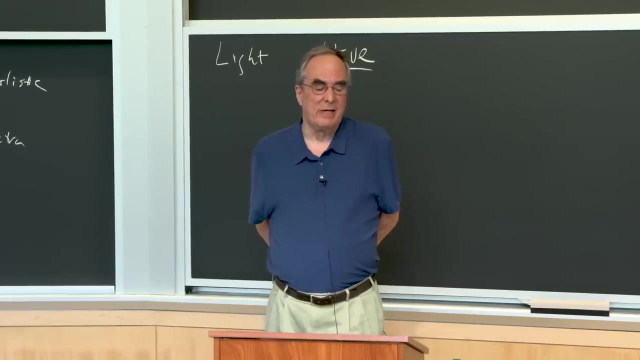 So it's a frequency and a wavelength and an amplitude. Yes, I'm angling for something more, I'm, But it does have a frequency and a wavelength, And wavelengths are how you understand interference effects. There are interference effects, And there You know, when you put light through a lens. 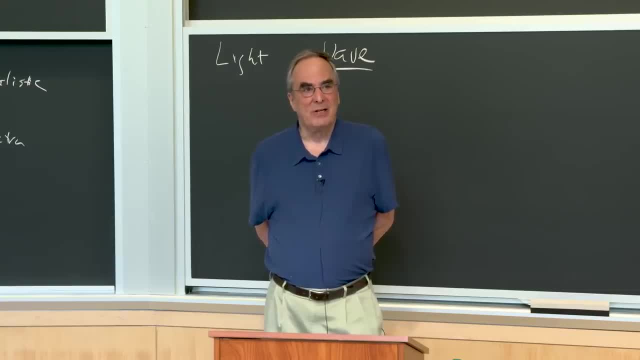 there's refraction. When you put light on a grating, there's diffraction- or through a pinhole. And there's the two-slit experiment, where you send light on an object which has two slits And you can't tell which slit the light went through. 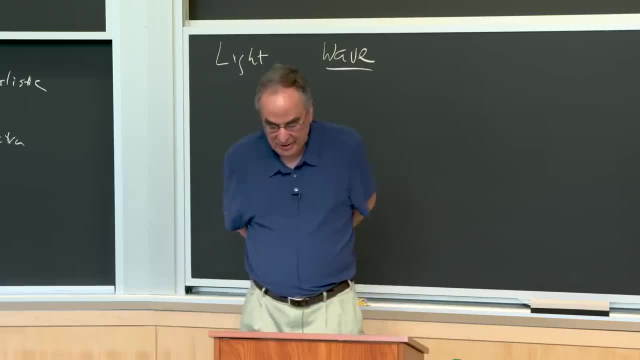 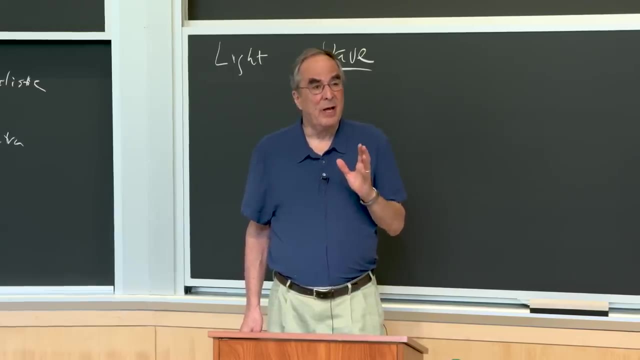 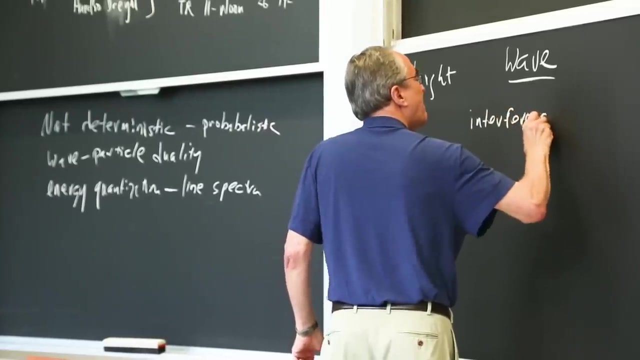 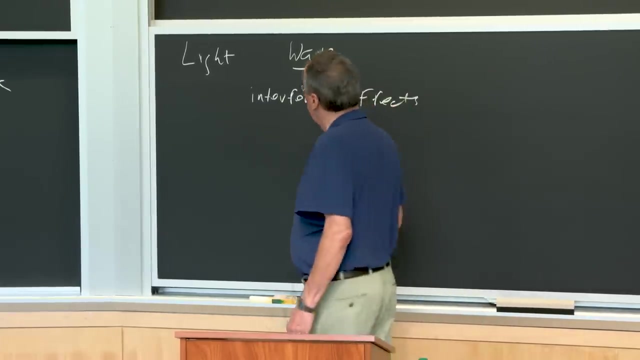 And this is a very beautiful thing which I will talk about in a coming lecture, In fact lecture number three. So the key properties of waves are refraction, diffraction, two-slit experiment, And behind that is interference effects, So we can have just a sort of a comic book picture or a cartoon. 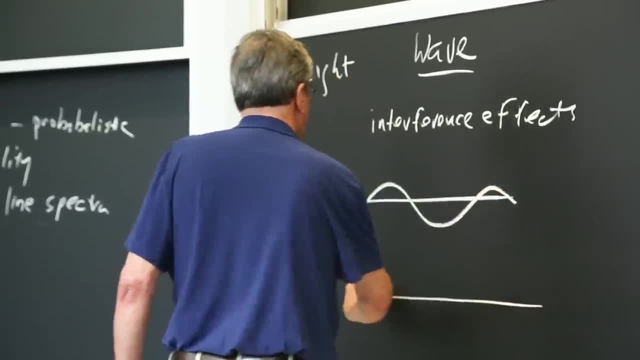 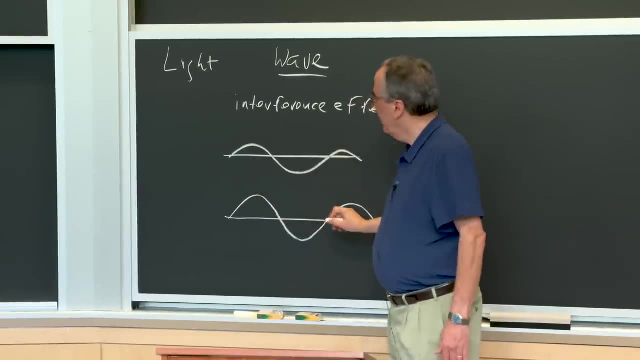 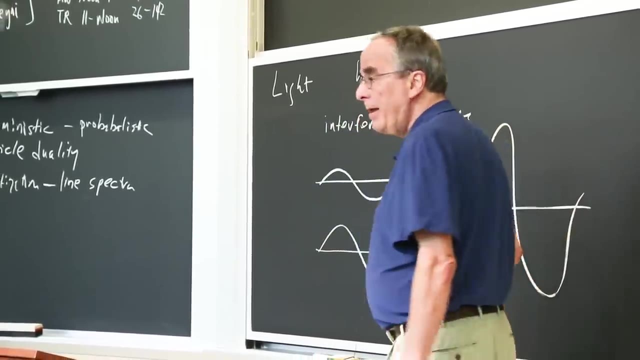 So here is a wave And here is a wave, And here is a wave, And here is another wave, And this other wave has exactly the same frequency and phase, And if we add these two guys together we get something that looks like that: 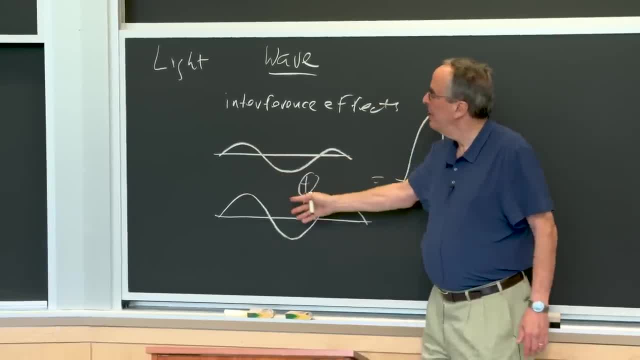 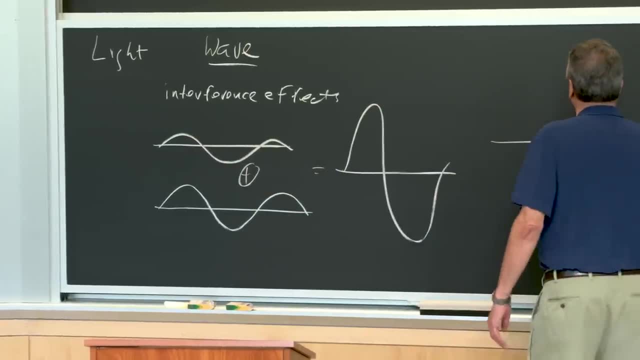 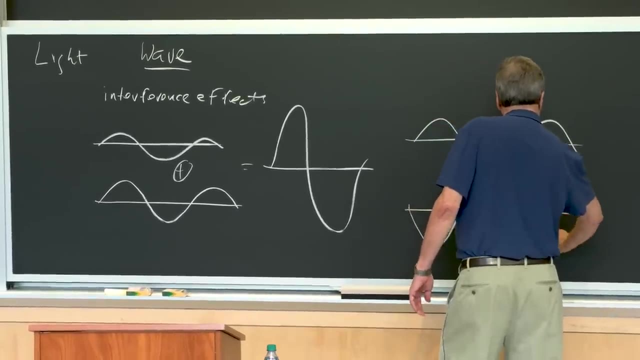 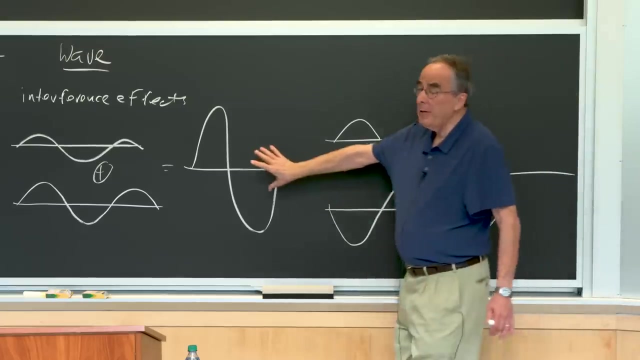 And in fact the addition is a little bit nonlinear. But so we have constructive interference, Or we can have destructive interference And anything in between. If we add these two guys, what you get is nothing. So here you get an intensified wave- constructive- 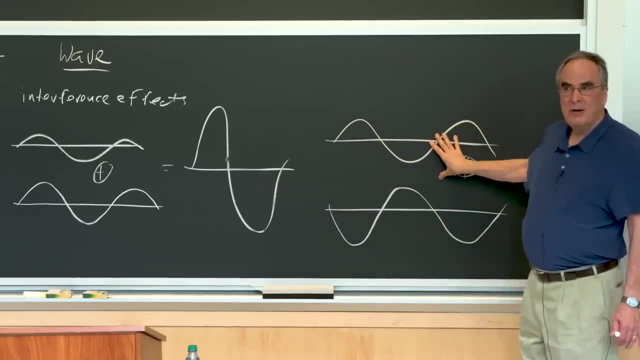 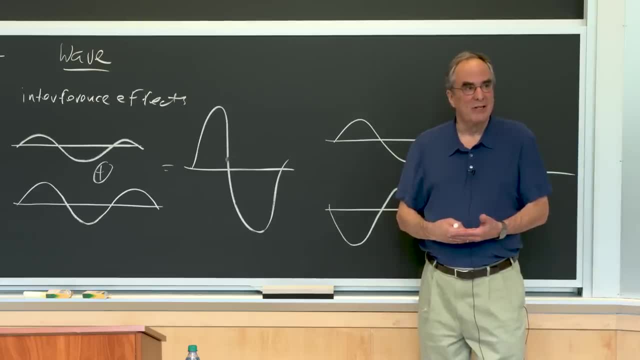 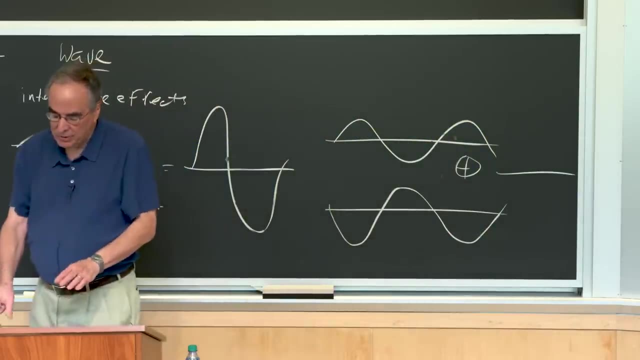 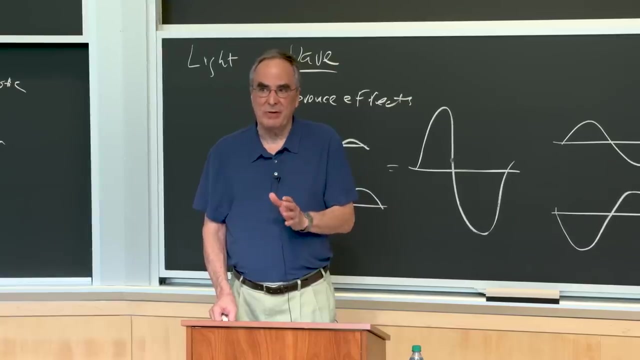 And here we get cancellation. Now it's a little bit stressful to think that if particles have wave characteristics, they can annihilate each other. Well, so you'll have to be prepared for that. So quantum mechanics exploits constructive and destructive interference. 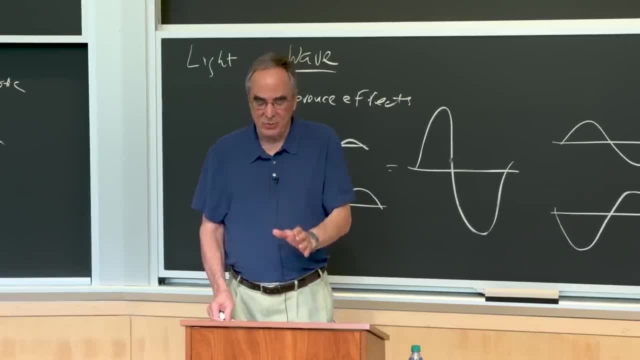 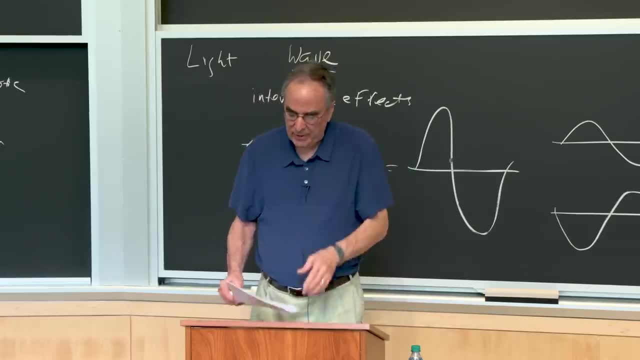 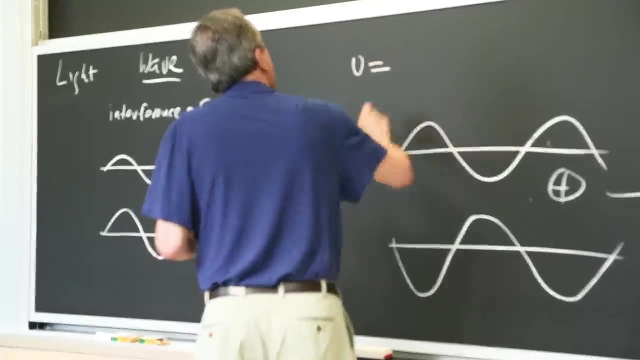 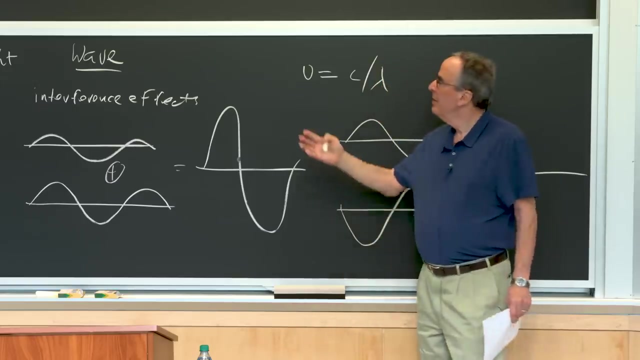 That's at the core And you have to get used to that, And you have to get used to seeing particles do that. So waves have a frequency and a velocity and a wavelength. And now, here, what is new? New is C over lambda. 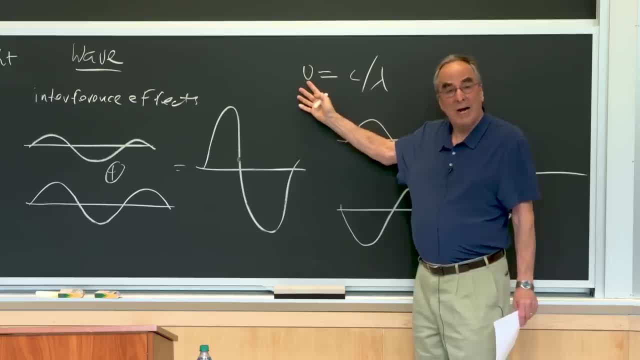 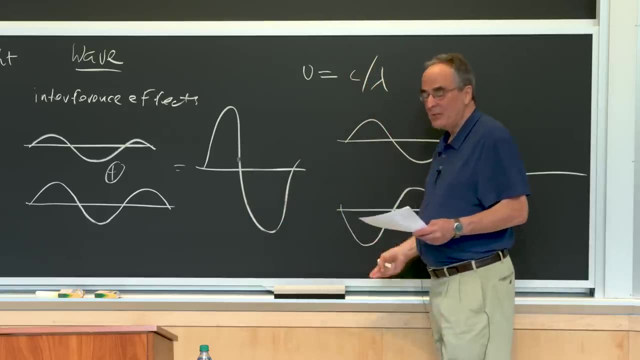 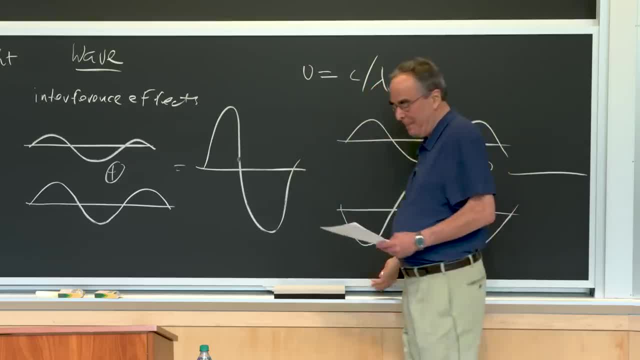 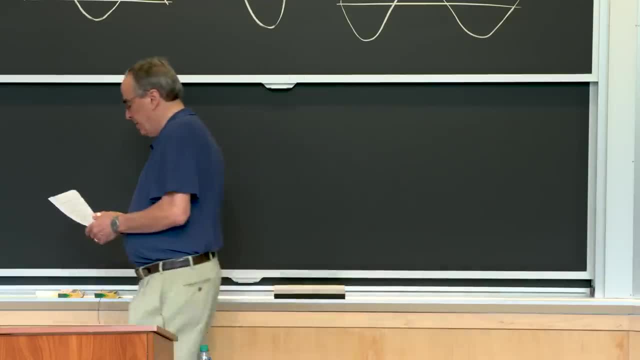 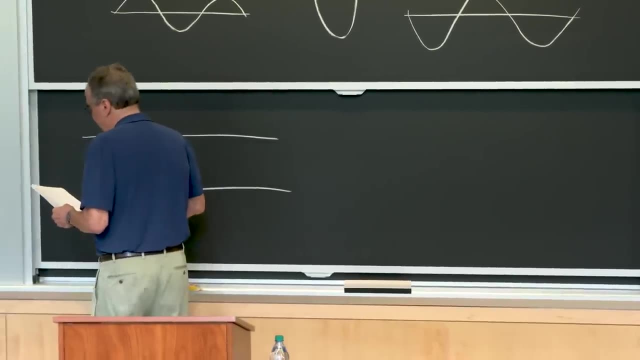 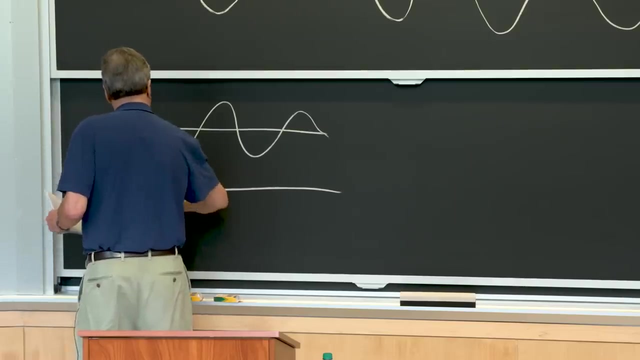 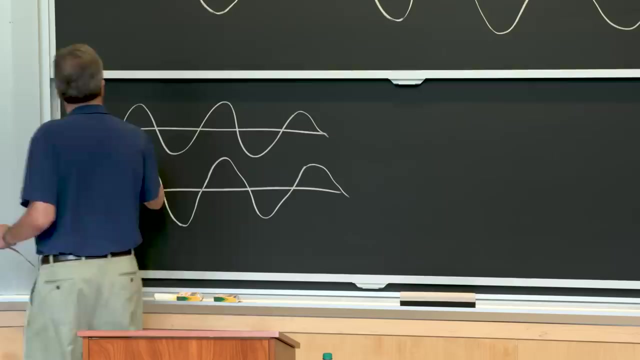 As a repellent and also as a crucial organizing principle. Waves are electromagnetic, And so that means we have transverse electromagnetic waves. And so here is one part of the wave And here is another part of the wave, And this is the electric part of the wave. 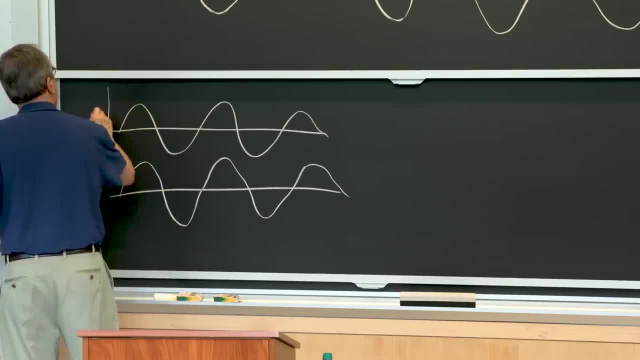 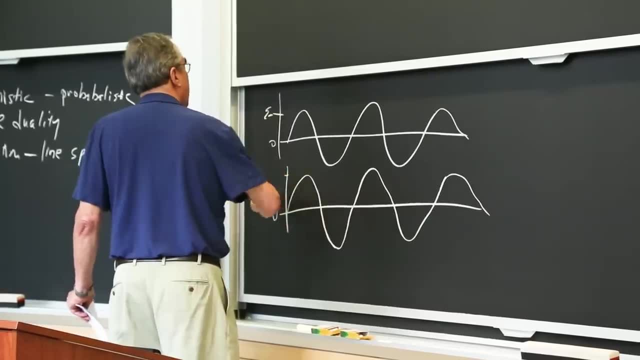 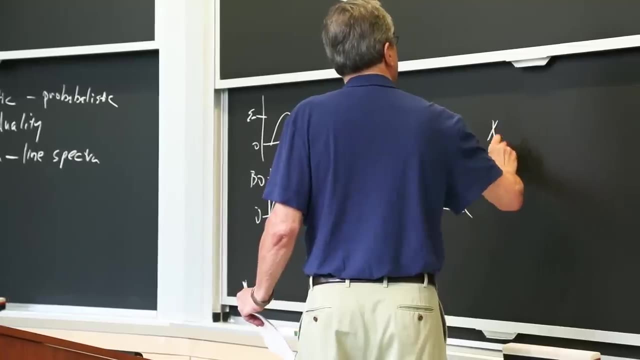 And so we have 0,, and here is E0.. And this is the magnetic part of the wave 0, and B0.. And this is in the xz plane. This is the z direction. This is the z direction. 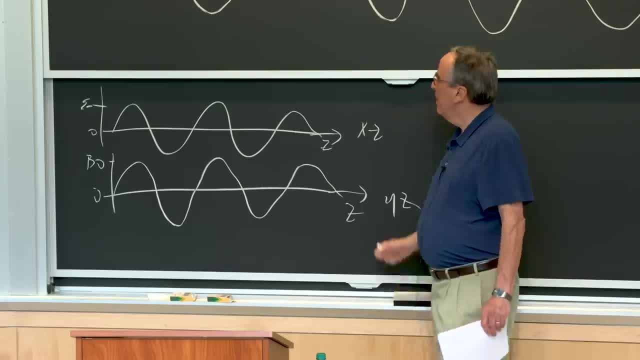 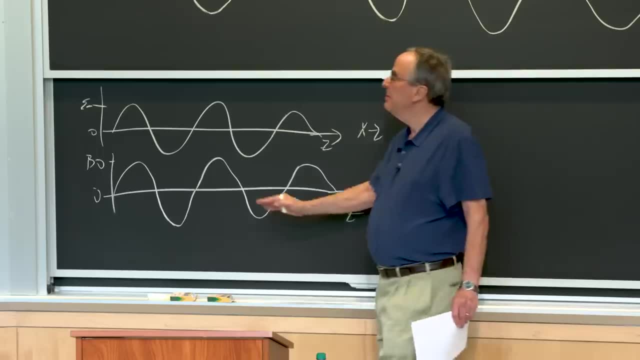 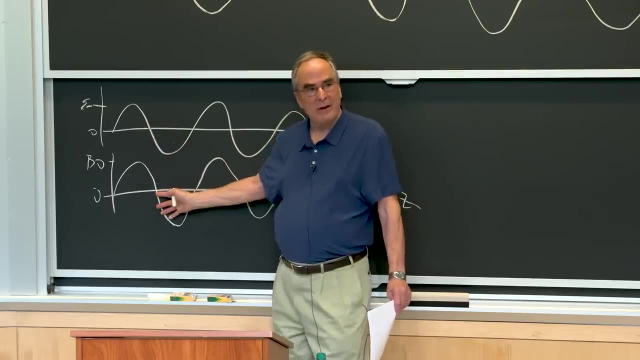 And this is the yz plane. Now this corresponds to a wave which is linearly polarized along the x-axis, And so it's kind of hard to draw a transverse electromagnetic wave. But there's an electric part and a magnetic part. 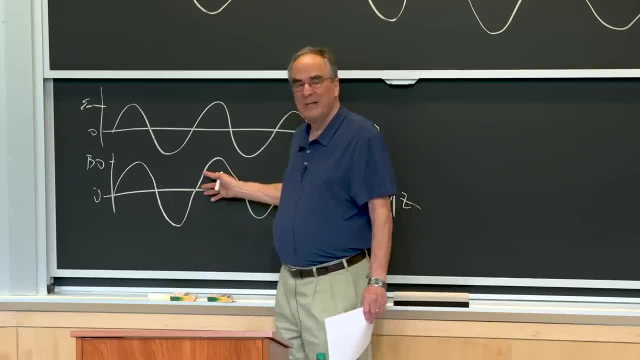 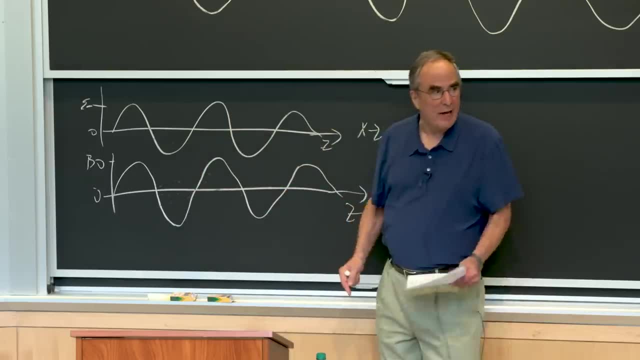 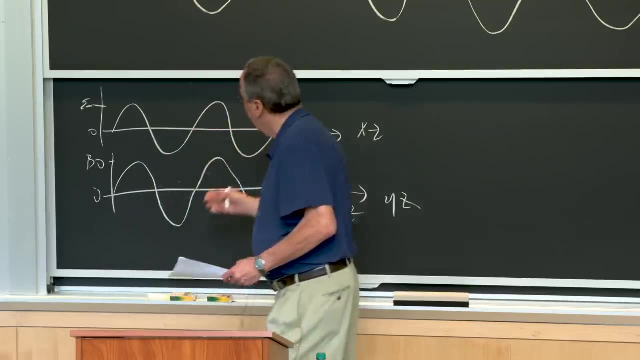 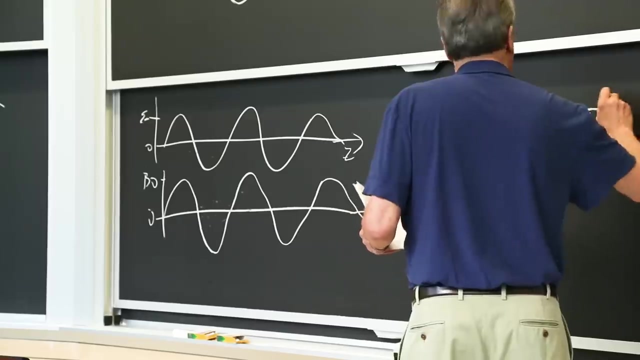 And for the most part I forget about this In magnetic resonance. this is the only thing you care about. But they're both part of light And OK. So we have these waves, And now the intensity of the light is proportional to the E0 squared, the electric field. 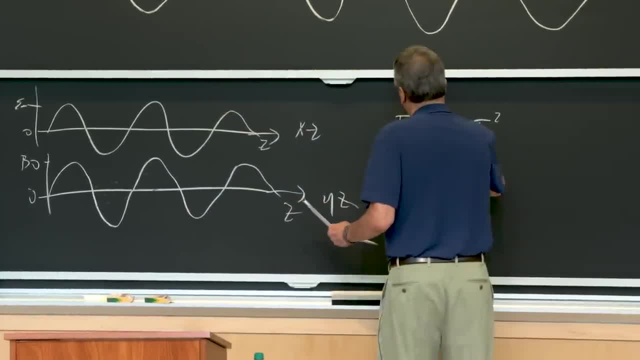 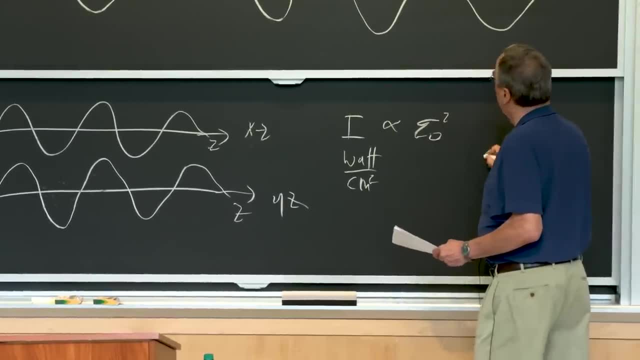 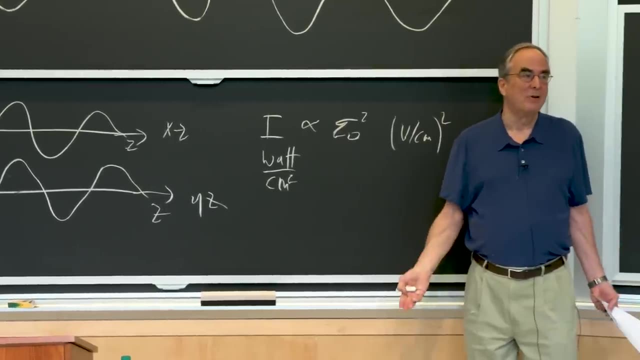 squared, And it's also measured in watts per square centimeter. And this is in. So this is in volts per centimeter squared. Now, I'm an old-fashioned guy. I use centimeters instead of meters. You'll just have to forgive me for that- not using MKS units. 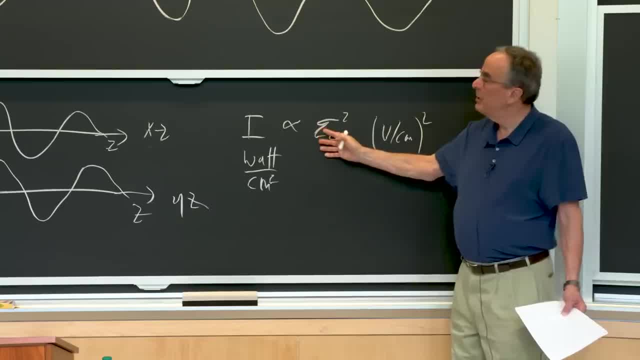 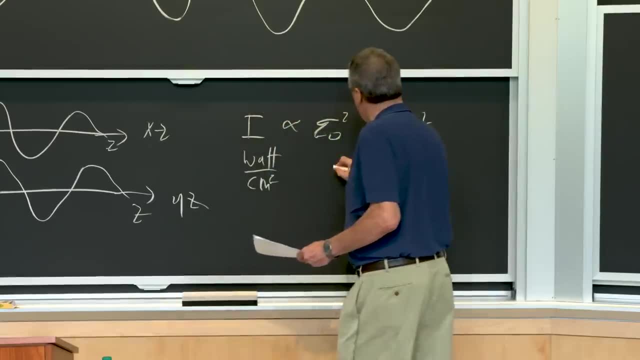 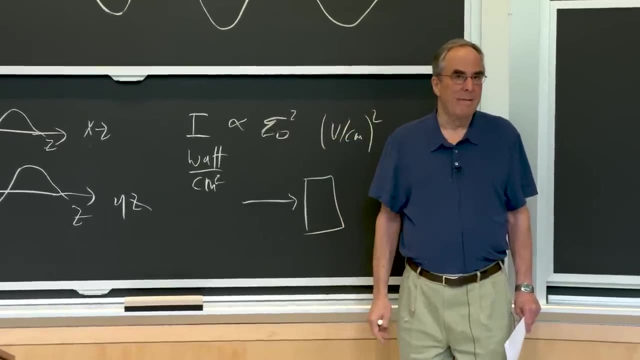 But the important thing is that the intensity is related to the square of an electric field. So suppose we have light impinging on a hunk of metal, The Starting Line. What will that be? Is that a beam of light, Or it'll be a beam of light? 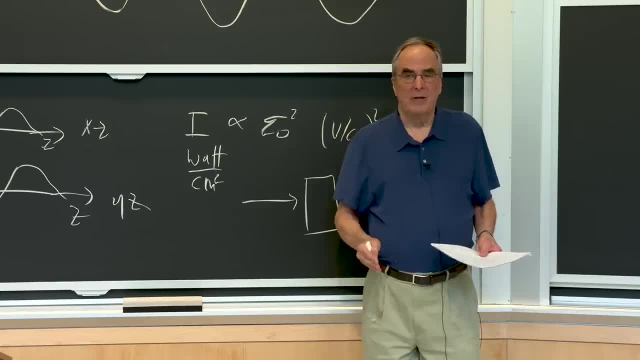 What if we have a beam of light on a hunk of metal? Well, what would it do? It's a beam of light. Think about it. What if it's a beam of light, You could ask yourself. It would be a beam of light. 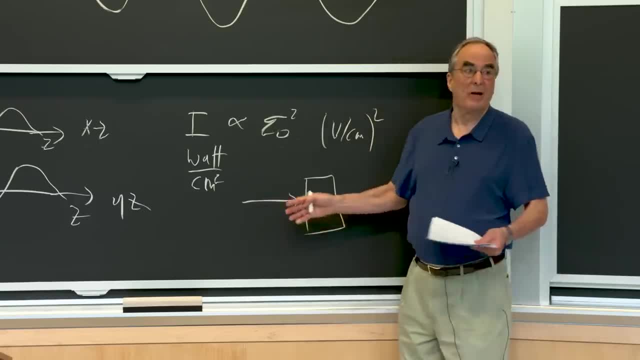 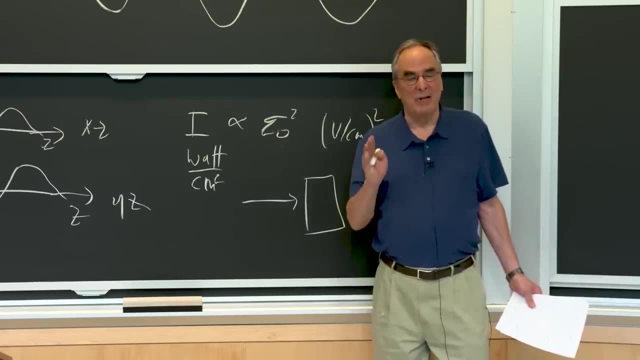 What will happen when we put a beam of light on a metal? Well, that's a different question. It's a beam of light on a metal. The space is just the same, So it's not all very unique. The beam of light is a beam of light. 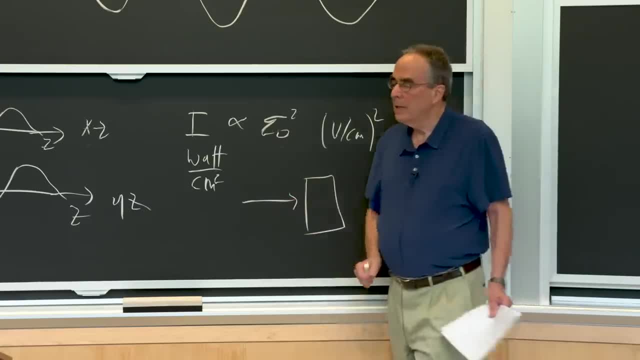 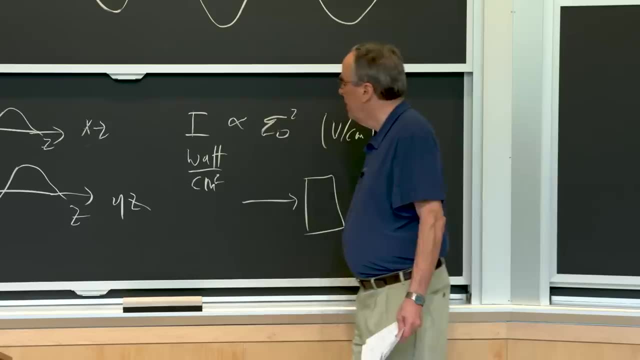 And let's say a metal. Well, we'd have to figure out what if we put a beam of light on a metal And it's pushing the electrons around, because that's what an electric field does: It moves the electrons, And so you would expect, classically, 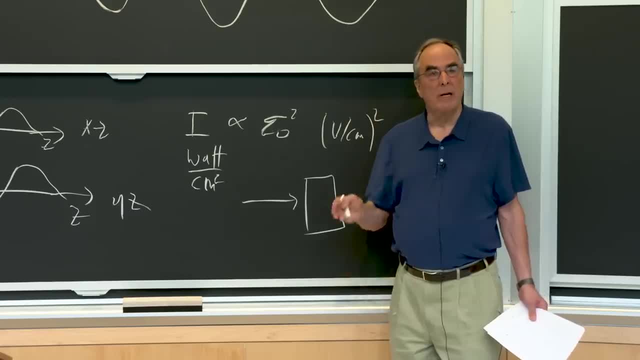 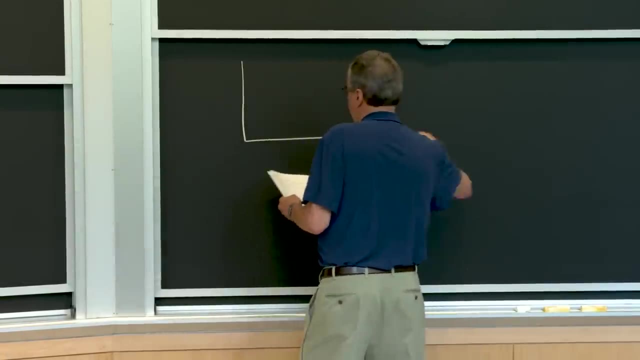 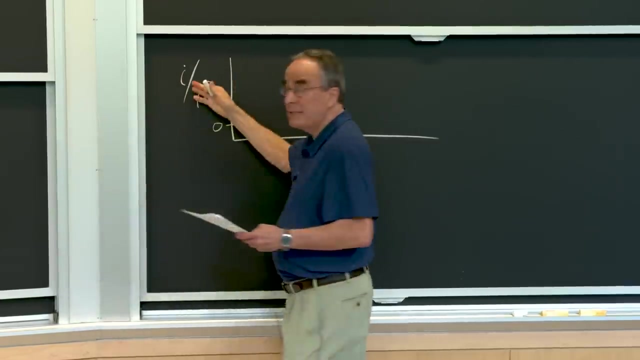 that, at high enough intensity, you're going to start ripping electrons out of the metal, And that would be wrong. And this is the photoelectric effect. This is what we observe. Zero, The current divided by the charge on the electron. So that's the number of electrons per second. 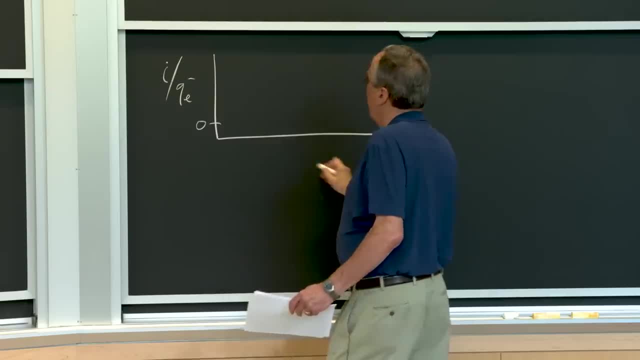 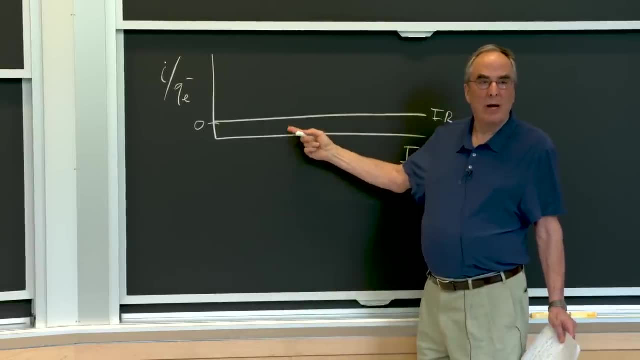 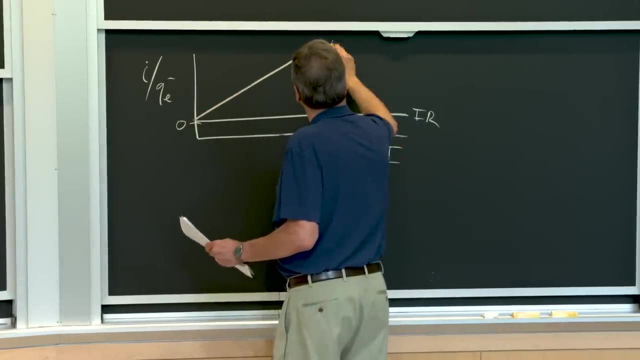 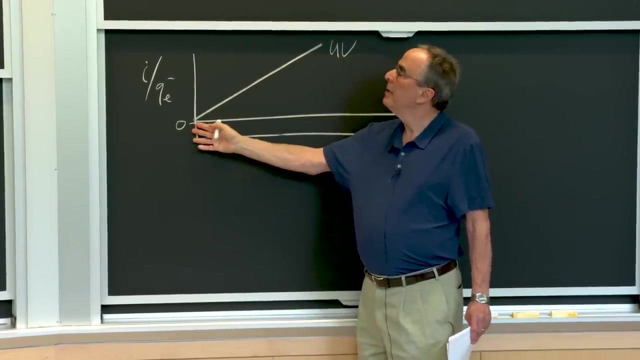 And this is the intensity. And if we have infrared radiation, nothing happens, no matter how strong it is. If we have ultraviolet radiation, we have something happening: It's the intensity of the light increases The number of electrons per second ejected from the metal. 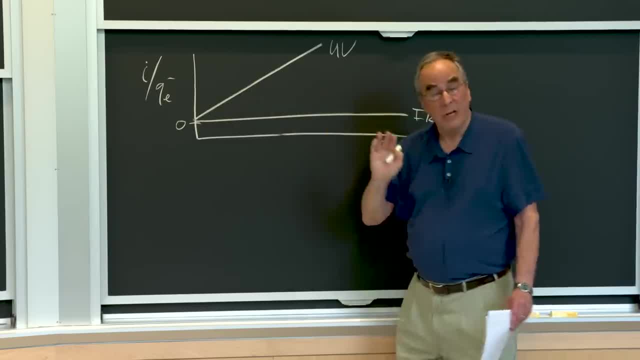 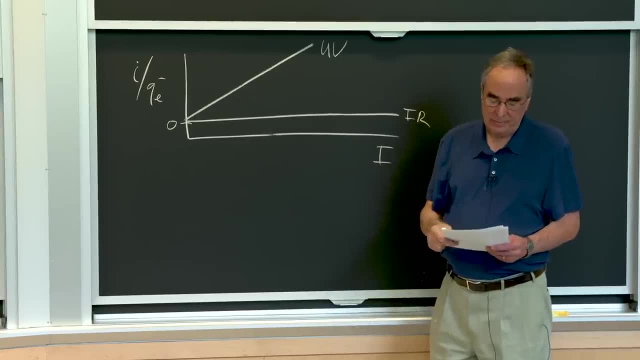 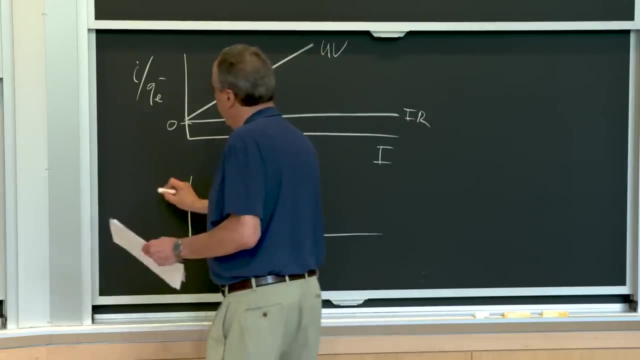 increases linearly. So why is that? We expected it would be intensity that determines it, But it's the color of the light that determines. We can also do something like this, where we again ask: OK, What is the current divided by the charge? 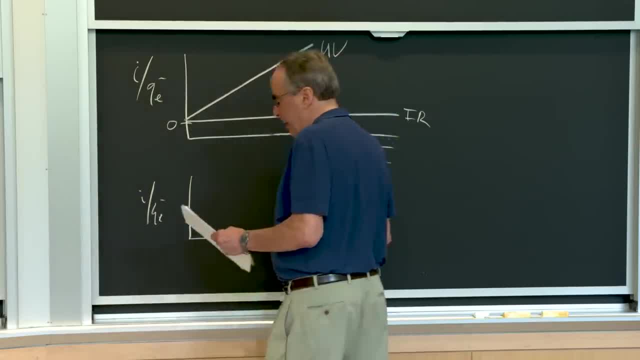 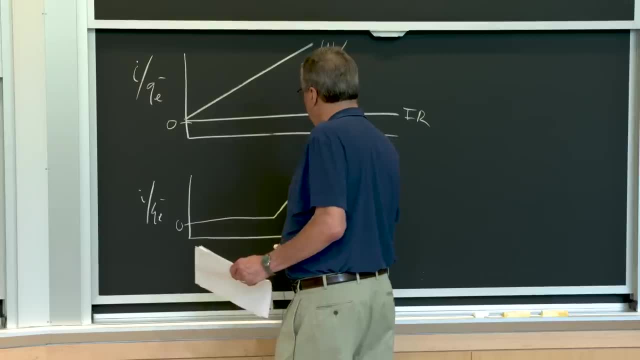 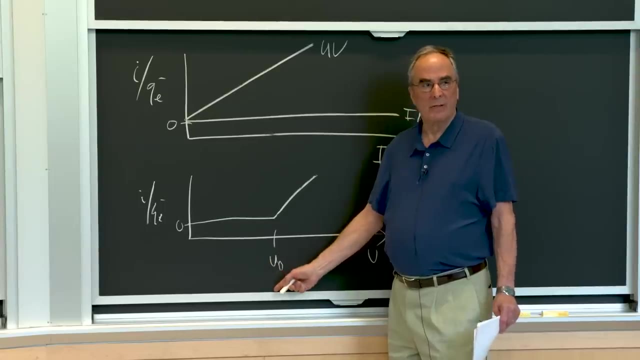 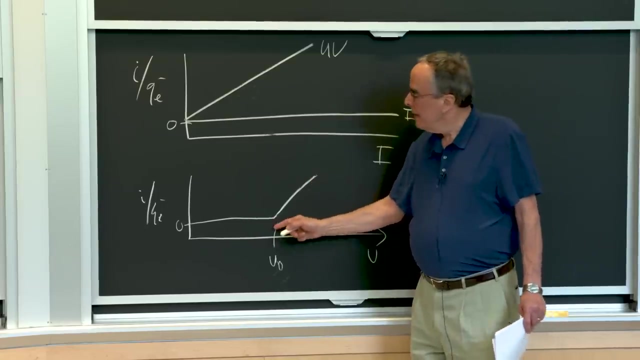 of the electron versus frequency. And again we have zero here And what we see is nothing up until some critical point. And then this is some special frequency which is different for every metal, And then all of a sudden, we start getting electrons. 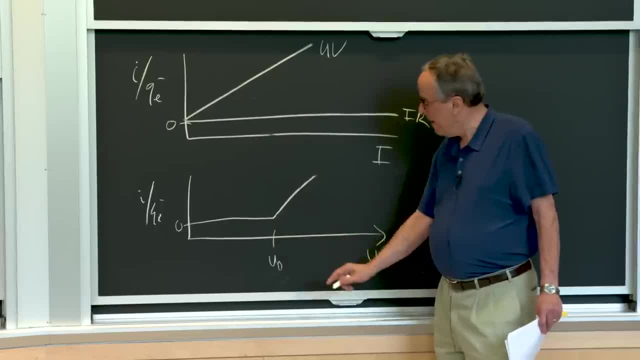 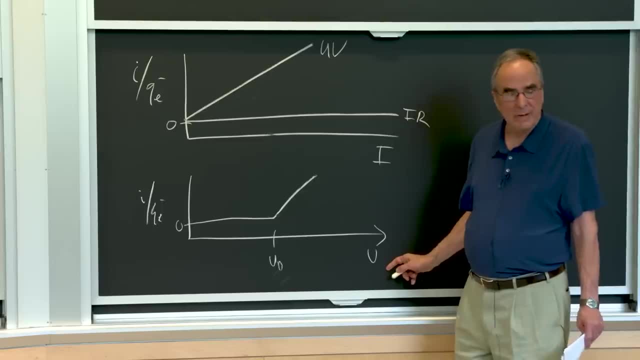 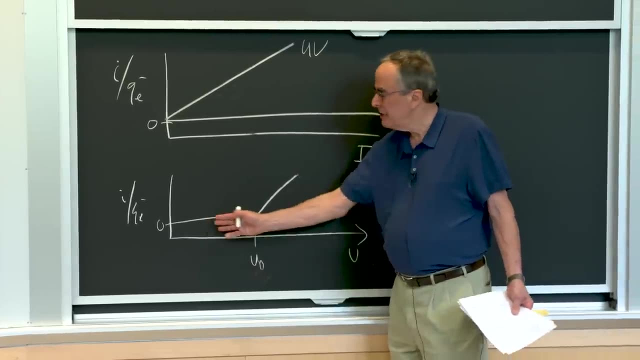 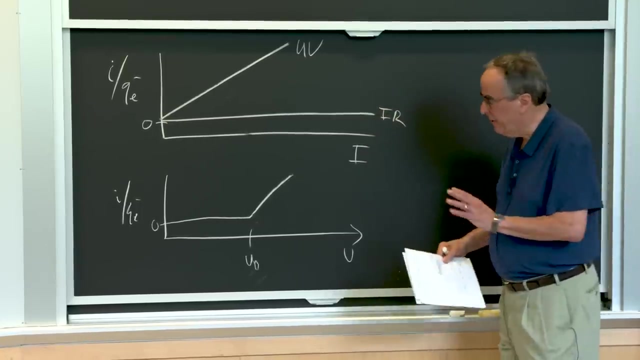 And this Increases linearly, or at least for a while, increases linearly with the frequency. So there's something about the frequency of light that rips out the electrons. It has to be above a certain minimum And then the electrons increase with the frequency. 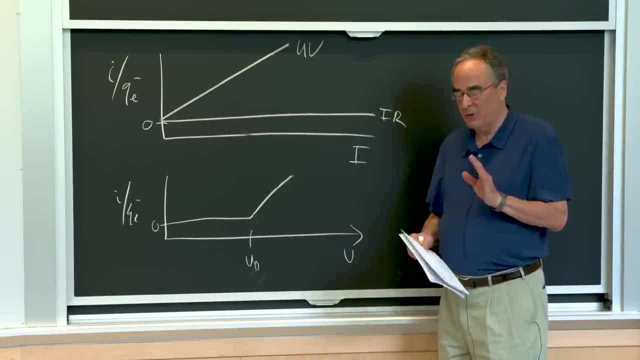 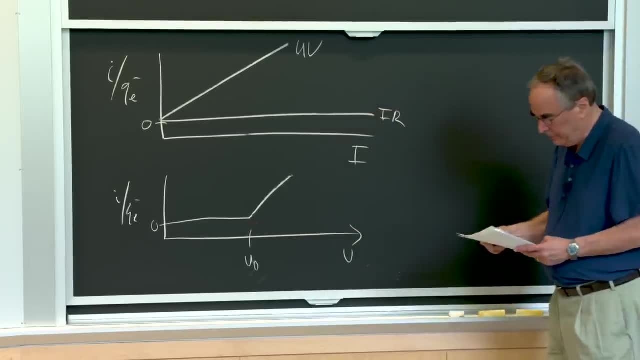 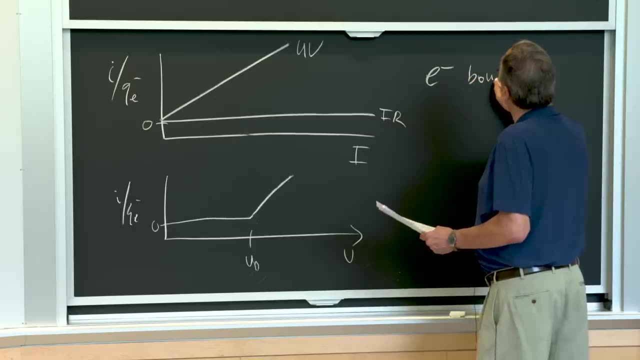 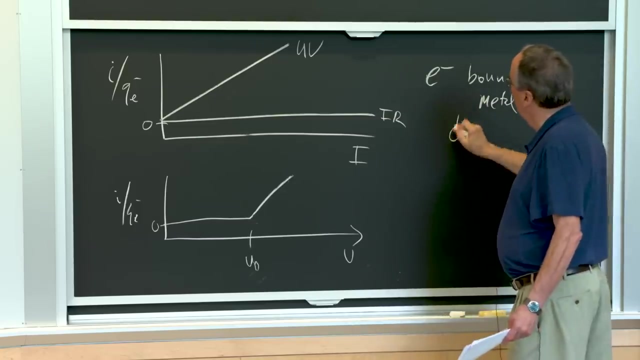 but in a little bit more complicated way than linearly, And so I have something in the notes which is not quite right, But this, This onset, is important. So these observations suggest that the electron is bound to the metal by some energy, which we call the work function. 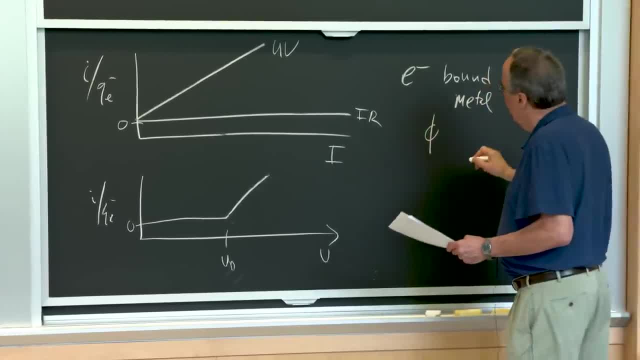 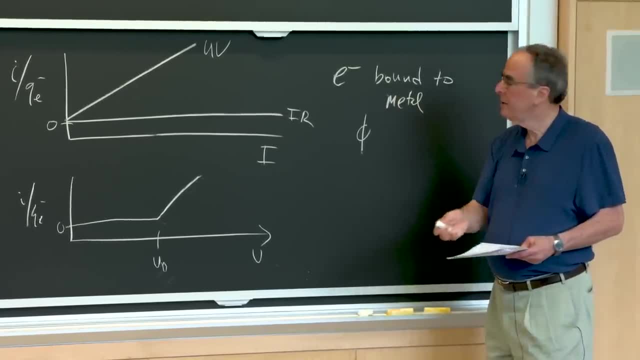 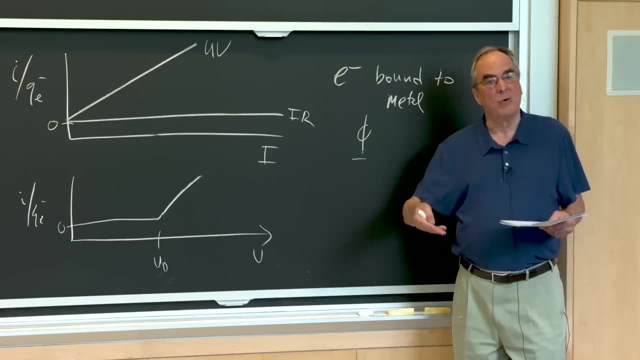 And it's called phi, And so this is an energy that it takes to rip an electron out of a metal, And so it's called the work function, And work functions for metals range from a little over one electron volt to around five electron volts. 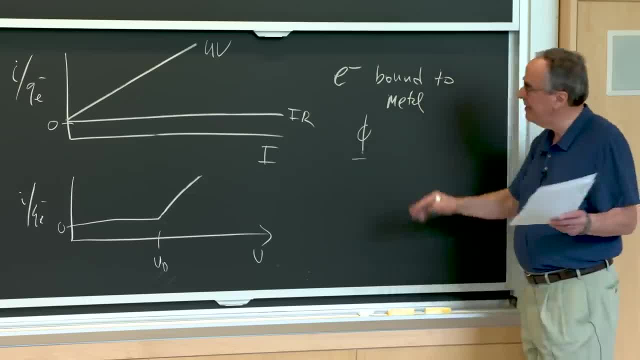 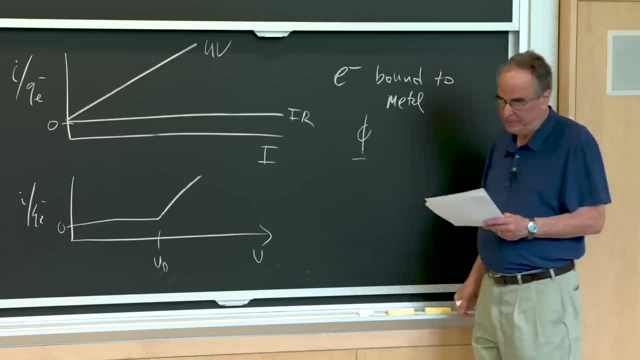 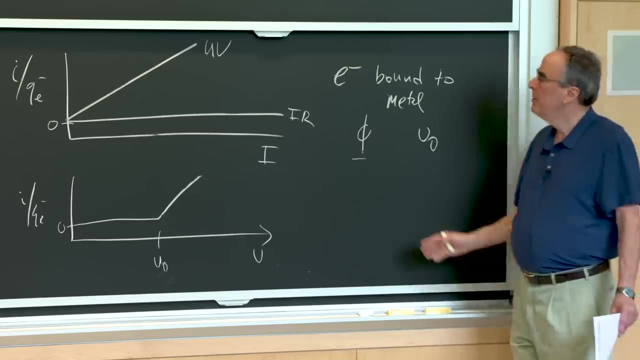 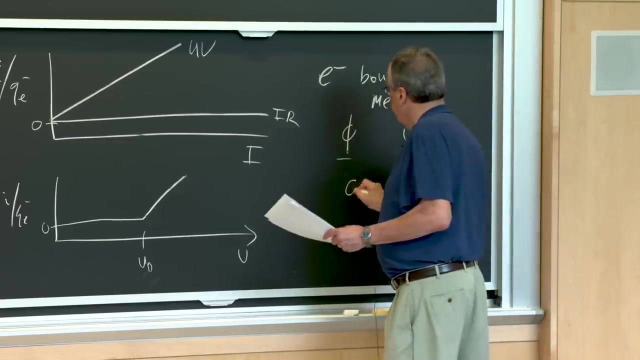 These are. I'm going to use those units. You can forget that, But all metals are within a relatively narrow range of work functions And this is somehow related to nu zero. So this is an energy And this is a frequency, And so we expect that there is some relationship. 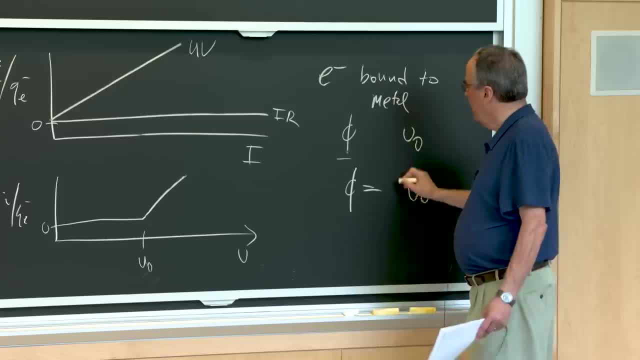 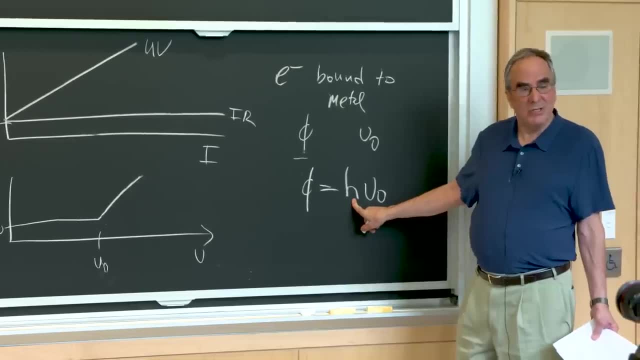 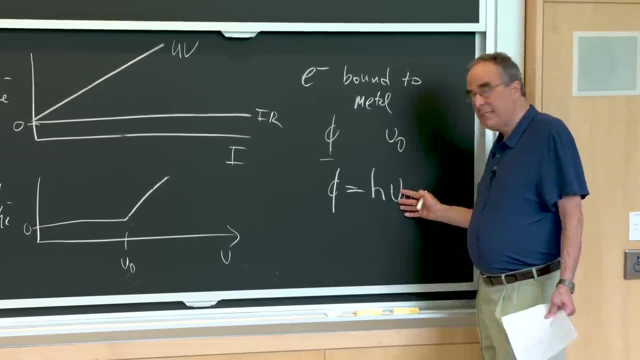 between nu zero and this energy, And there is some proportionality constant which I can call anything I want, but I'm going to call it h because it's going to become Planck's constant. That's a proportionality constant, And so the onset of ejection of electrons is when the frequency 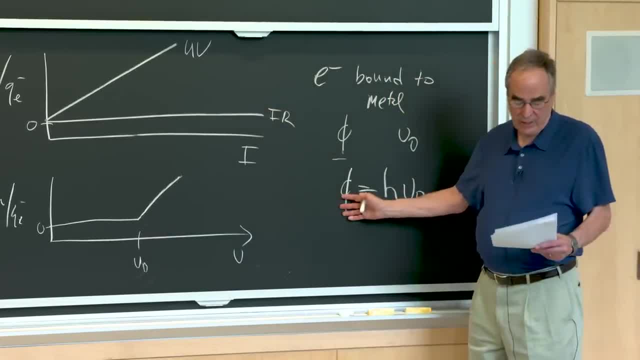 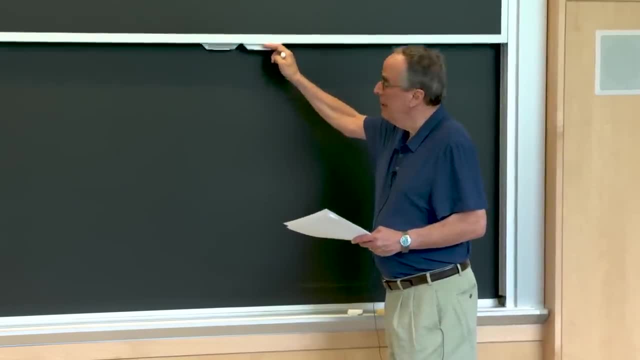 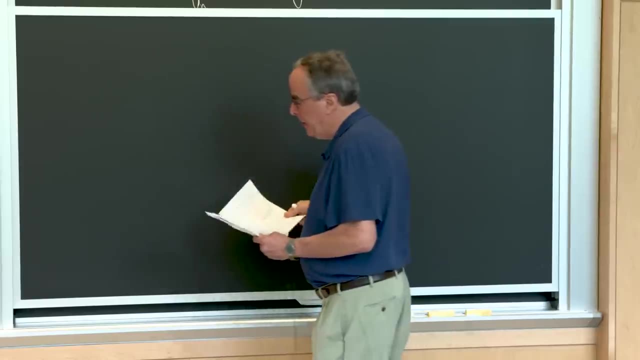 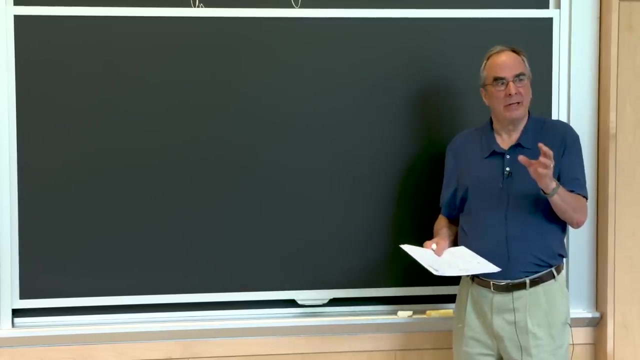 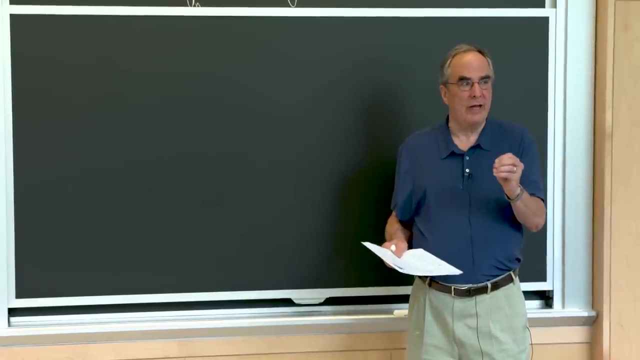 where- Yeah, Yeah, Yeah, Yeah Yeah of light is greater than the work function. As I said, every metal has a different work function And OK, So this is looking like somehow the light does not act in an additive way on the metal. 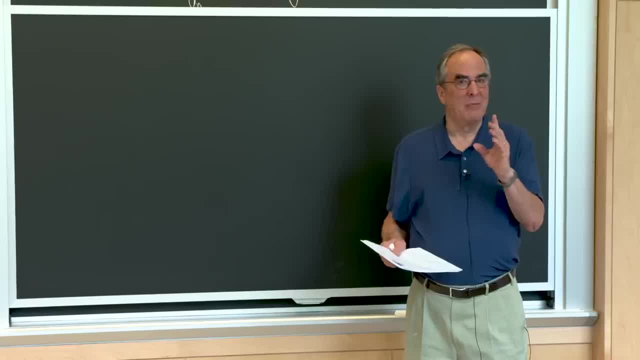 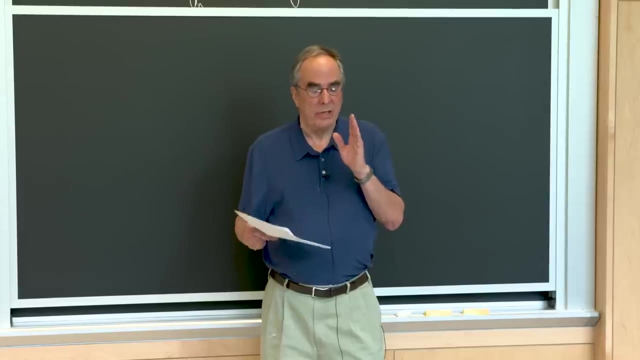 It acts in a singular way. somehow There are particles of light that have definite energy. This is what it looks like, And we're going to call those particles of light photons. And so now we're trying to think of all right. electromagnetic radiation comes as particles. 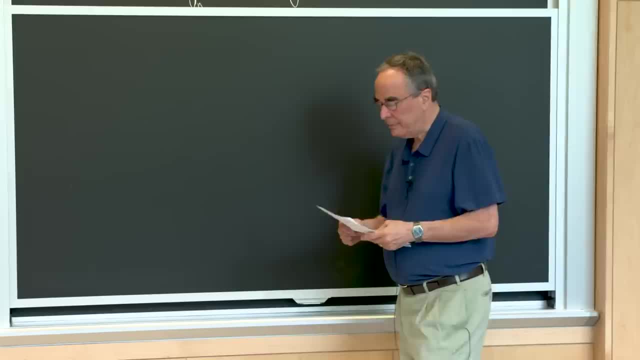 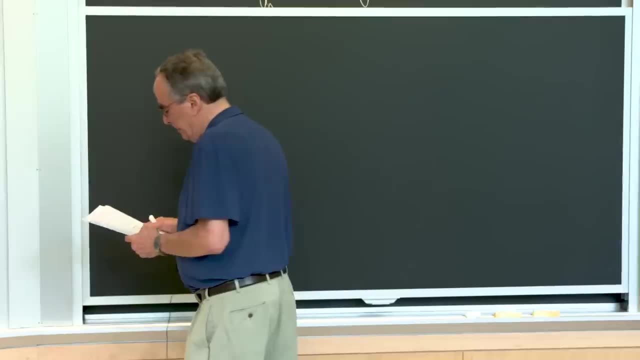 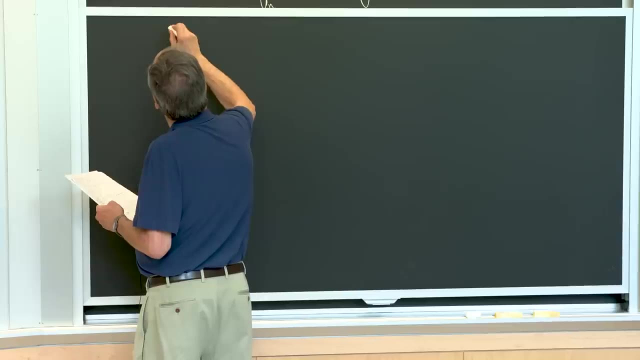 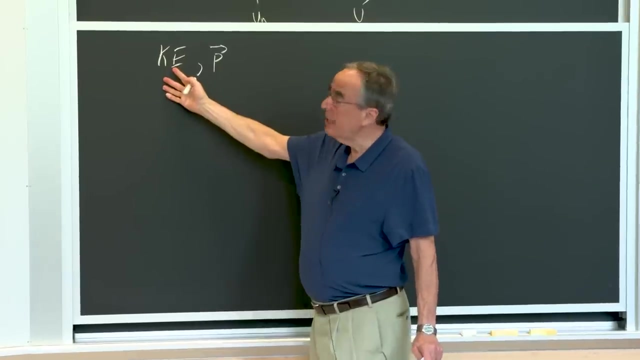 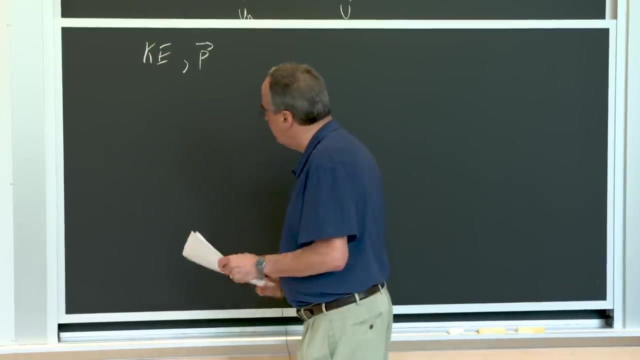 What are the properties of particles? Well, particles- well, I'm getting ahead of myself, But as long as I said this, particles have kinetic energy and momentum. Kinetic energy is a scalar quantity, Momentum is a vector quantity. And right now, what we want to do. 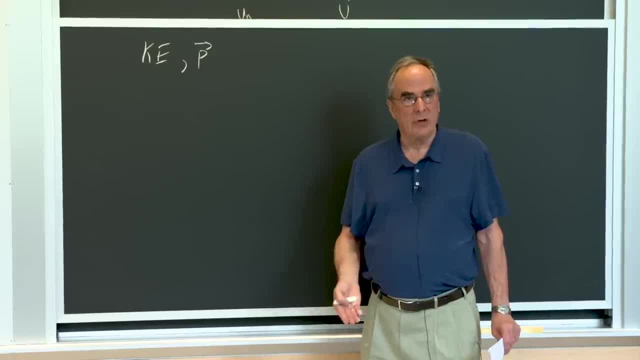 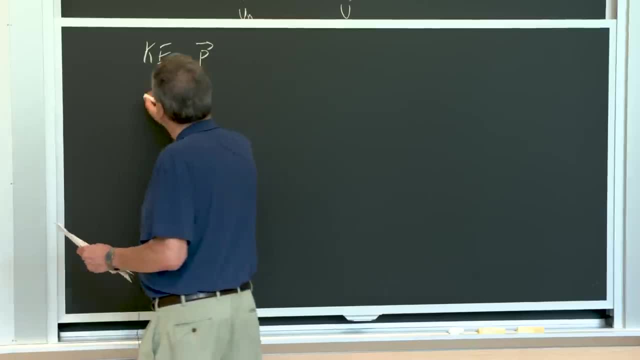 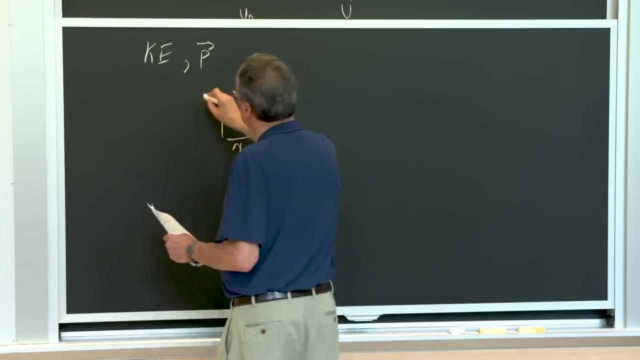 is measure the kinetic energy of the electrons that are produced by the annihilation of photons. OK, And so we can imagine an apparatus like this: Here is our metal, And here is the light impinging on the metal, And we have grids. 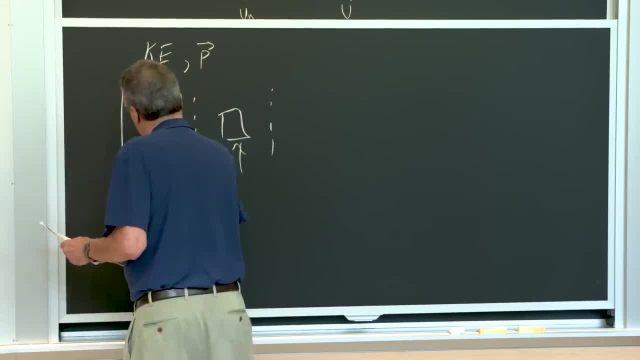 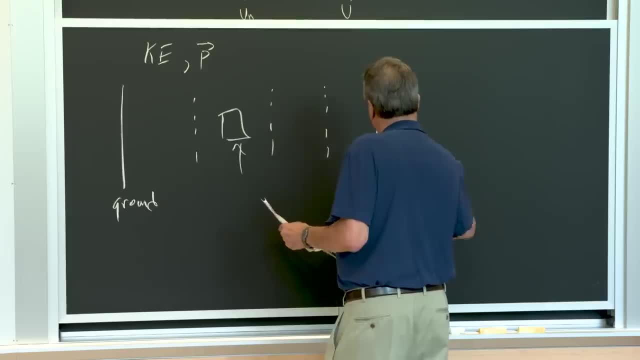 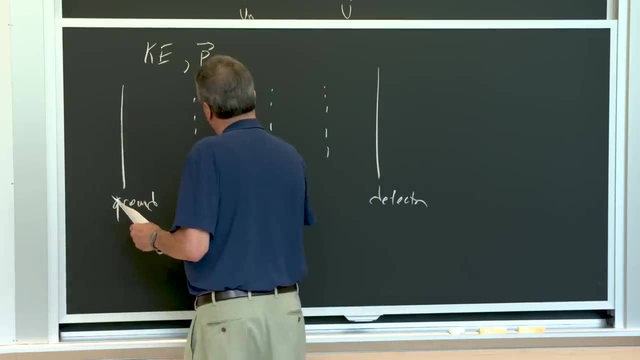 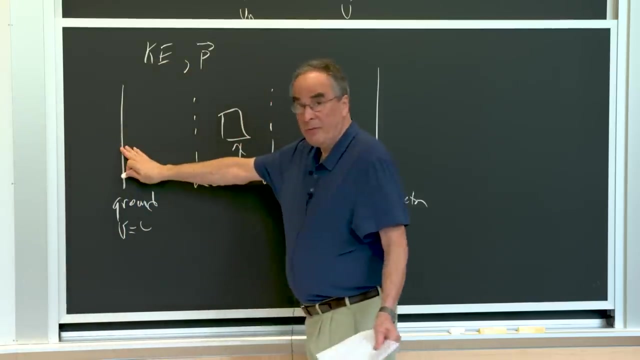 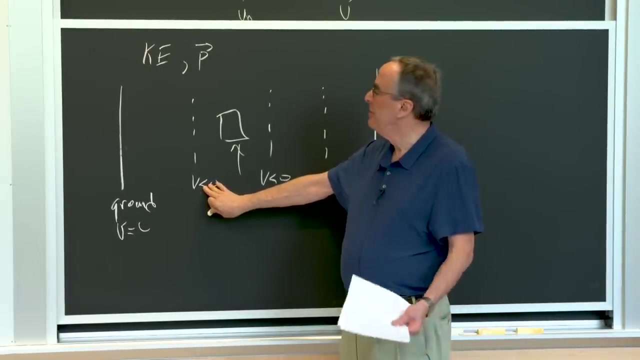 We have a ground And we have another grid And a detector. So we have ground. The voltage is 0.. Here we have a voltage less than 0. Electrons don't like that, But these two grids are at the same potential. 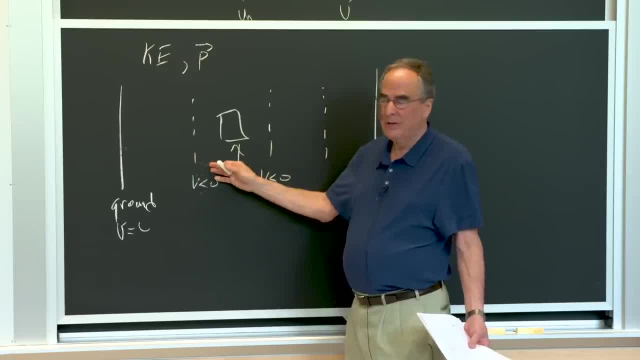 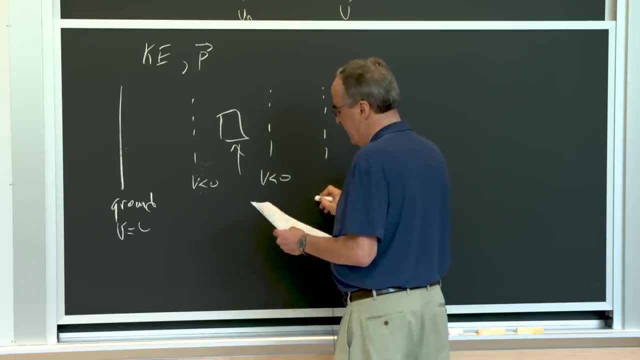 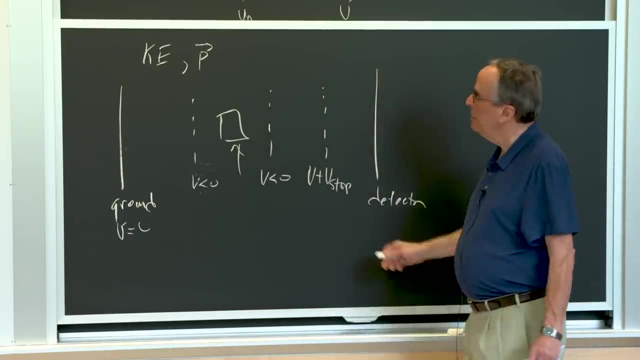 So the electrons, OK, OK, OK, OK, OK. Don't know which way to go. And then there's another grid where we have the potential is v plus v, stop. And so what happens is if the electron is ejected. 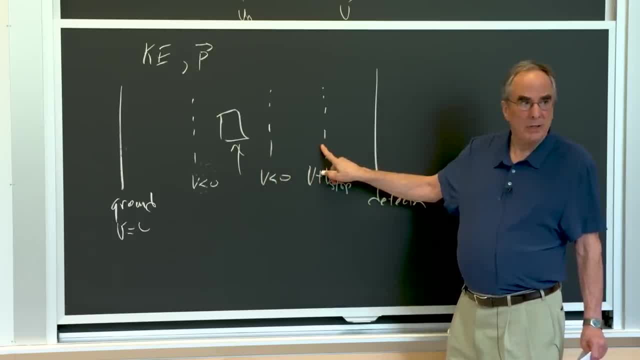 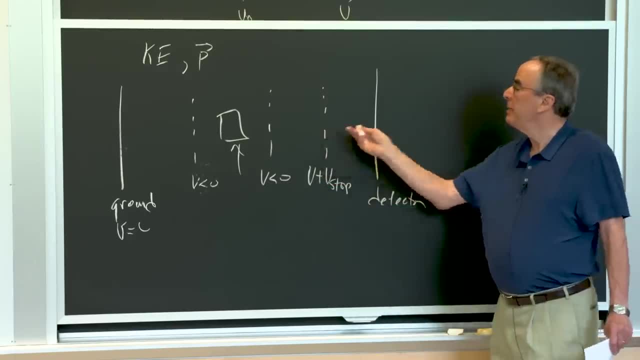 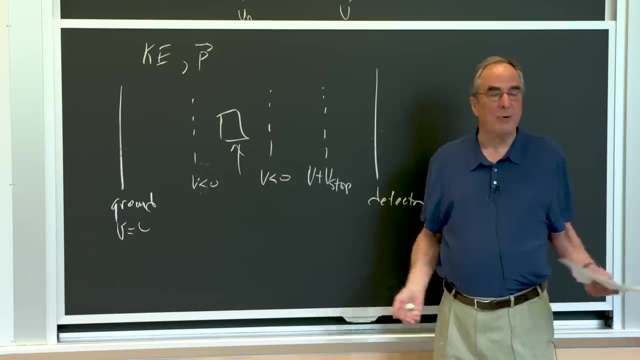 with enough kinetic energy to go uphill and cross through this potential, this grid, then it will make it to the detector And we'll count it. So this is just a crude apparatus. If you were going to do this experiment, you would probably design it better. 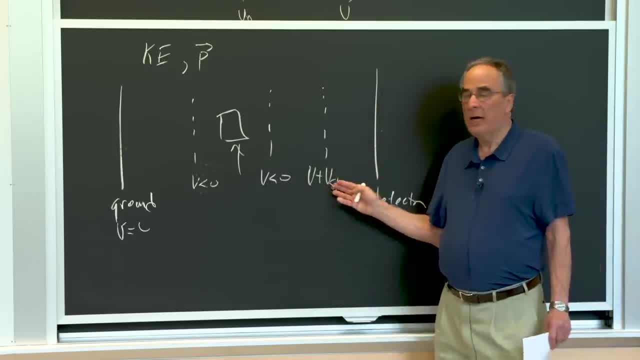 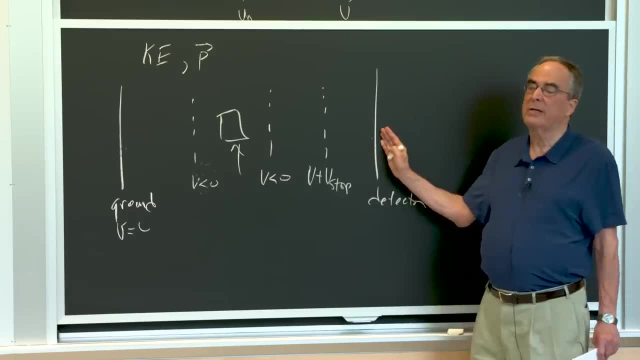 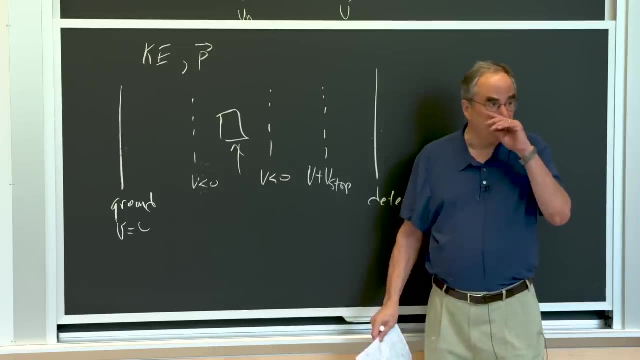 But the idea is, what we want to do is to measure what is the voltage that we apply that causes the electrons to stop reaching the detector, And that's the way we measure the kinetic energy- The kinetic energy of the electrons, When all of the electrons stop hitting the detector. 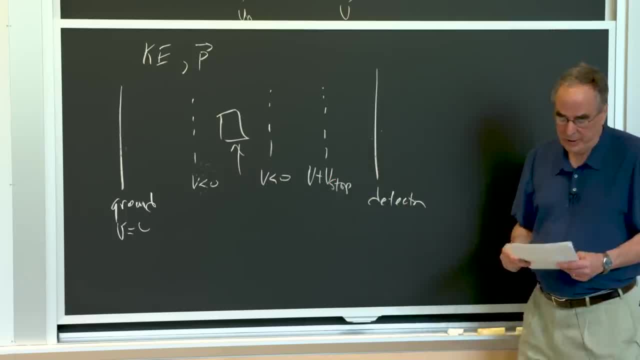 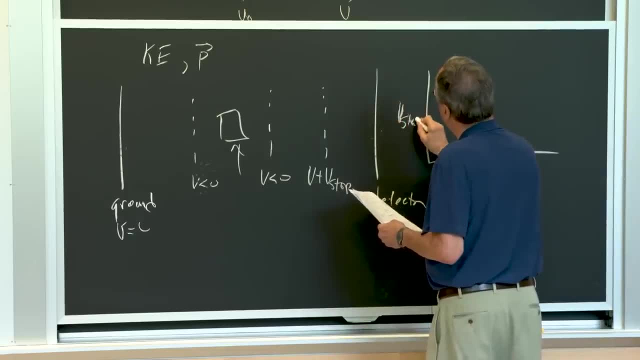 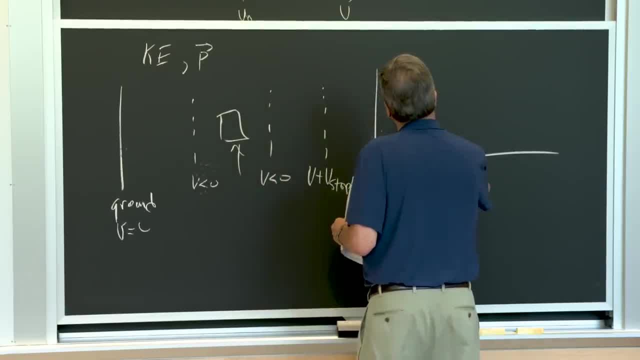 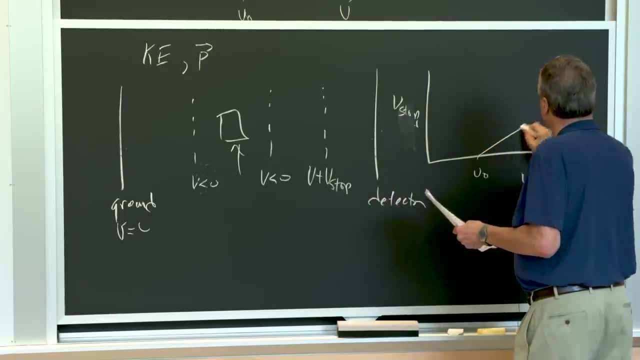 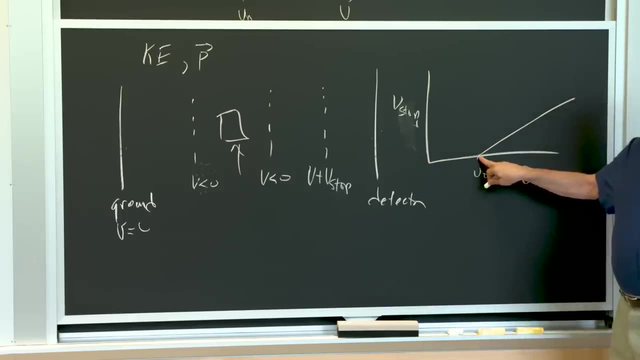 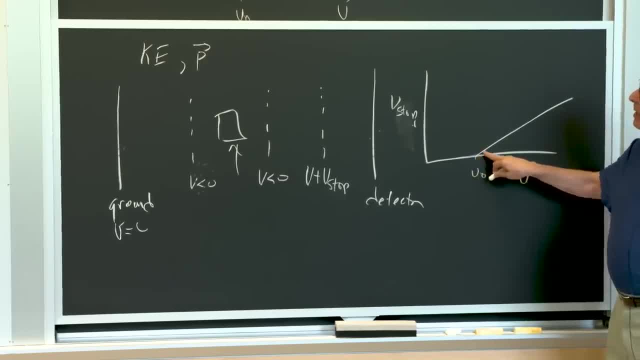 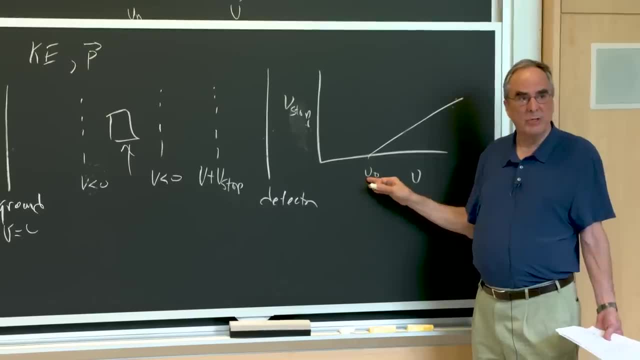 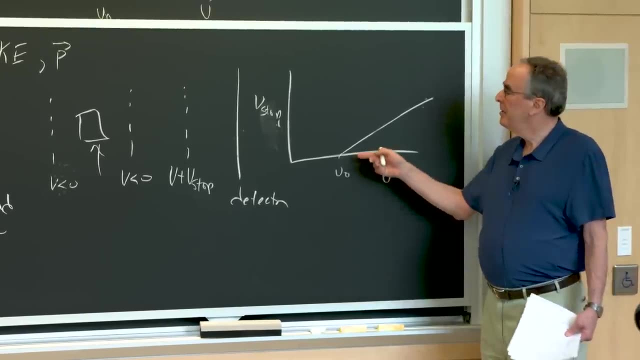 Once we're above nu 0, electrons start being ejected And they have a kinetic energy which is measured by v stop And it increases linearly with frequency. Now, when we do this experiment on different metals, the slope is constant the same. 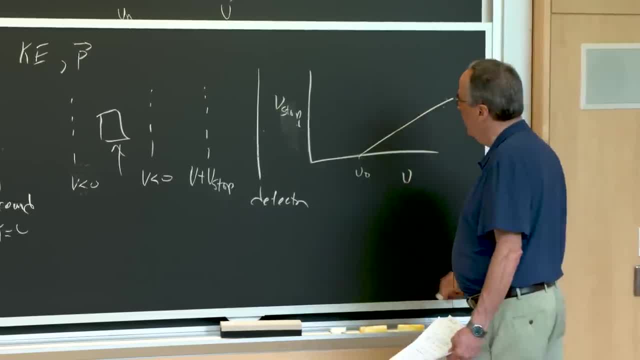 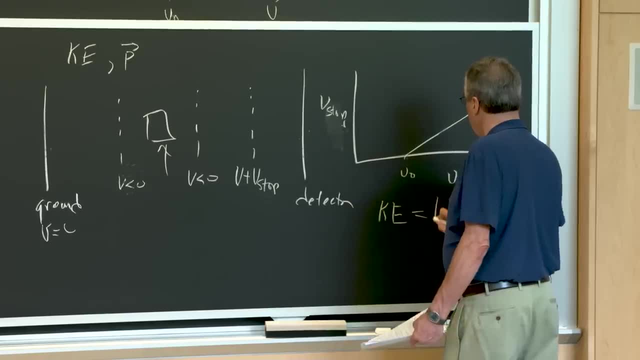 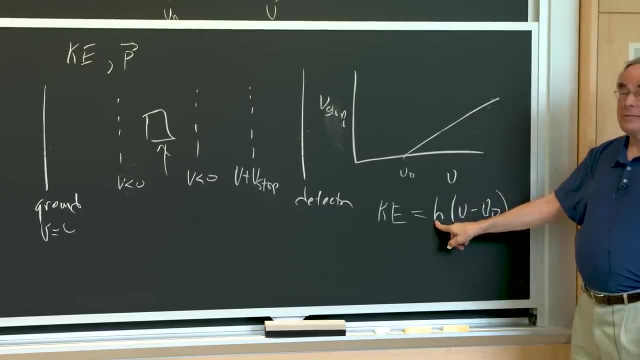 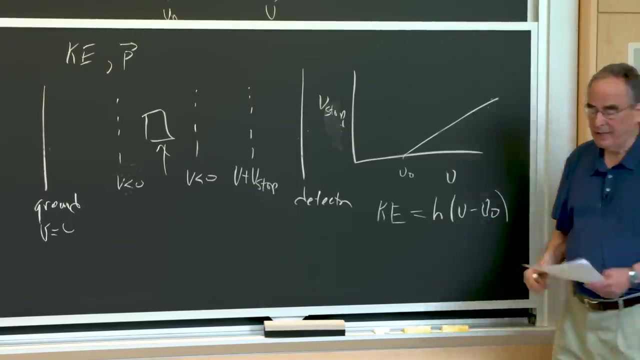 It's universal. So the kinetic energy of the ejected electrons is equal to some constant. It goes as nu minus nu 0.. And this is the same constant that we saw before, And this is Planck's constant. And now what we've seen is that these 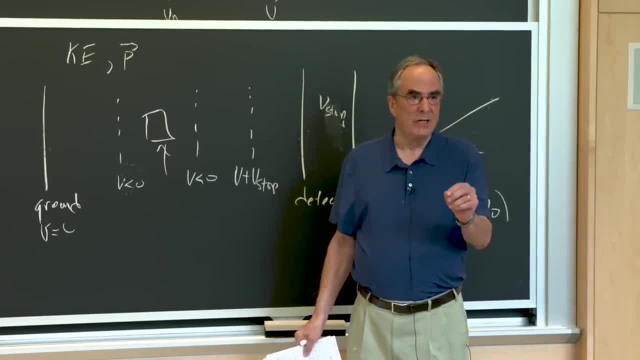 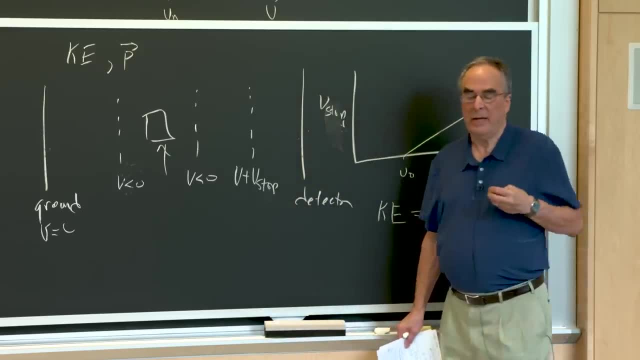 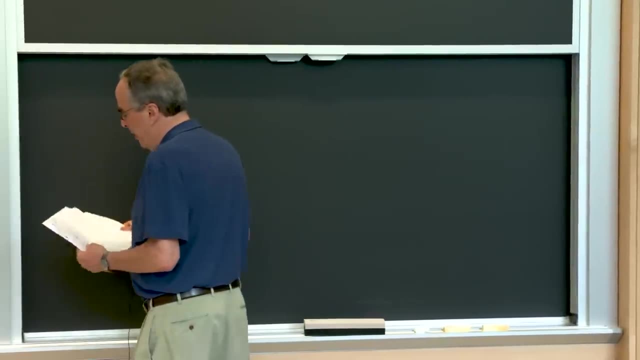 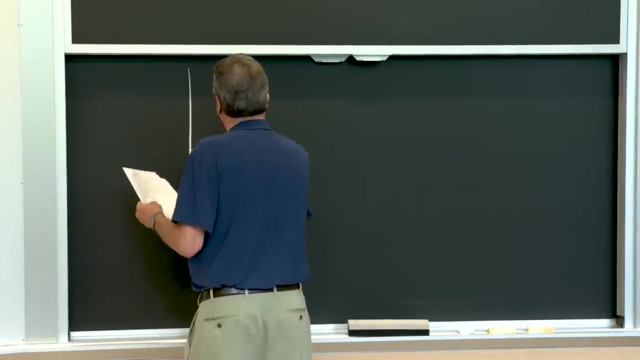 these particles of light have definite energy. They have definite kinetic energy And we can stop And they transfer that energy, And so we can draw an energy level diagram. So here is 0. And here, So this is energy. OK. 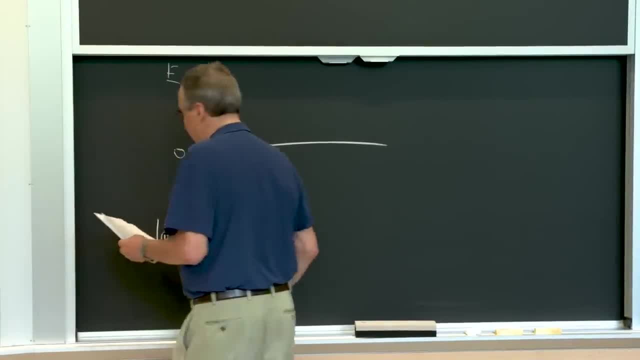 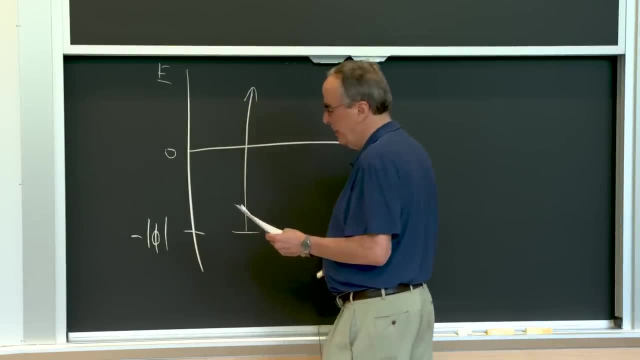 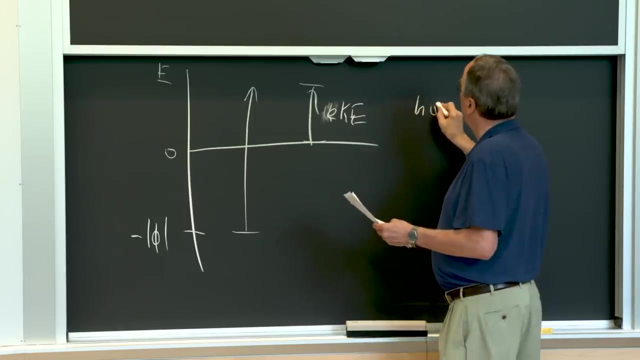 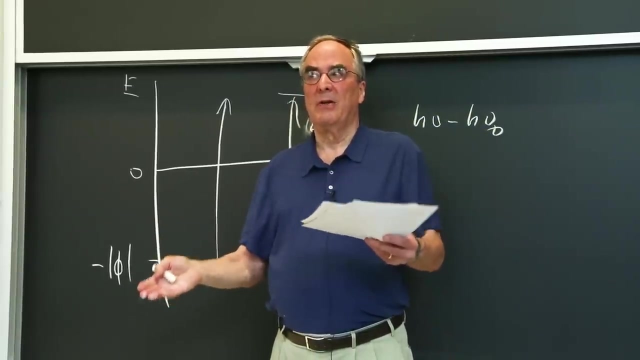 And this is minus the work function. And so we have a photon which has this energy, And we have the kinetic energy of the electrons, And this is h nu minus h nu 0.. So, OK, The story is complete. The photoelectron effect is the easiest thing. 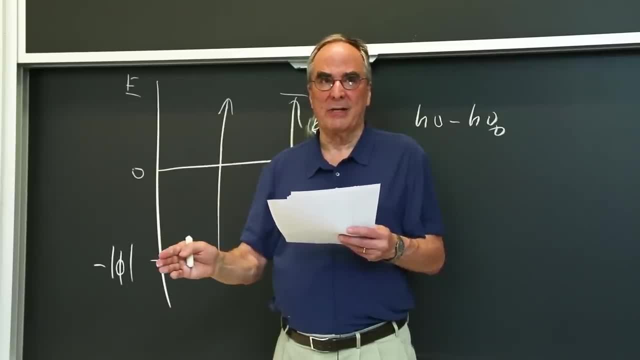 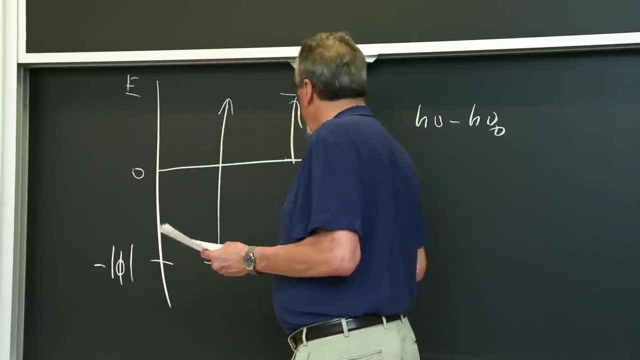 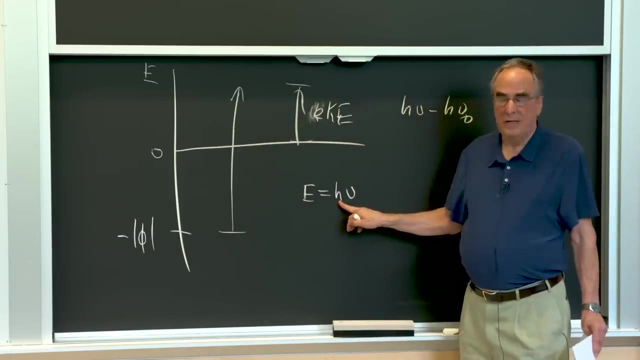 to understand at the beginning of quantum mechanics, And it says that light comes in particles which we call photons, And the energy of a photon is h, nu. h is a fundamental constant And we know what nu is And it's exactly what it is. 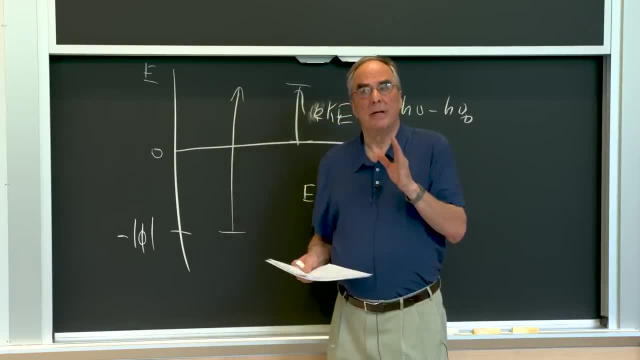 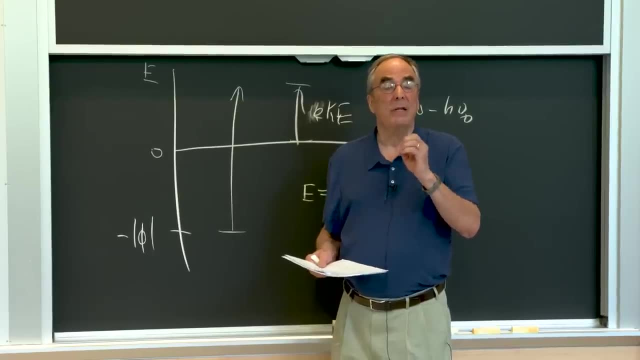 And we know all the facts. So I'm going to try to compare the effects of this And I'm going to shoot you a couple of results. We'll get to that in a minute. But now let's look at the energy of a photon. 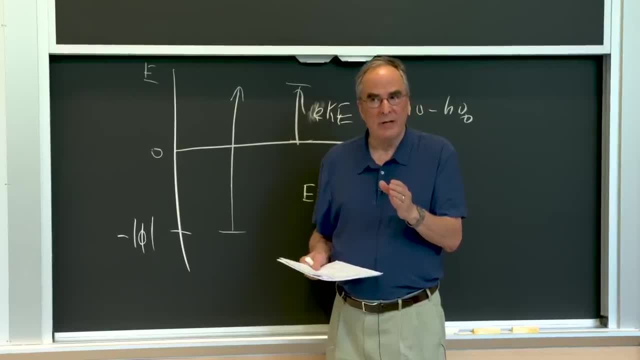 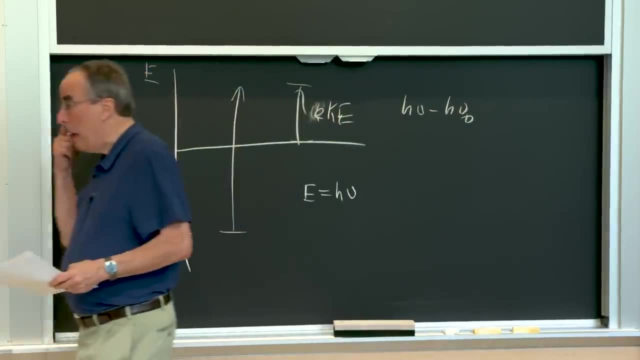 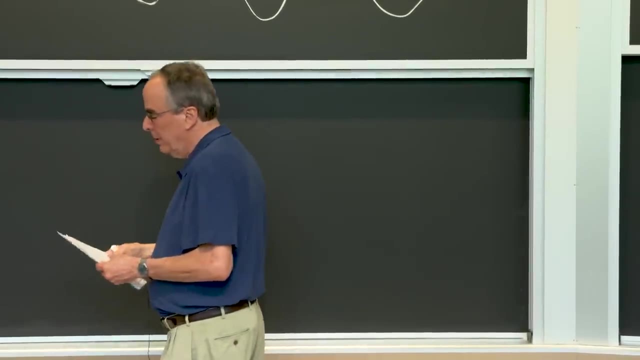 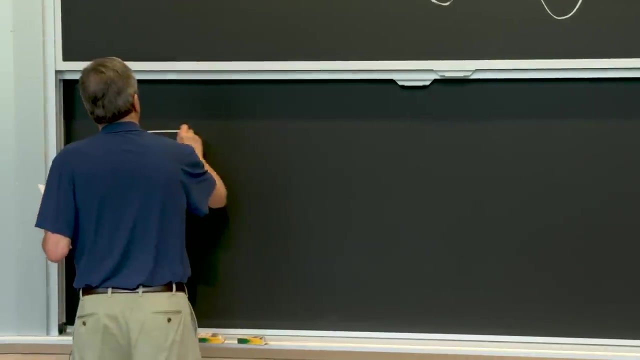 that is a permanent constant And we can do something together. So we're going to look at the emission of the electron. This is the resistance of the particle-like characteristic of light. So for Compton scattering we have a beam of x-rays. 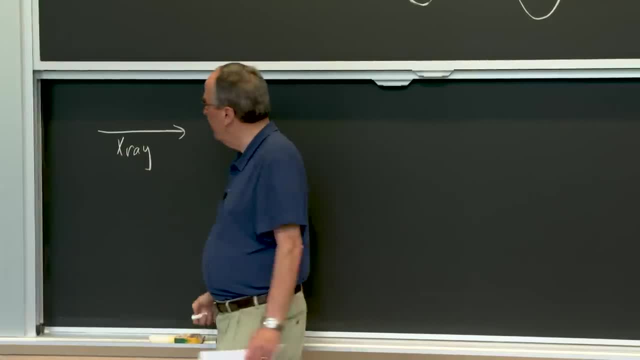 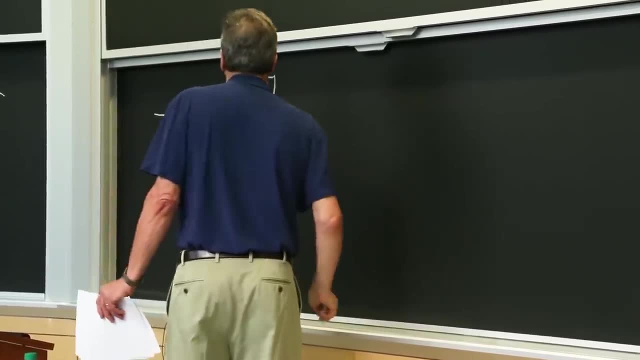 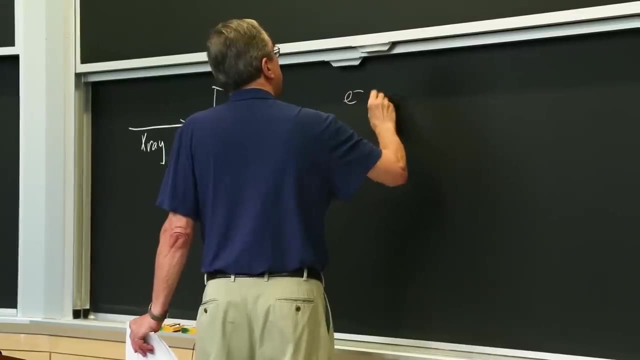 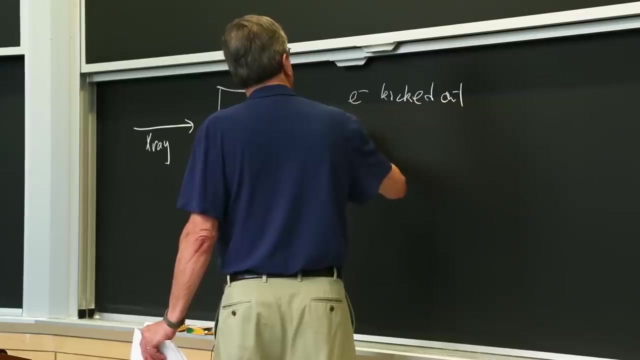 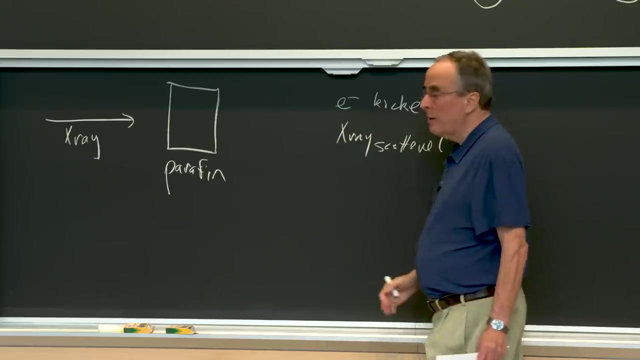 X-ray is a form of light. It's a very high energy form of light. We have a block of paraffin and what we observe is there are electrons kicked out and there is x-ray scattered. So the experiment is: we're looking for the particle. 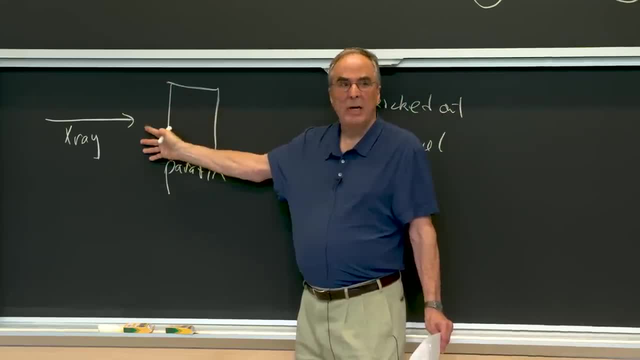 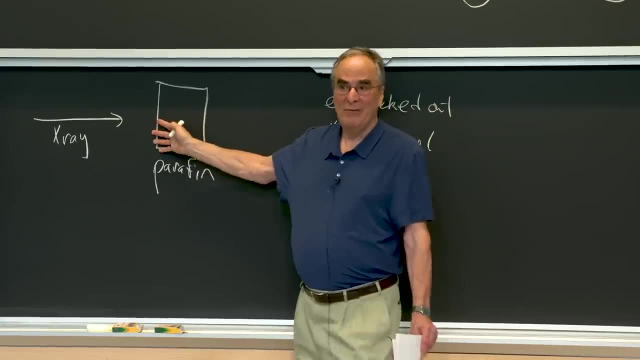 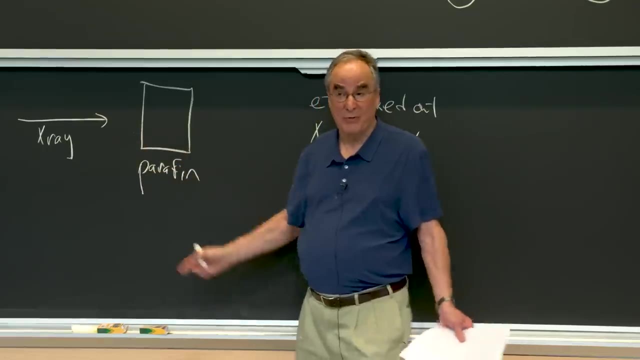 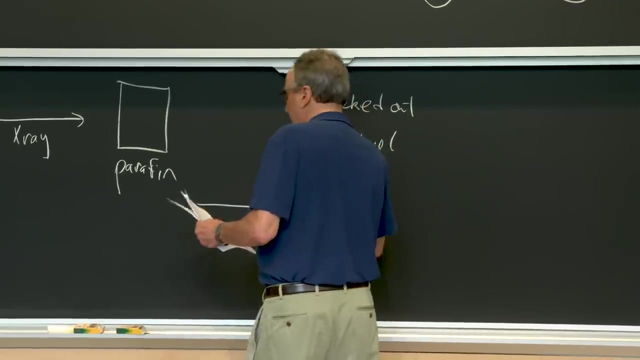 characteristics: Particles have kinetic energy and they have vector momentum And you have been trained painfully and completely in conservation of energy and momentum because it enables you to solve all sorts of useful problems. So suppose the x-ray comes in, hits the block. 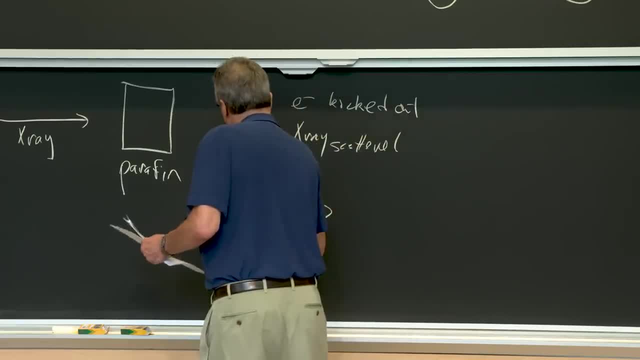 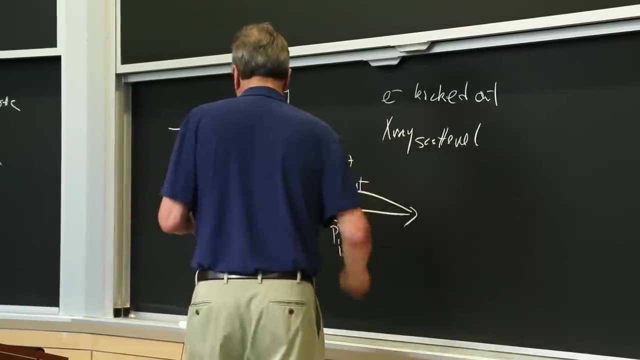 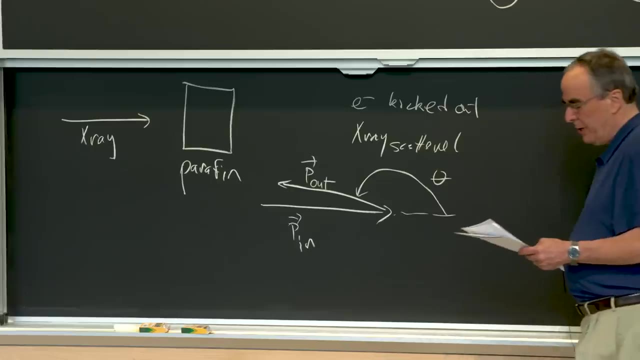 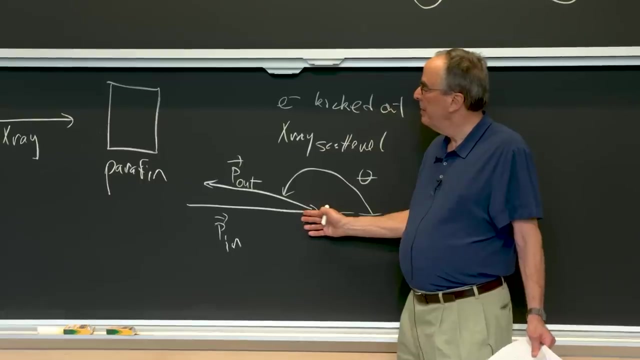 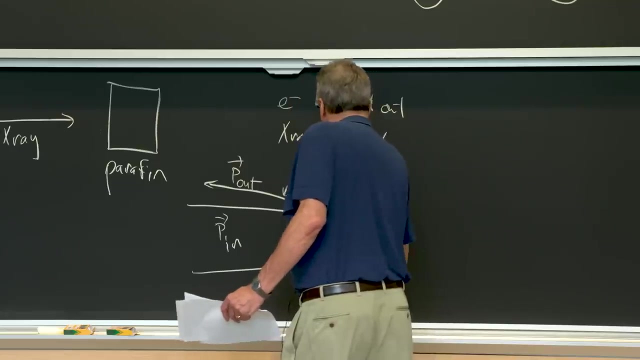 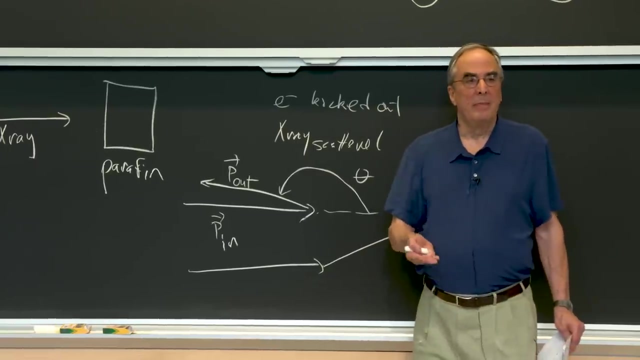 and so we have the incident momentum And the x-ray is backscattered and the scattering angle, theta, is measured this way. So the difference in momentum for this scattering is large for backscattering and much less for forward scattering. So now this momentum has to be transferred to the electron. 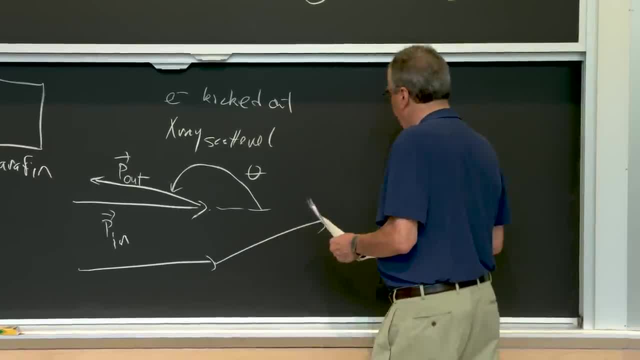 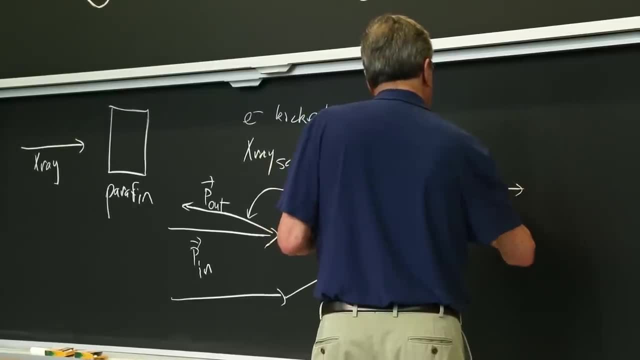 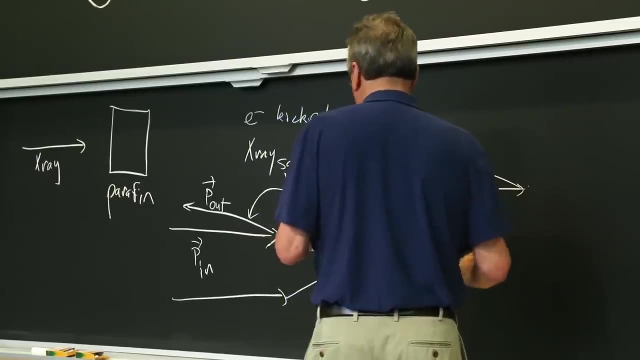 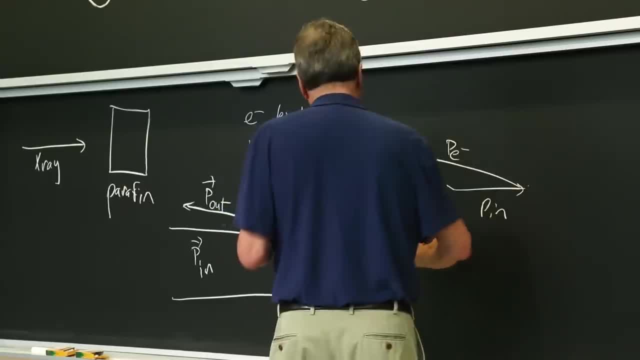 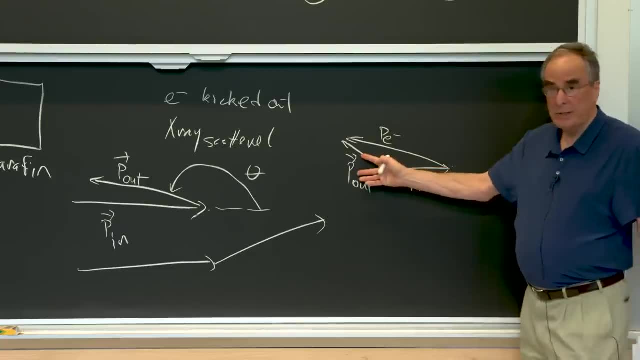 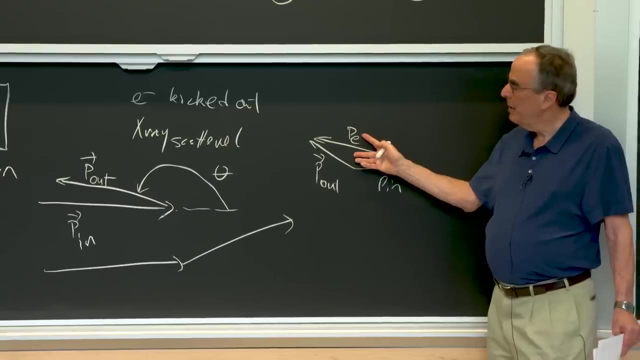 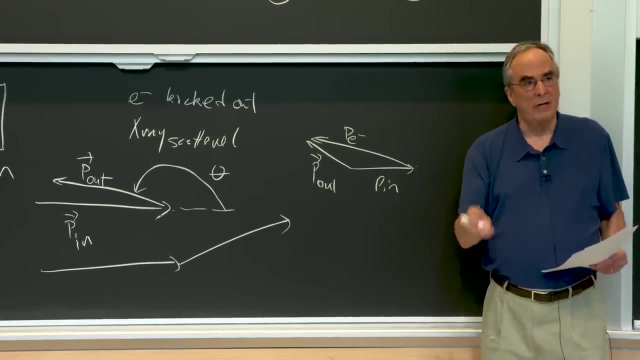 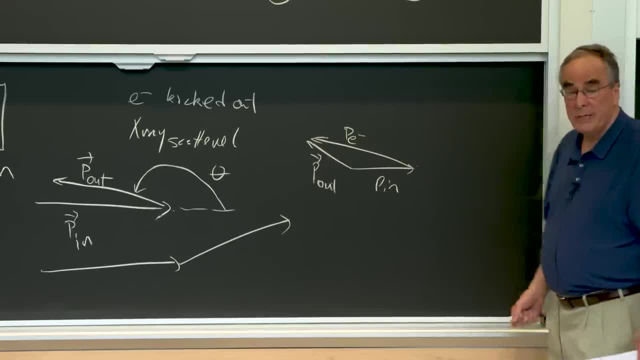 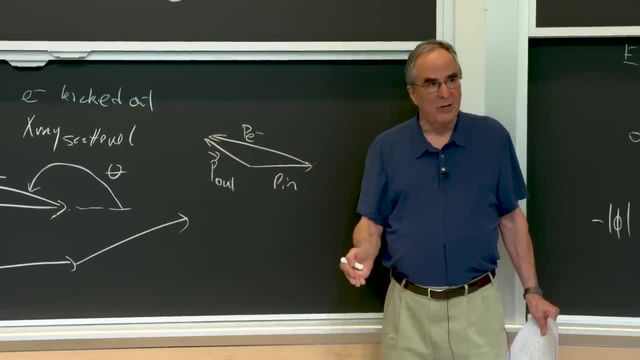 it also transfers energy. So what we're going to see- and I'm just going to wave my hands because the mathematical analysis is something you can do, but I don't want to go through it. I just want to show the structure of the argument. 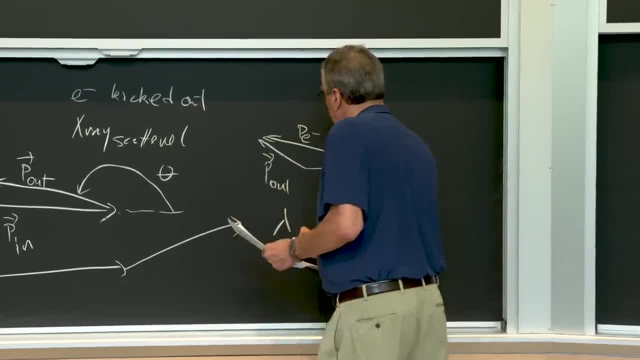 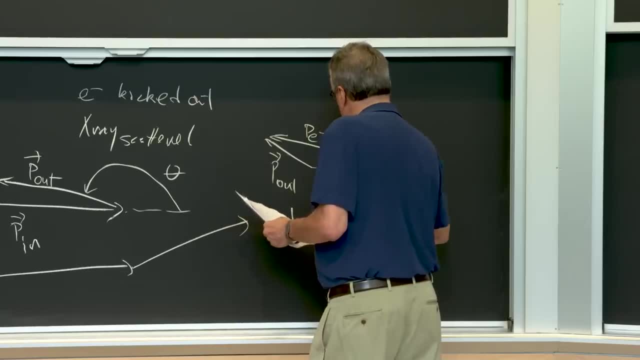 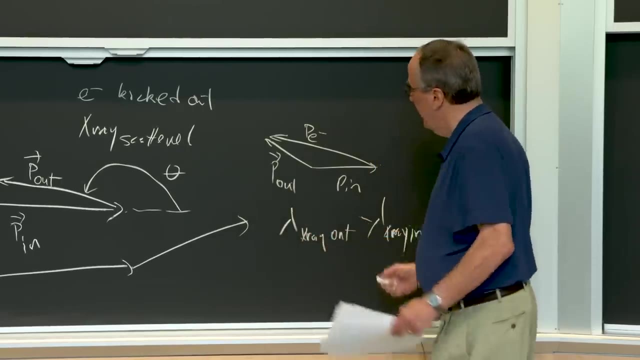 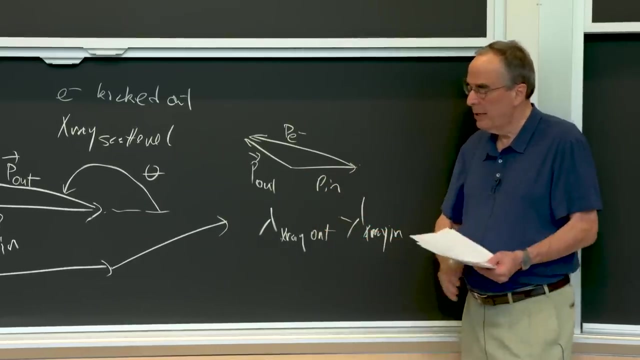 What you measure is the wavelength of the x-ray out, minus the wavelength of the electron. What you measure is the wavelength of the x-ray in, And so if the x-ray has transferred energy to the electron, it has less energy when it leaves. 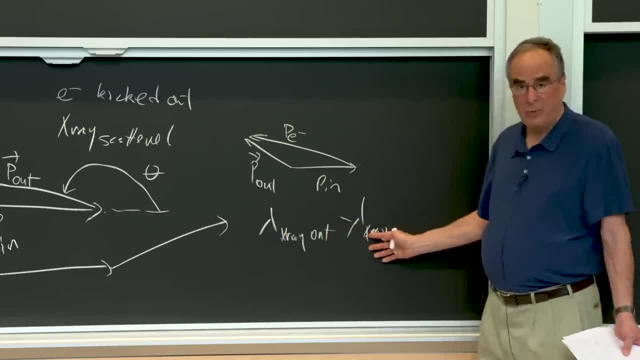 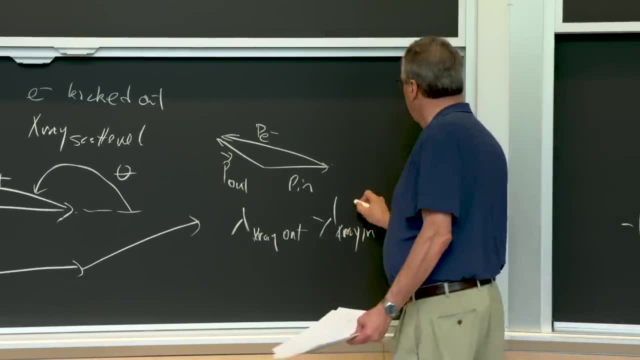 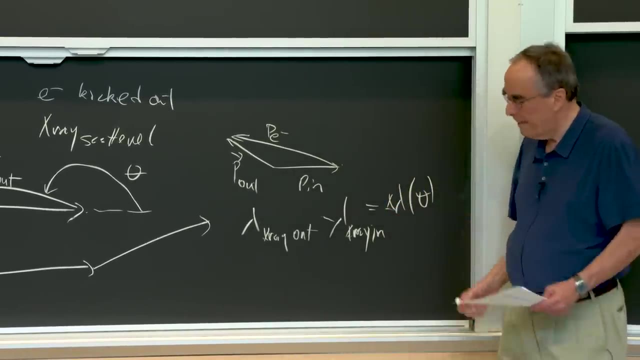 and it has longer wavelength. So this is measurable: the change in the wavelength of the x-ray And that's going to be so we'll call that delta lambda And that's going to be a function of the scattering angle. So Compton scattering basically says OK, particles. 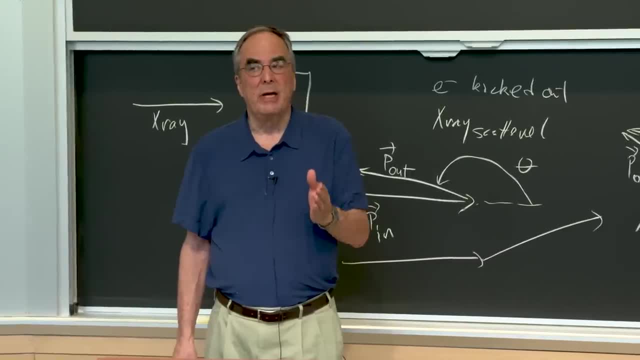 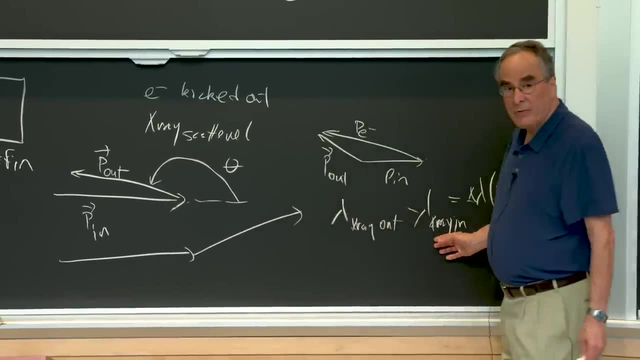 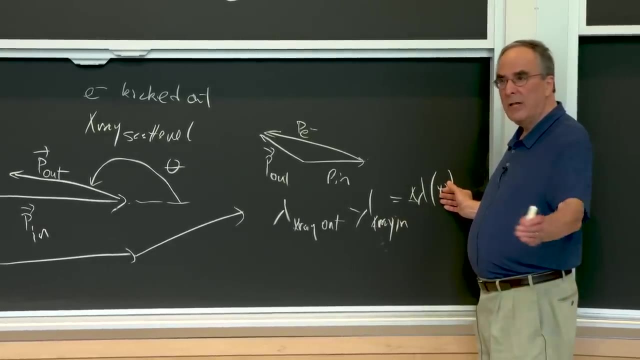 light is a particle. Particles have kinetic energy and momentum. Conservation of energy and momentum predicts a difference, a redshift of the photon, which depends on the scattering angle. The rest is all 801.. You can do that, OK. 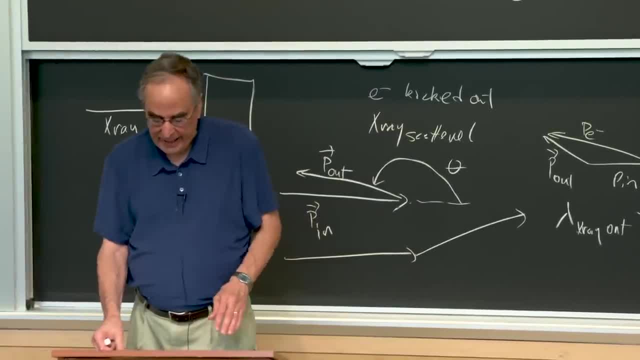 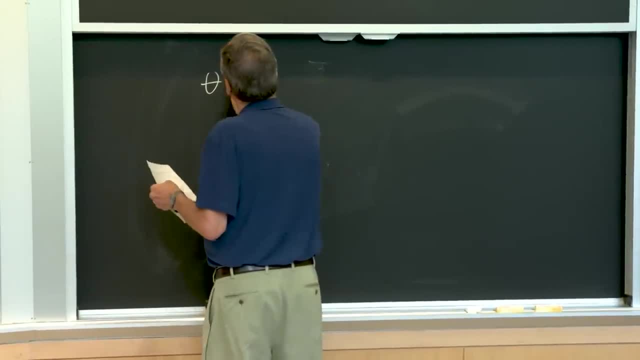 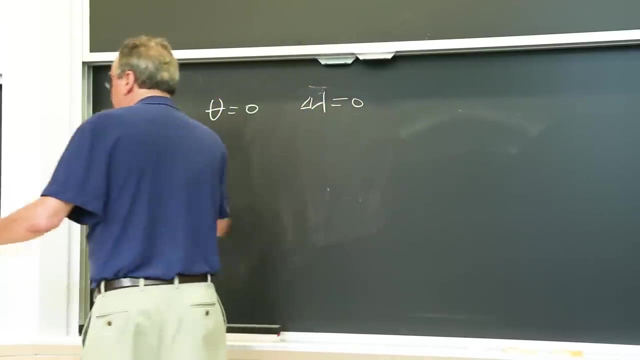 And so what you're going to do is what you end up finding is that if the scattering is 0, then delta lambda is 0. There's no momentum. The photon just goes through If the scattering is pi, in other words, 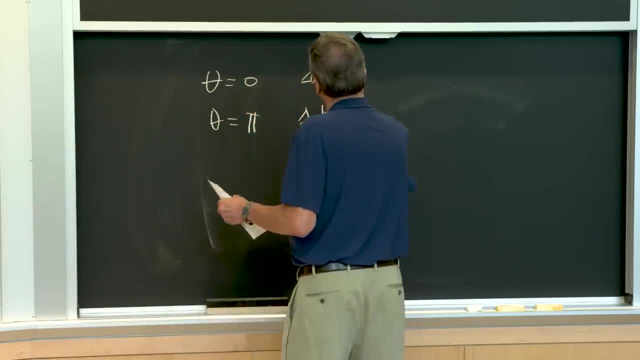 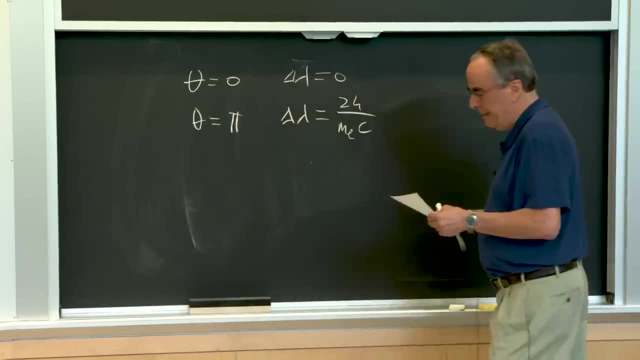 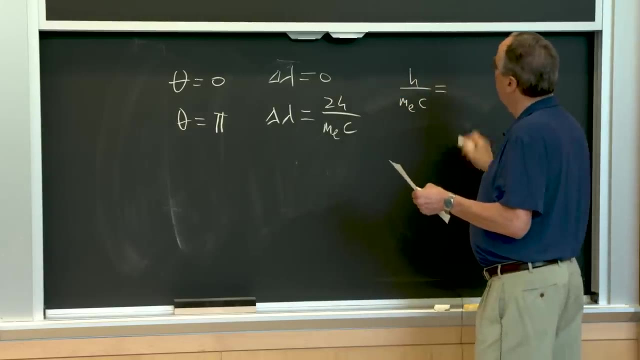 it's perfectly backscattered. then delta lambda you can calculate is 2h over the mass of the electron, The mass of the electron times the speed of light. Now this quantity, h over the mass of the electron times the speed of light, has dimensions of length. 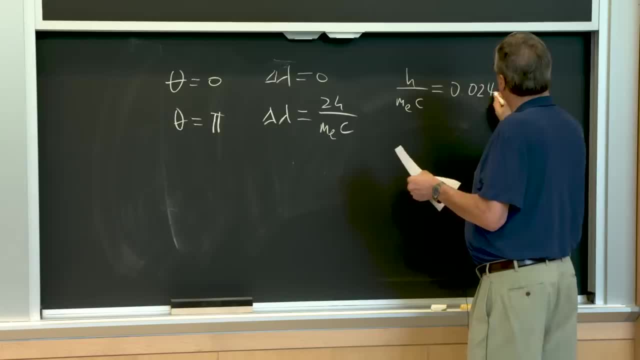 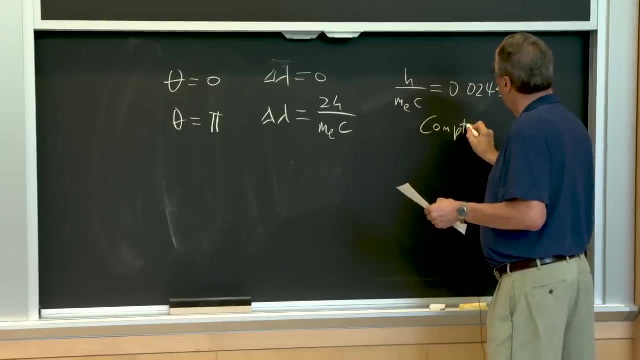 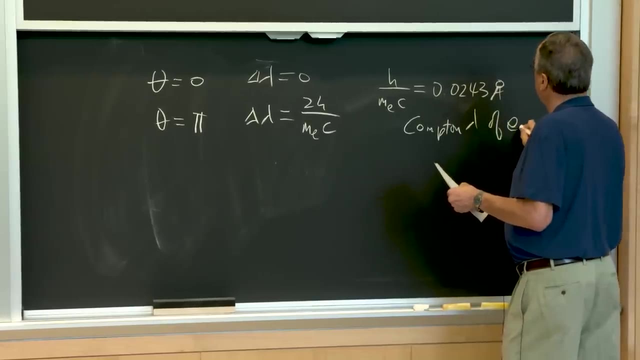 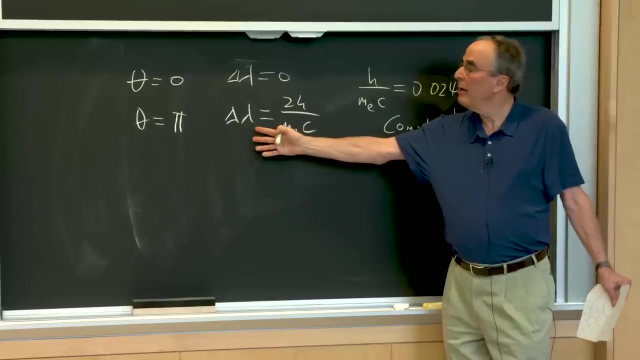 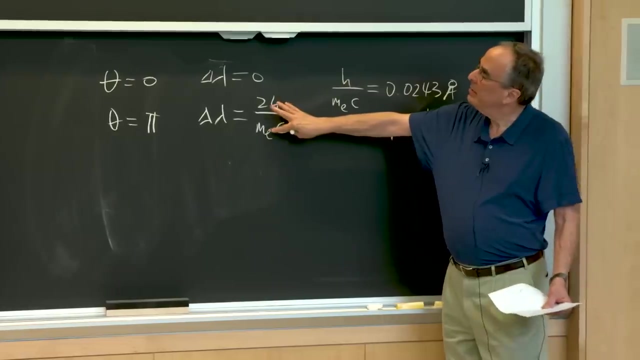 And it's 0.0243 angstroms. And this is called the Compton wavelength of the electron, Because the photon is scattering an electron. the change in wavelength of the photon is determined by this. This is the momentum transfer. This gives you the momentum transfer. 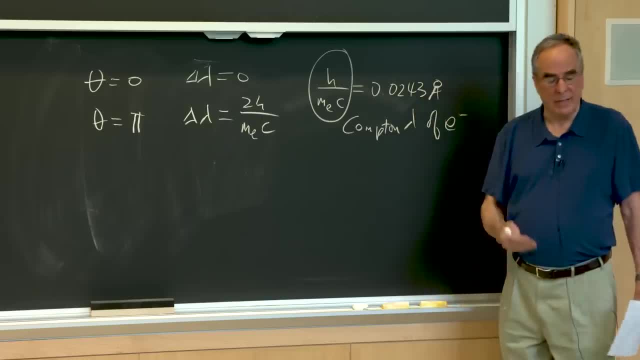 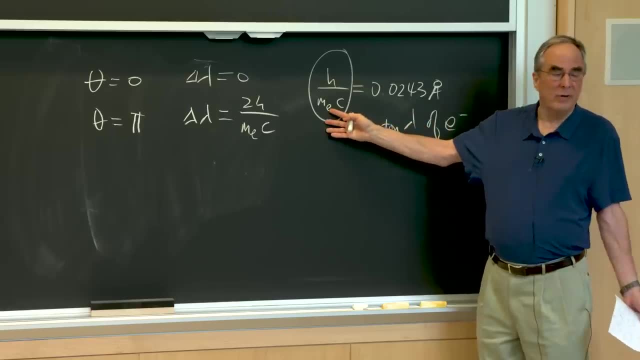 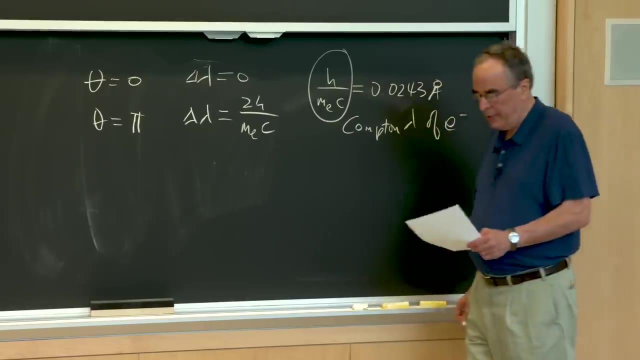 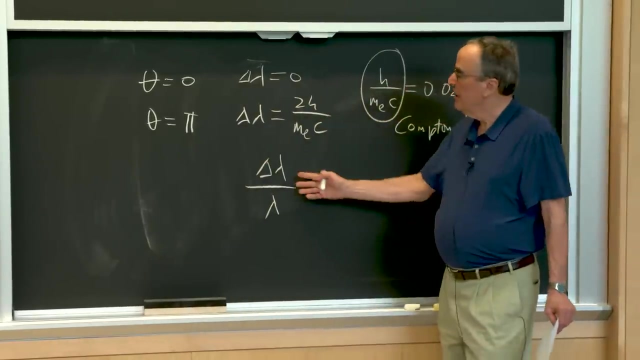 And so this is a universal constant. It says electrons, when they're scattered out of any material, have this behavior. Again, universal and strange. The actual experiment, since what you actually want to measure is the change in lambda over lambda. the change in lambda doesn't depend on lambda. 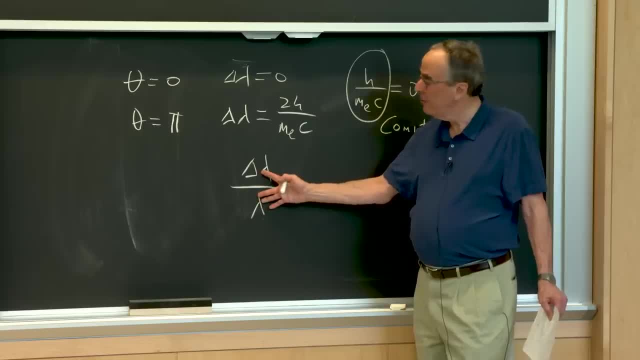 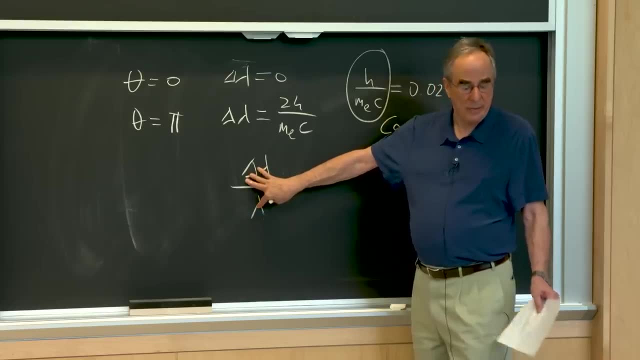 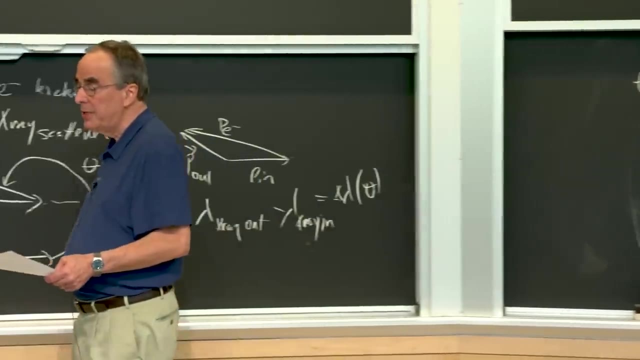 But this does, And so what you want to do is make the observable thing large, And so you go to a short wavelength to make this a large fractional change that's easily measured. OK, The equations are derived in the lecture notes and, better, in text. 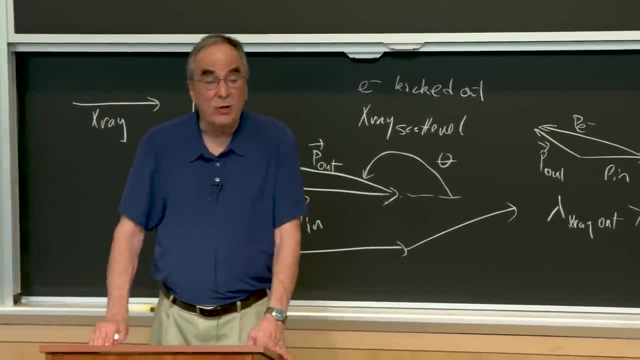 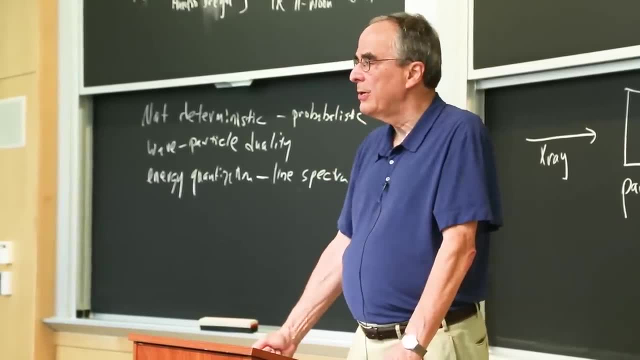 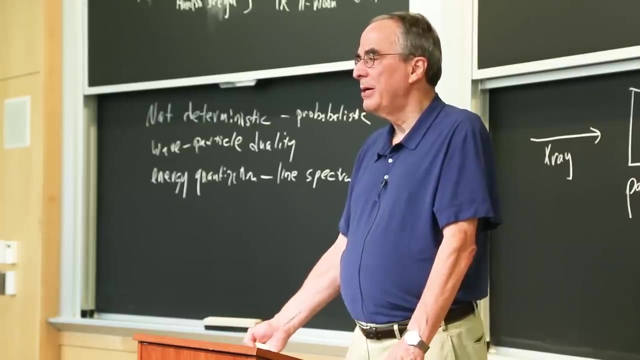 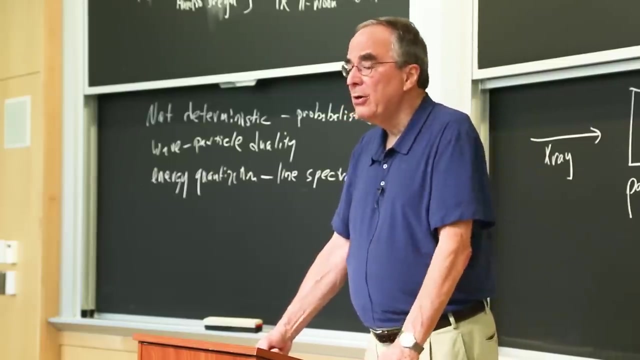 And what I want to do now is just tell you where we're going. We've talked about the wave and particle nature of photons of light, And the particle nature is a surprise, But it's perfectly understandable and observable. The next thing we want to do is determine the wave nature. 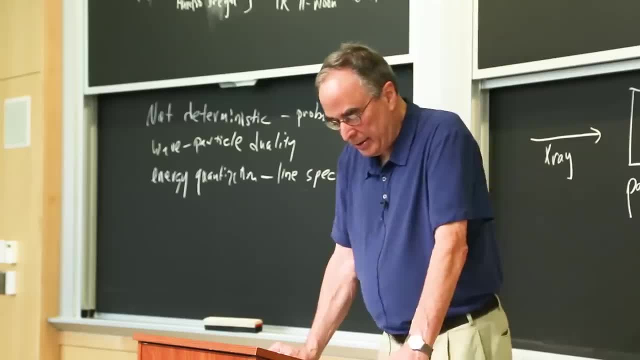 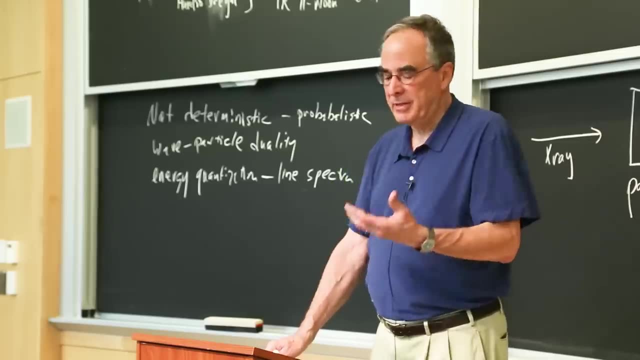 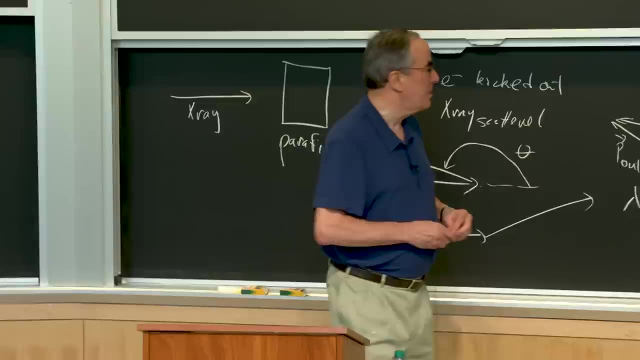 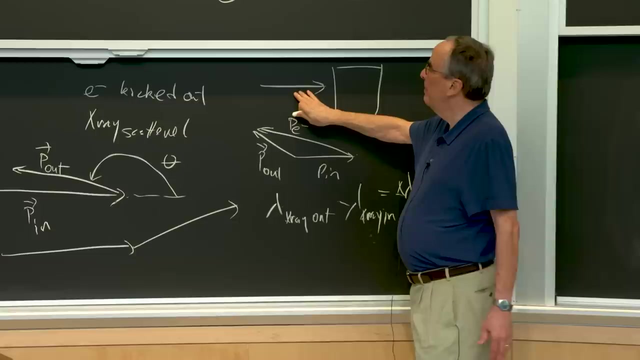 of things that we call particles, And so we're going to do other kinds of simple scattering experiments where we discover that the electrons, So we have some solid And we have- uhh, We have a certain OK- UV light or x-rays- 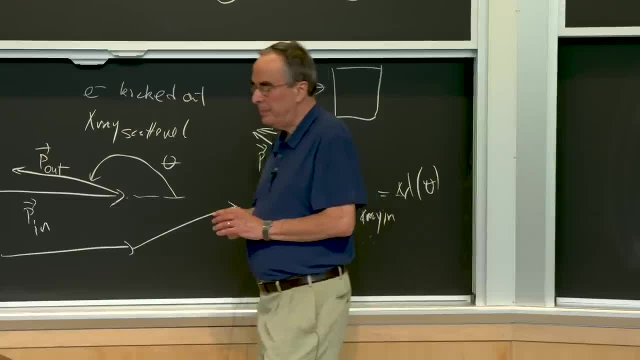 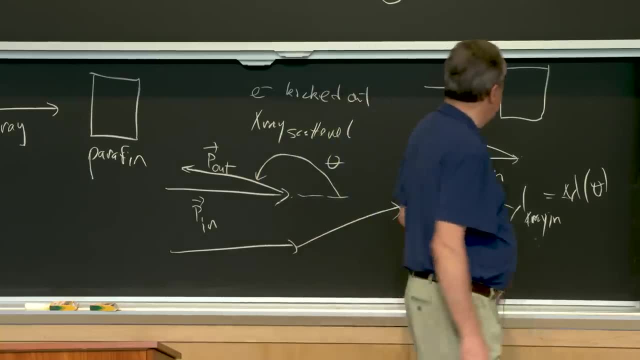 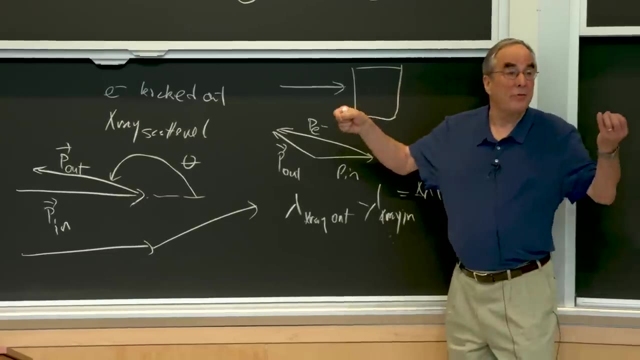 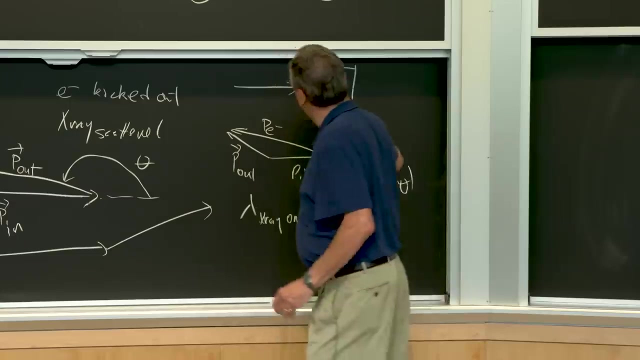 And we go through this solid and it's mostly transparent. It's mostly free space And so this light is interacting with the electrons and maybe with the other stuff that is involved in matter, the nuclei, But the important thing is that the electrons, that 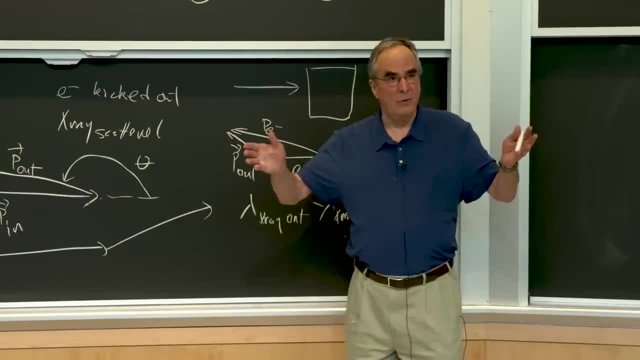 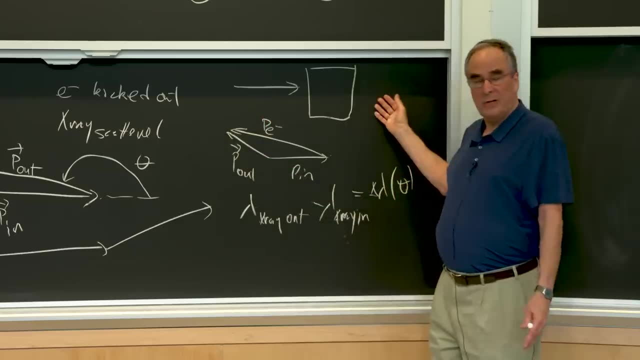 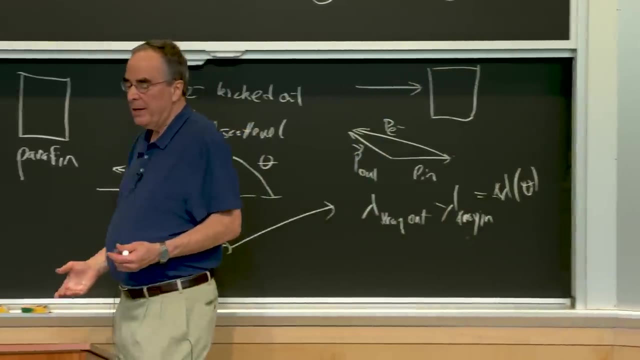 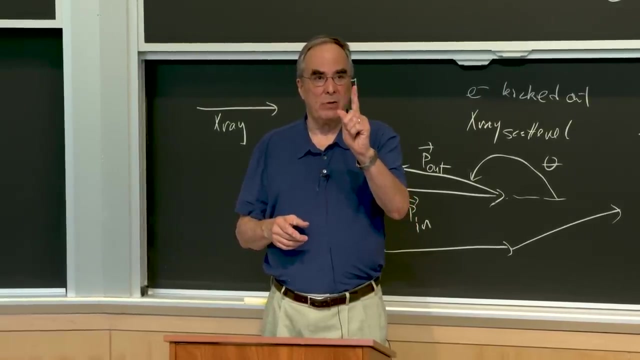 get scattered, are in a kind of a diffuse state. This is mostly nothing. This material doesn't scatter x-rays. It's mostly transparent, And so an explanation for that is the Rutherford Planetary Model, where we have a nucleus- It's a nucleus with a charge and electrons orbiting that nucleus. 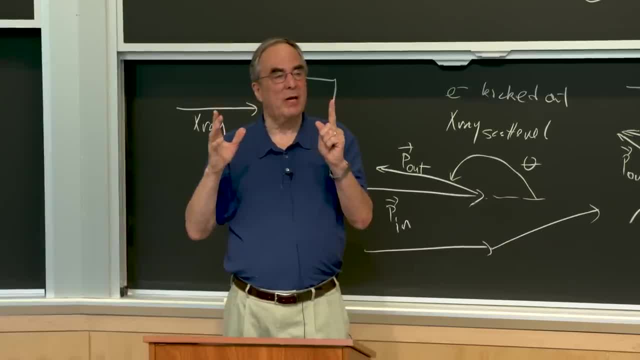 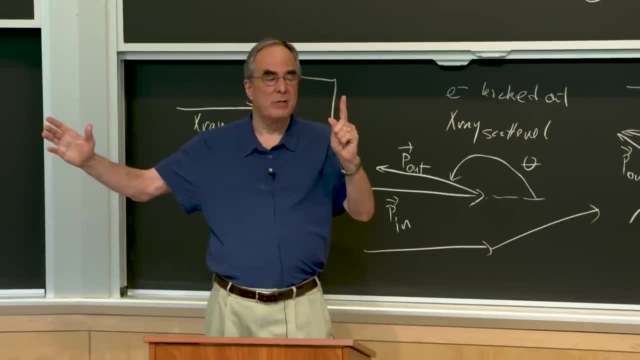 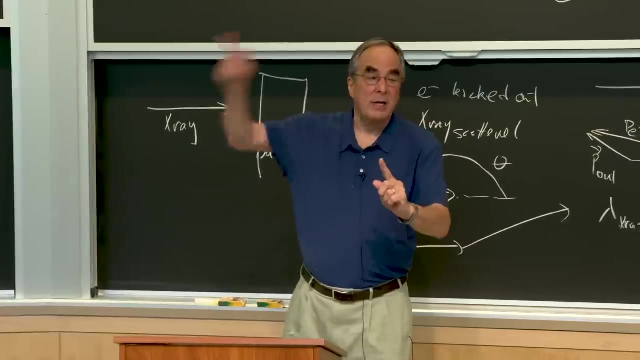 And that's all very nice. It's a way of saying: well, OK, the electrons are forced to choose distances from the nucleus and there's mostly empty space. But then you look more closely and the electrons are doing this, They're oscillating in space and they're 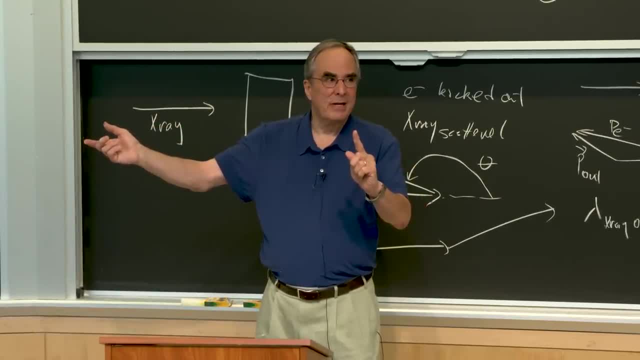 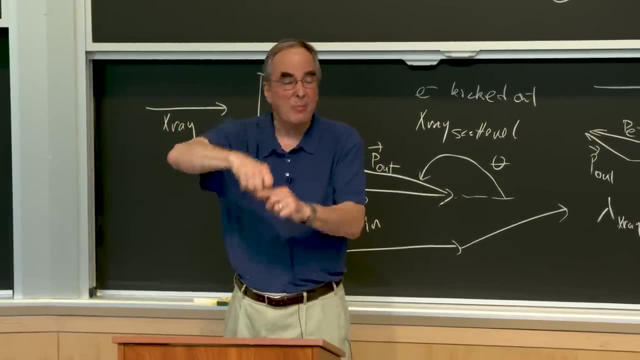 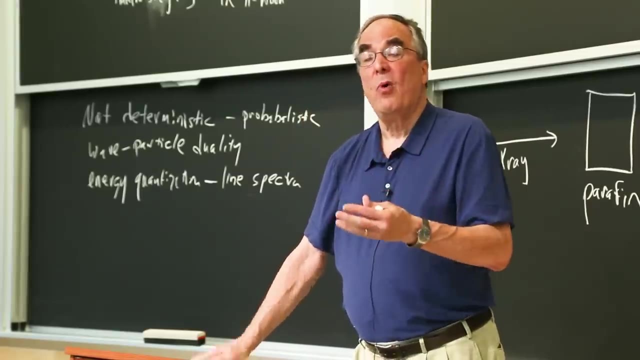 going to radiate energy, And this is really important. This radiation of energy will cause the electron to spiral in and combine with the charge in the middle, and that's a problem, And so we have an explanation for why matter is mostly empty space. 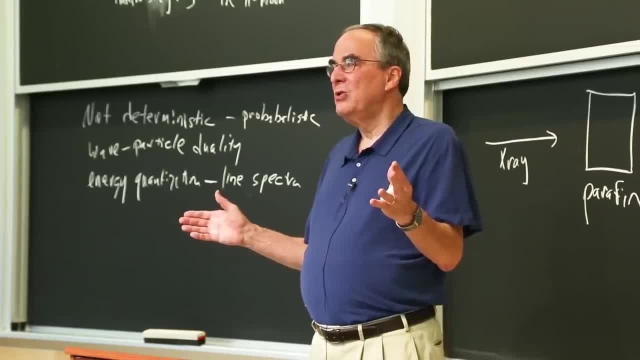 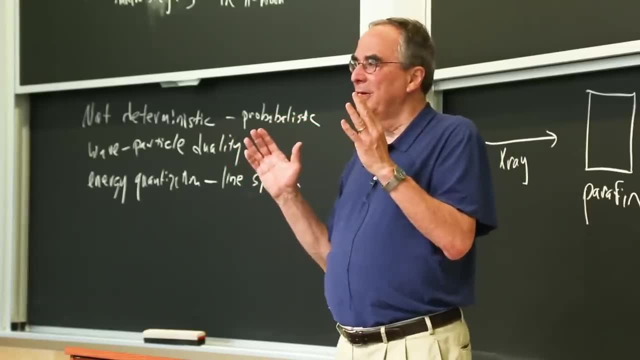 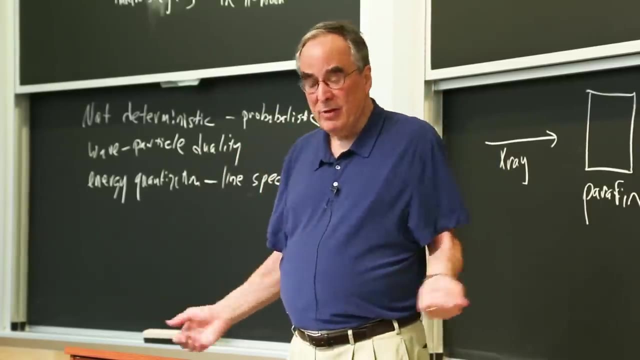 And a conundrum: the electron should recombine with the nucleus. So how can matter be relatively non-compressible if it's not in the nucleus? And the best explanation is this planetary idea. But then we have this thing. we have to explain. 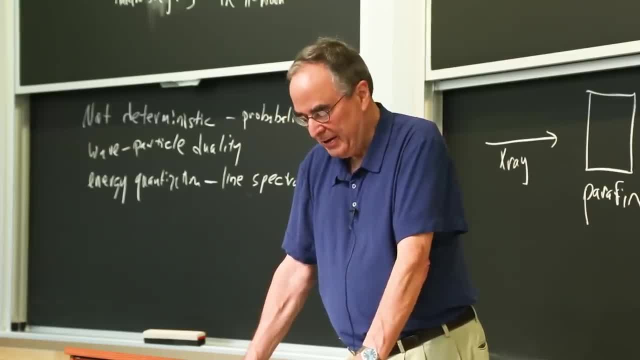 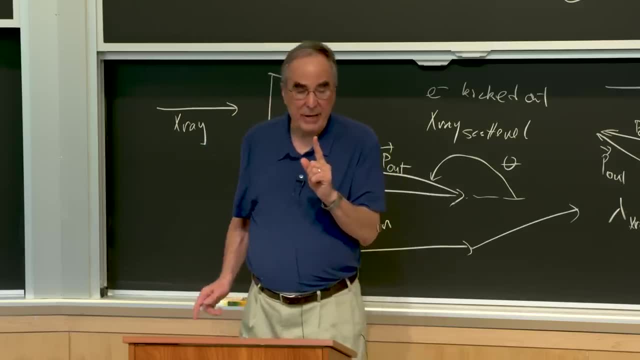 Now there's two hypotheses for this, which are really just ad hoc things. One is the Bohr model, where it says: in order for the electron to obey some laws of physics, as it orbits the nucleus, the nucleus, it conserves angular momentum. 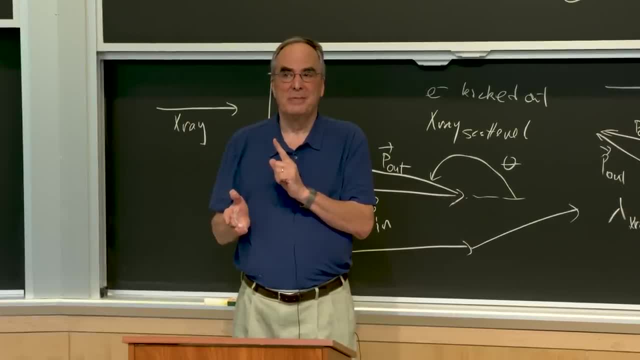 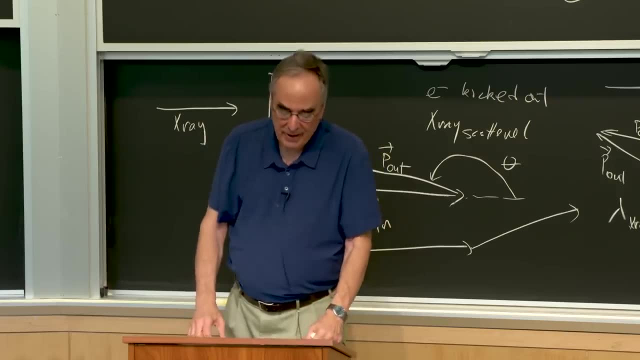 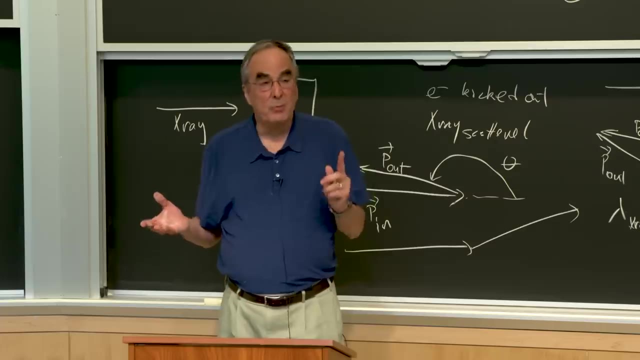 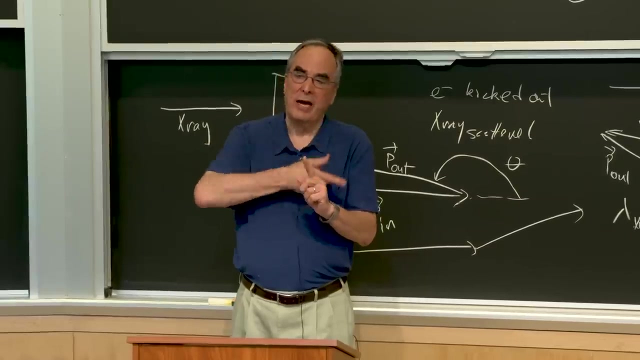 Well, if it were rotating into combined with the nucleus, it wouldn't do that, And so that's sort of OK. And then there's de Broglie, who's a very smart person, was a very smart person, And he said that in order for the electron. 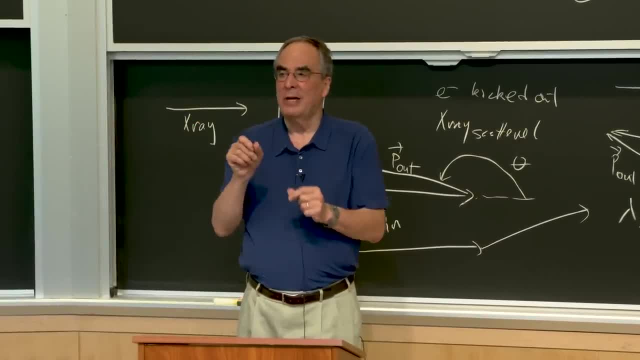 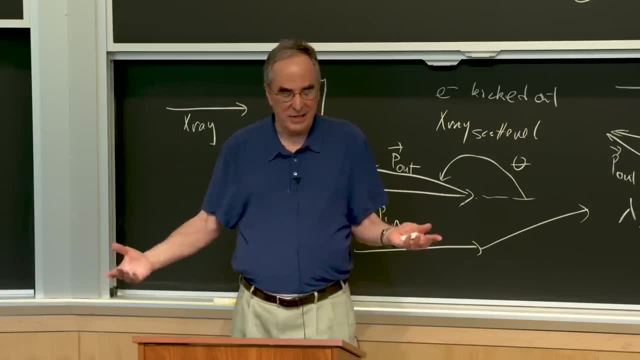 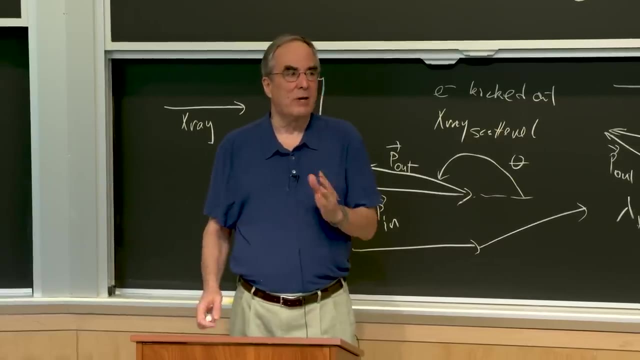 not to annihilate itself as it goes around the orbit, it has to have an integer number of half wavelengths along that trajectory. Then it will annihilate itself, And that is much better than Bohr's hypothesis. But both of these hypotheses lead to line spectra hydrogen. 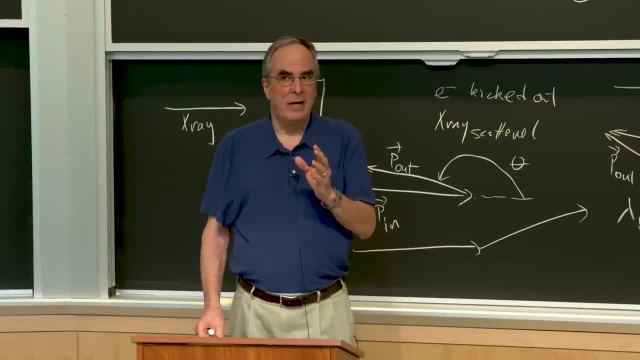 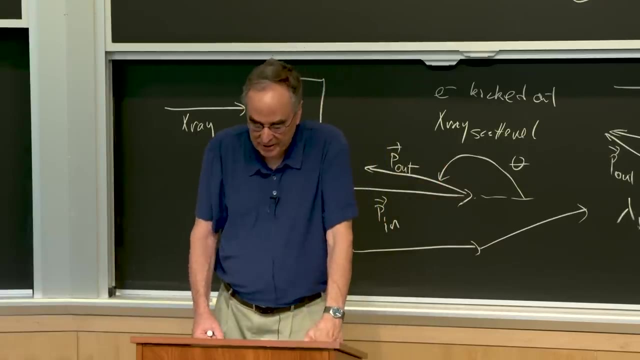 where you can build a really simple model and you can predict to eight decimal places all the absorption transitions of hydrogen atom. So a very simple model leads to an incredibly, incredibly good analysis. It's an incredibly powerful and mysterious result. There's another experiment that I will talk about next lecture. 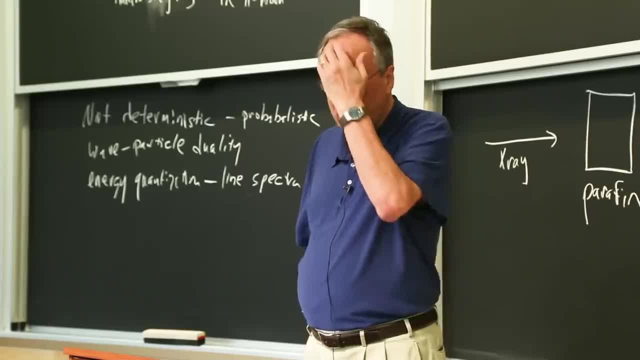 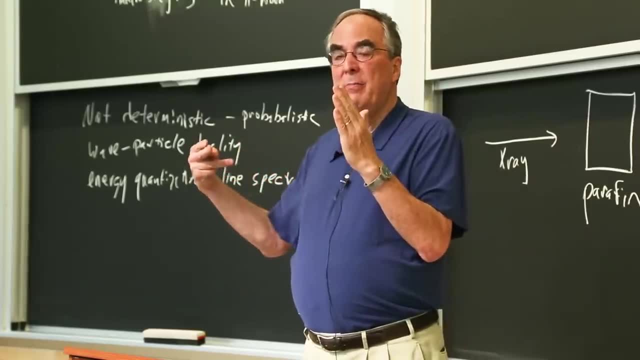 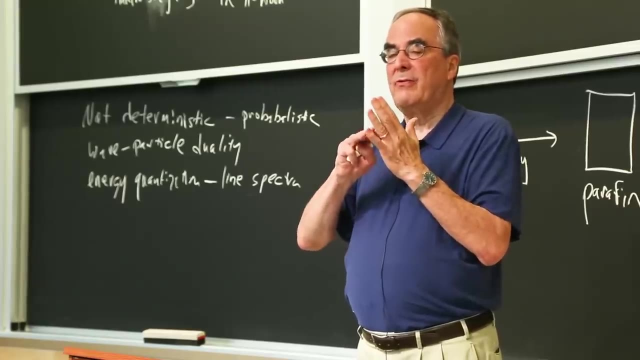 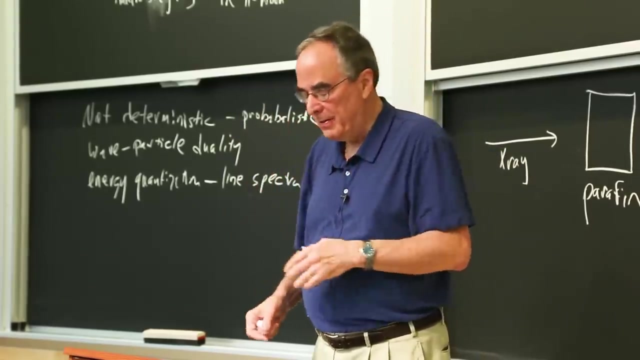 And that is suppose. we have a thin sheet of metal, We have photons, x-rays or UV photons impinging on this metal And what it's? the there's diffraction, regular distances between atoms in the particle, in the foil. 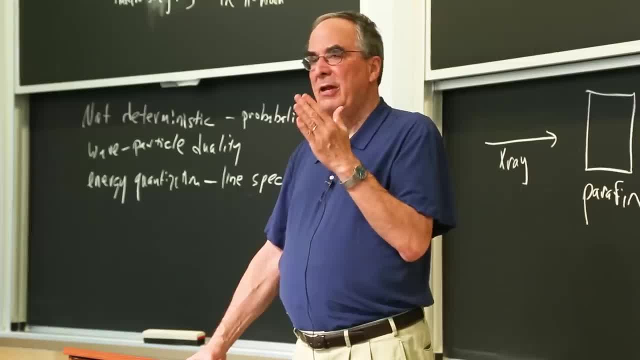 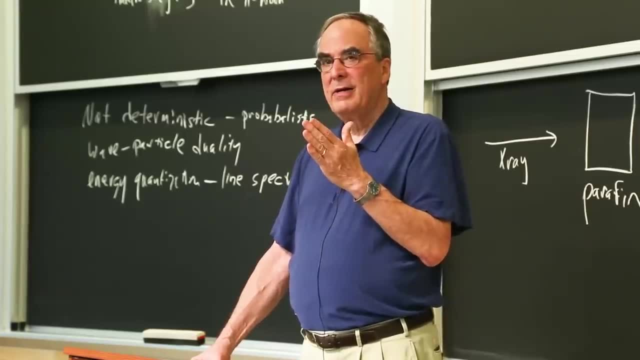 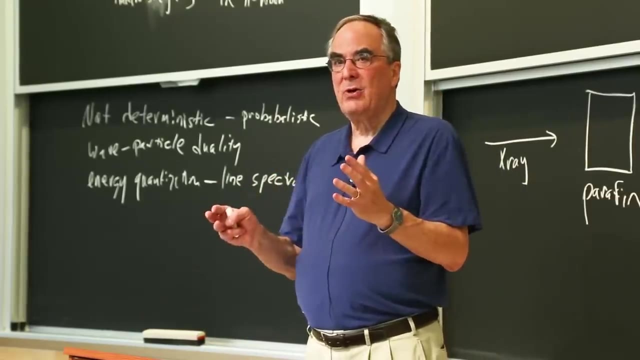 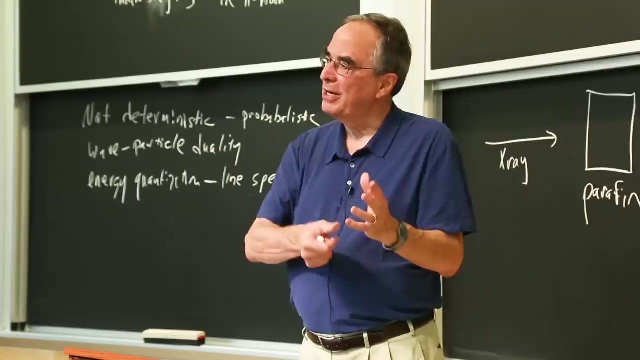 And so what we measure is diffraction rings for the electron and for the photon, And the diffraction rings are identical when you choose the wavelength of the particle to be equal to the wavelength of the photon, And so this is another way of showing wave-particle duality. 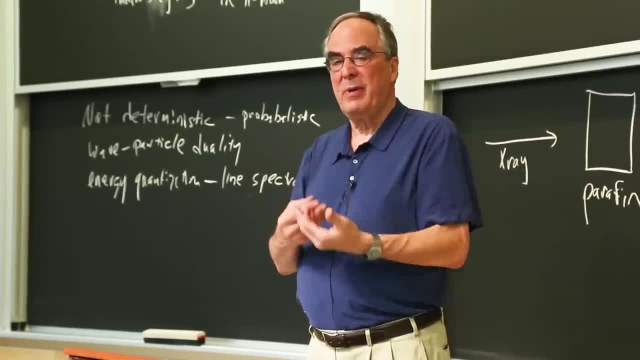 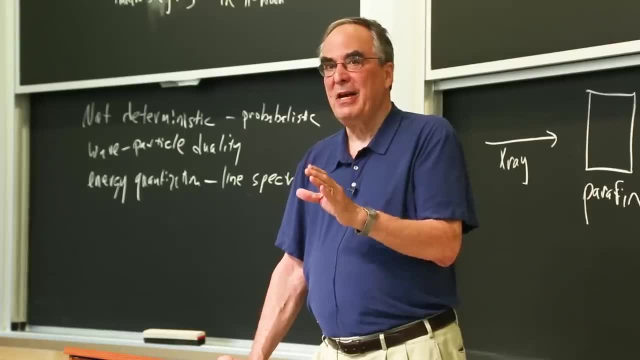 We can show that they have wavelengths and we can calculate to make them the same. So this is all very exciting, And this is about as much philosophy and history as you're going to get from me We're going to once we understand.